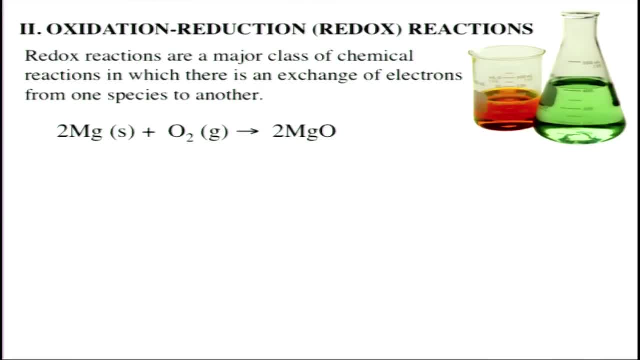 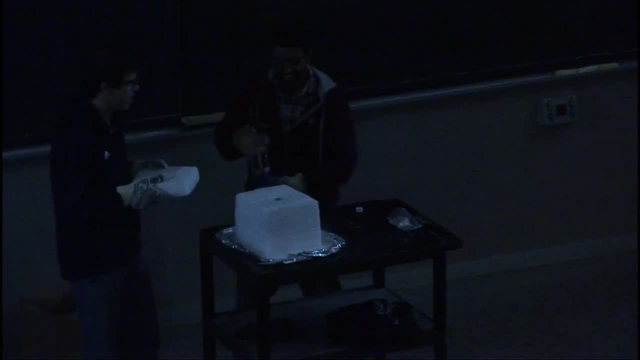 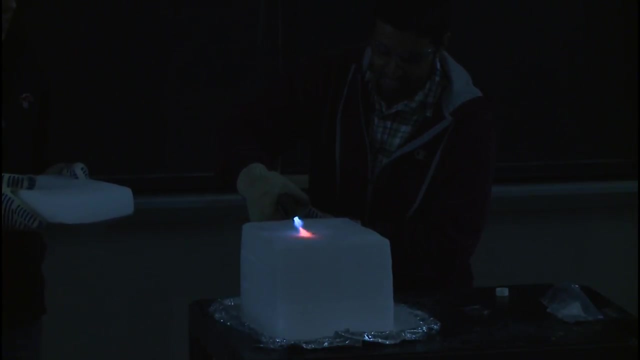 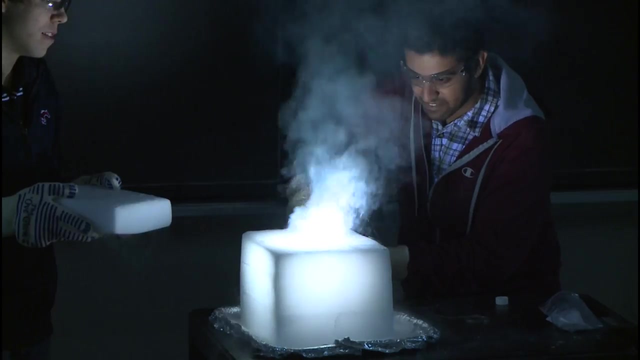 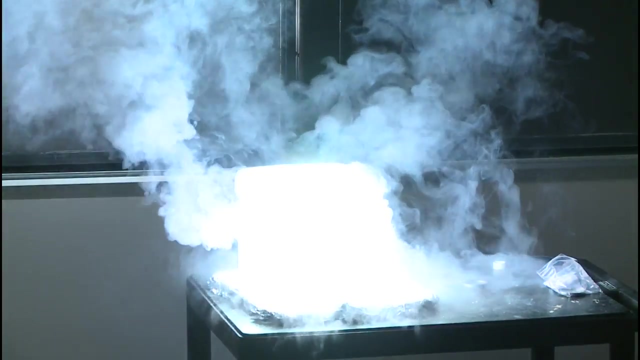 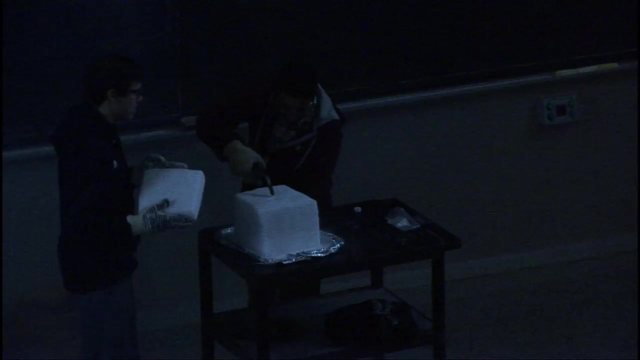 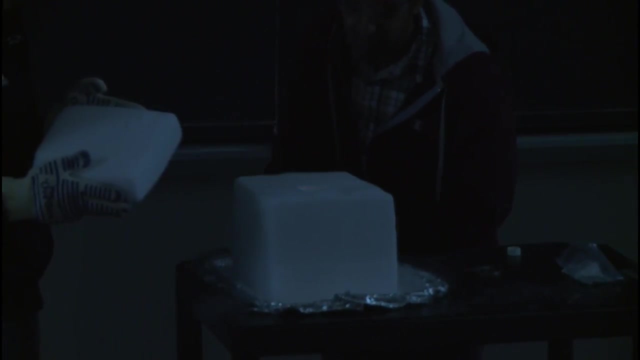 That makes it a whole lot more fun. Hi, Which was two again. Two was the smiley, the resonance one. And three was the exciting one was very exciting. I'm going to try it one more time. OK, All right. 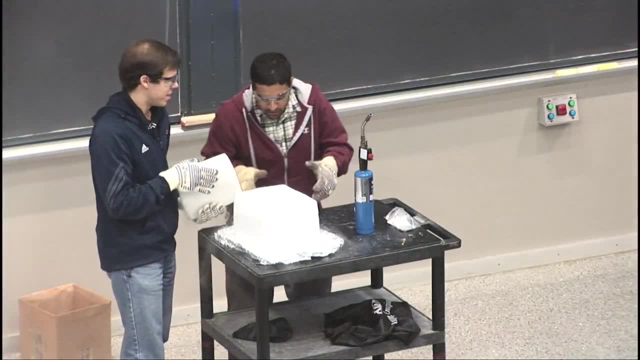 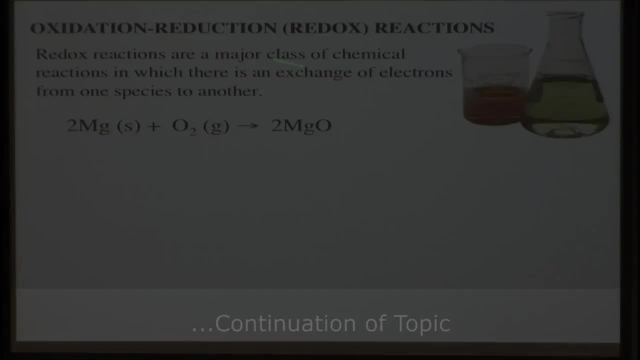 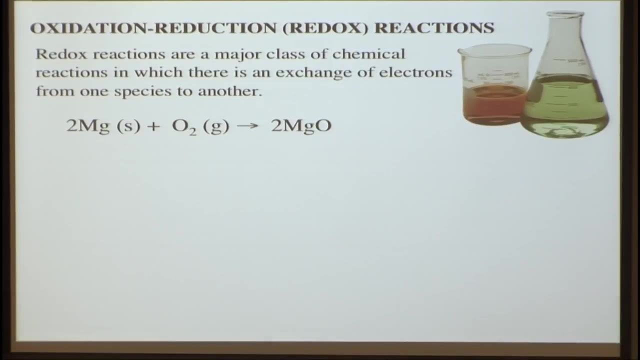 OK, Good try. So oxidation reductions are really fun, And so we're going to continue and tell you about those on Friday. So Oxidation reduction or redox. So redox is the shorthand for oxidation reduction. Let's bring out your hands, but let's bring the noise level. 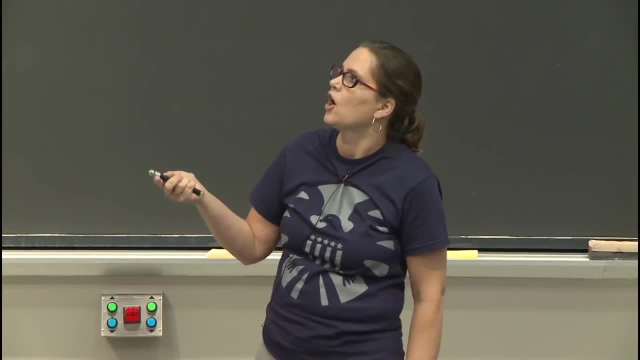 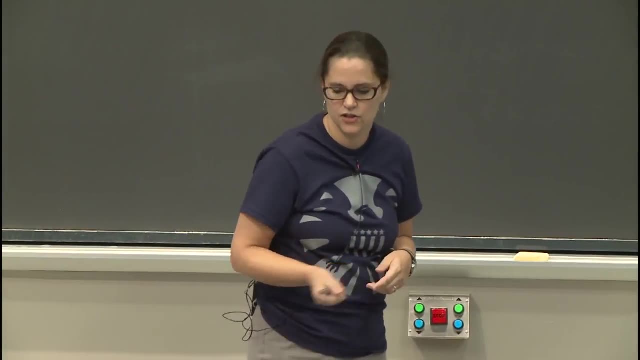 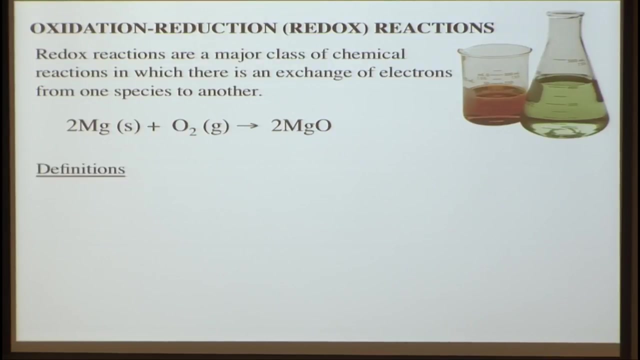 down. People have still been complaining about the noise in class. All right, So a redox reaction, chemical reaction that involves an exchange of electrons, And so we saw what happens when we mix this with some dry ice. All right, So let's do some definitions. 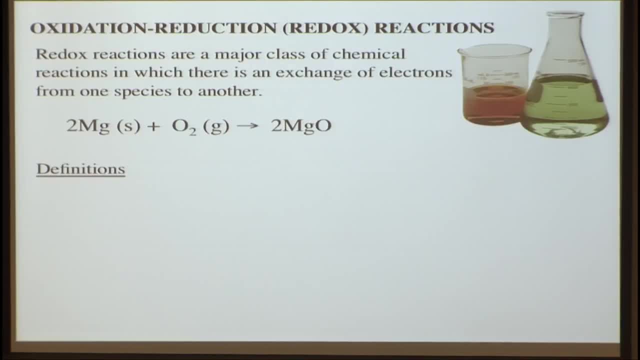 We always start units with definitions And most of you know some of these definitions already: Oxidation, electron loss Reduction. electrons are gained. This one, you may or may not be familiar with: Oxidizing agent: It accepts electrons. 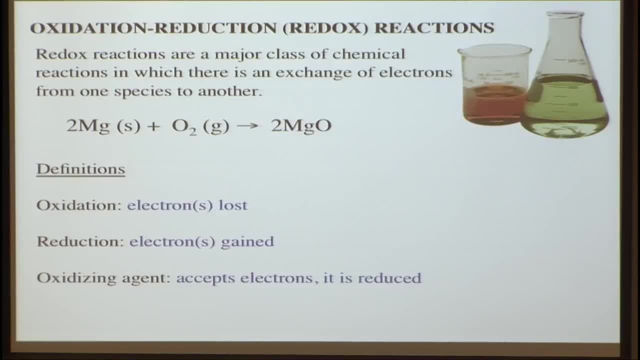 So it oxidizes other things, But it itself is reduced. And reducing agent donates electrons. It reduces other things, It itself is oxidized, And before you turn the page, I just want to try to get you to remember these two terms. 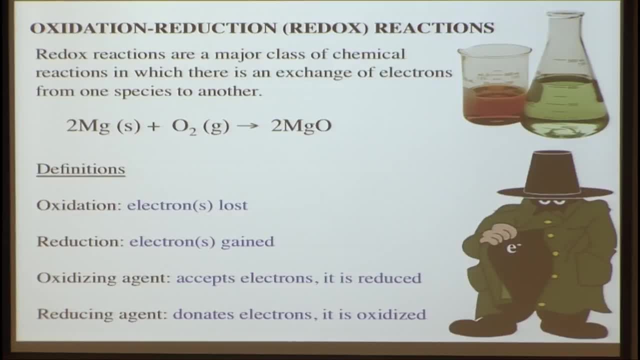 So one way that I like to think about it is that a reducing agent might be somebody who is a little bit shady. They might walk up to someone and say: in a crowded space, don't look at me, just listen. Do you want to buy an electron? 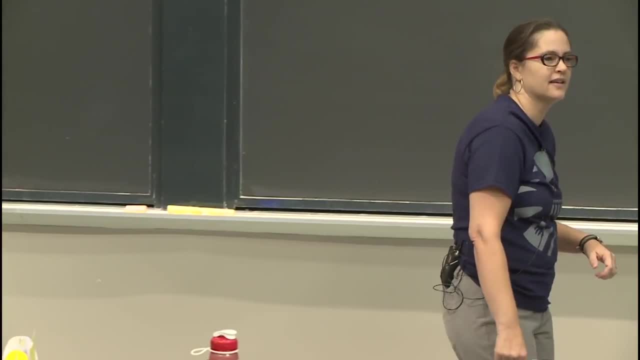 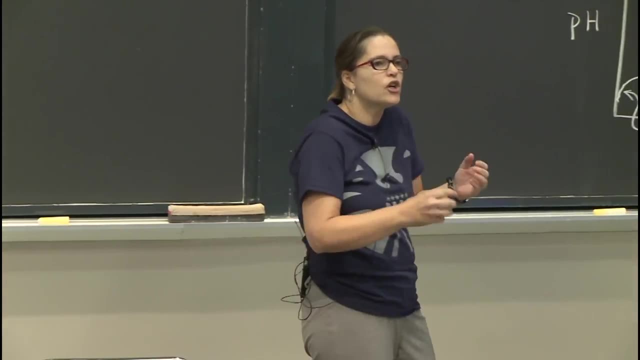 So that would be an agent of reduction. going around Now there could be ones that are a little bit shady, selling electrons to the highest bidder, But there could also be agents of good. I told you about free radical species. There's a lot of free radicals in the universe. 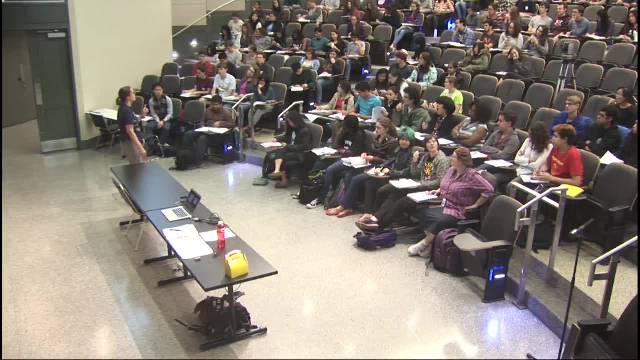 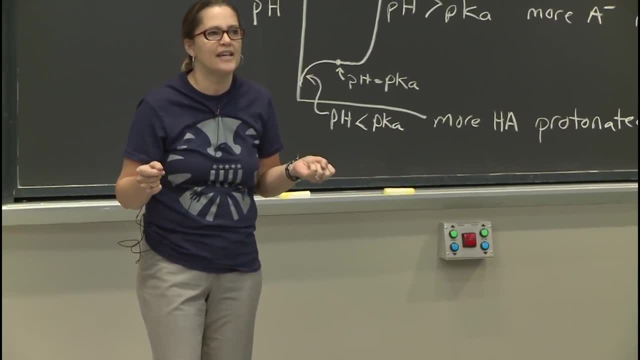 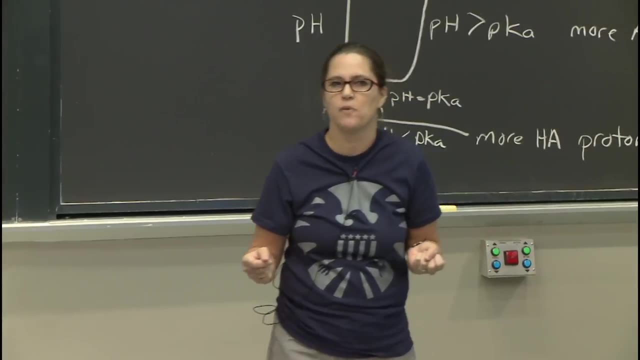 They can be dangerous because they have a single unpaired electron which makes them really highly reactive. So there might be an agent, a secret agent of oxidation, And it might want to shield the universe from the power of free radicals, And so it would go along and it would oxidize that. 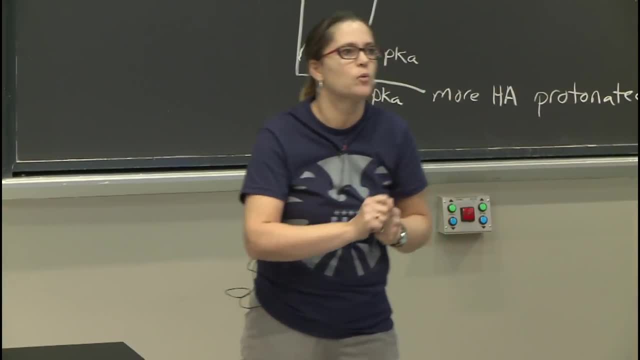 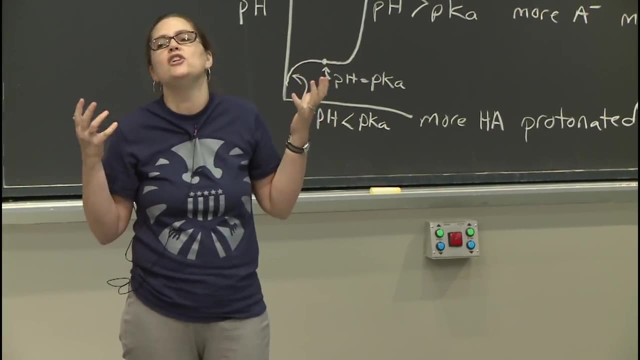 give it. take that electron away and oxidize it and become reduced itself. Take that free radical away, Because the free radical species might not know how dangerous it is. It's for everybody's good to shield you from that power. You might also have an agent. 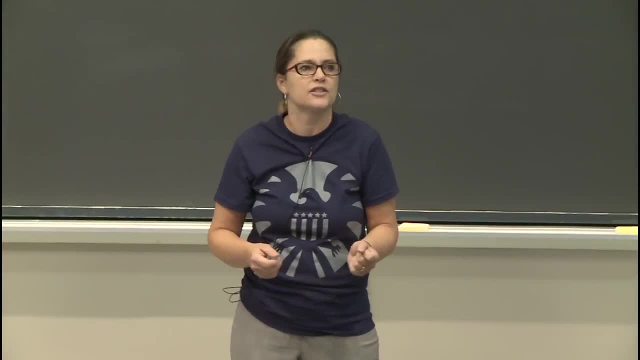 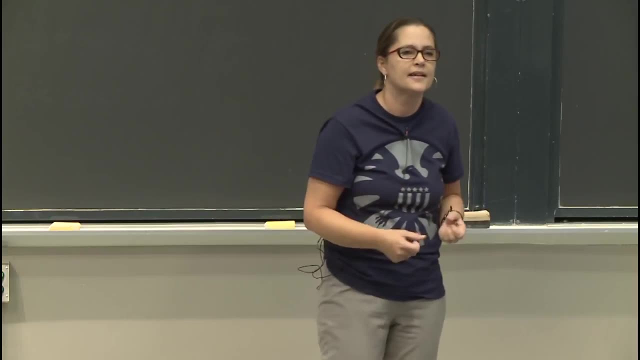 of reduction. that's a secret agent that might go up to the free radical species and give it an extra electron, and then it has two, and then it's more stable and less reactive. So you might have these agents. So that's how you should think about it. 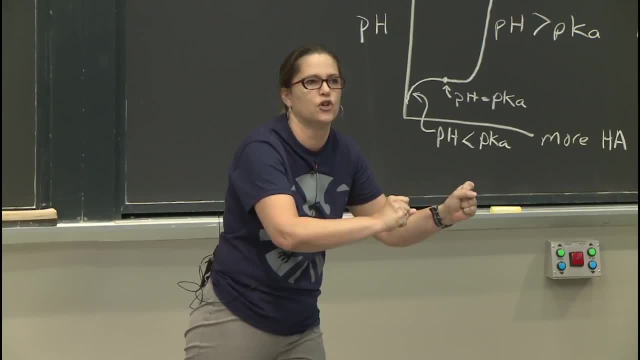 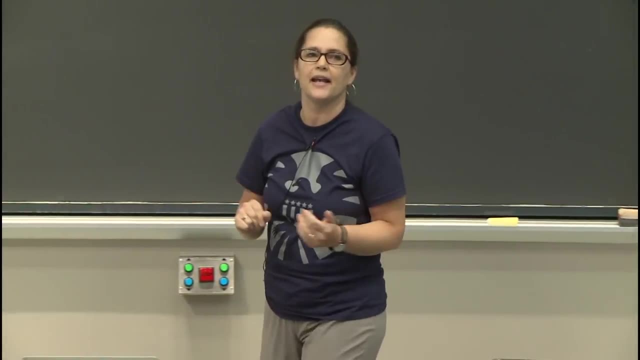 Think about an agent of oxidation that wants to go out and oxidize for the good of mankind, Or an agent of reduction that wants to go out and reduce other things. So that might help you remember those definitions. We'll hope so. All right, so let's take a look now. 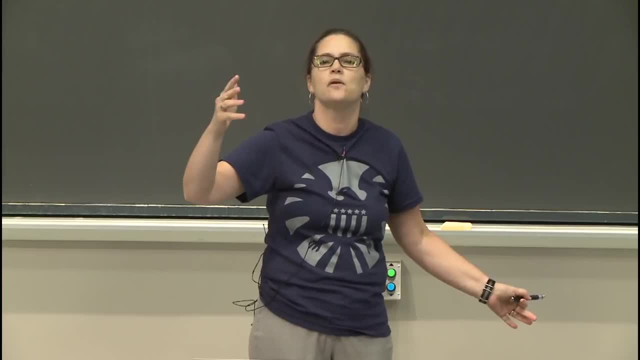 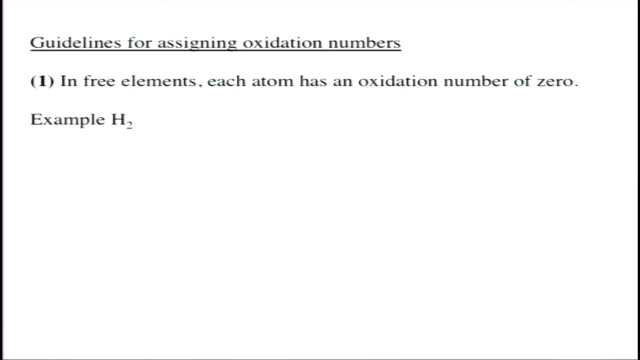 We always start every unit with definitions, and then we have a set of rules and guidelines. So let's take a look at the guidelines. Luckily, these guidelines are really pretty straightforward, and you really shouldn't have a lot of difficulty keeping them in mind. 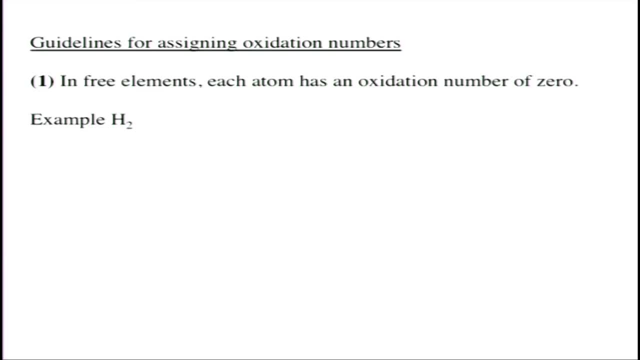 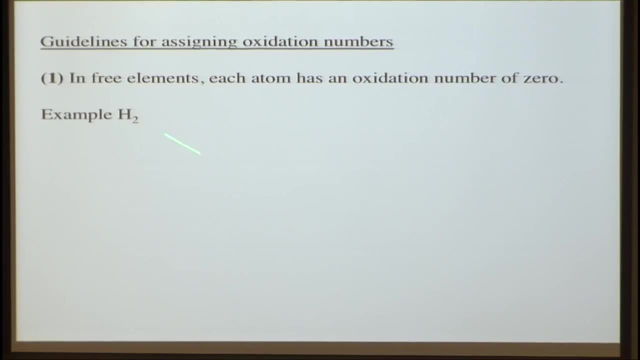 Some of them we've really seen already. We just didn't realize that they were going to be the guidelines that we would have. So guidelines for assigning oxidation numbers In a free element. every atom has an oxidation number of zero. Okay, that seems pretty straightforward. 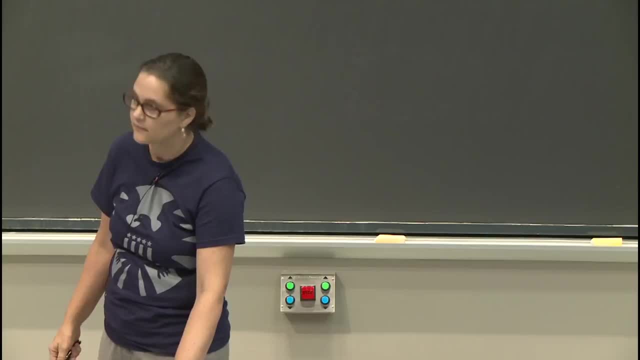 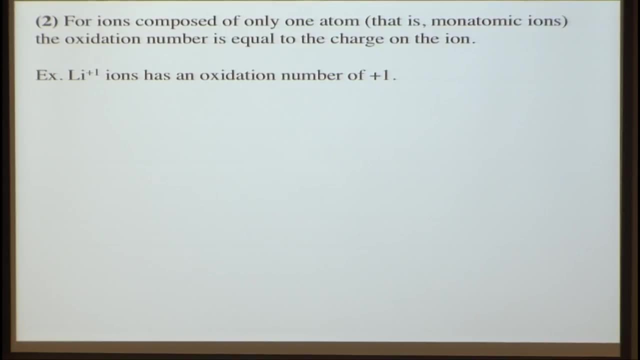 H2, oxidation number zero. Rule two Ions composed of only one atom, also called monatomic ions, have an oxidation number that's equal to their charge. If this wasn't true, it would be deeply disturbing Lithium plus one ions has an oxidation number of plus one. 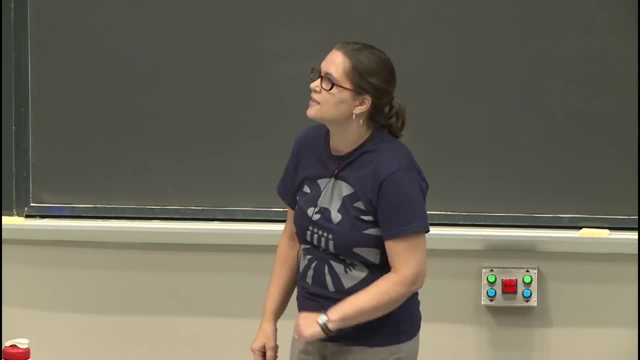 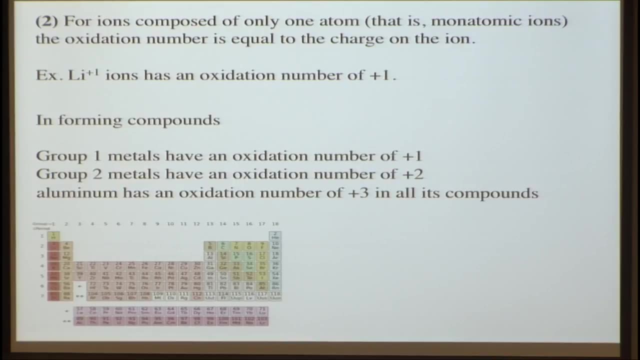 I think we're good. Okay, also in number two, in forming compounds, group one metals have an oxidation number of plus one: Lithium and all of its friends, sodium, et cetera. Group two metals have an oxidation number of plus two. 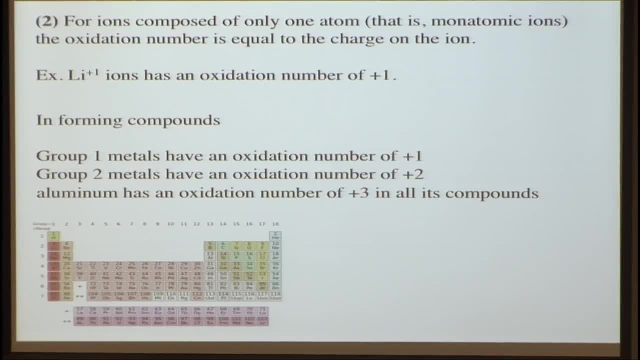 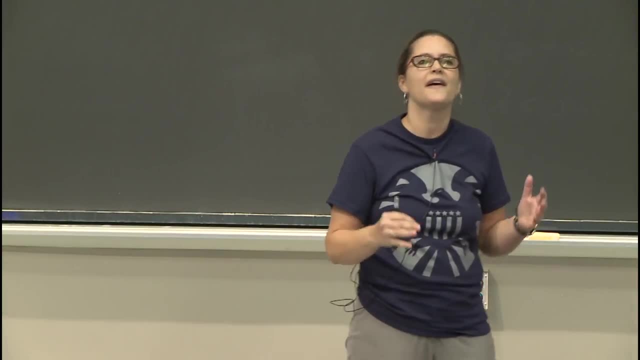 Calcium, for example, And aluminum is plus three in its compounds. This is also something that we've seen before. Those group one and group two metals are not all that exciting. They pretty much want to get their noble gas configuration and they want to lose either one if you're in group one. 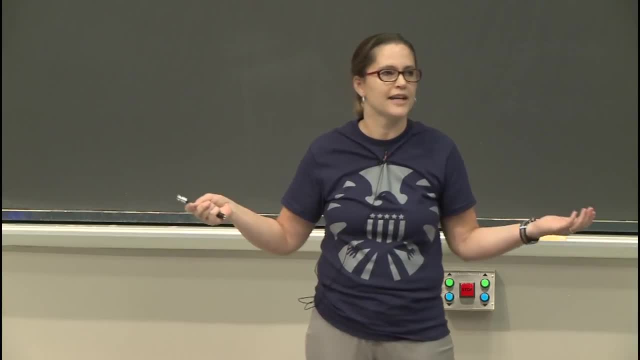 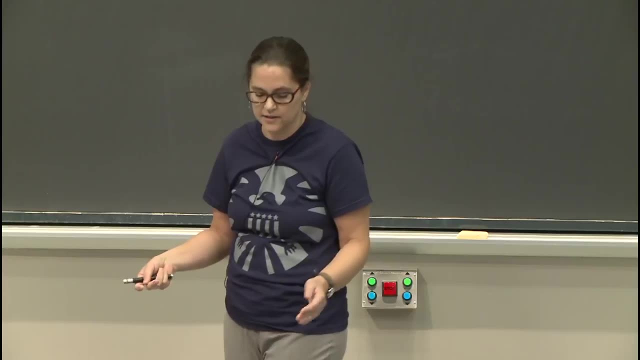 or two electrons if you're in group two, And so that's what they do here. So this is good to keep in mind because it's going to help you figure out the oxidation number of other elements for which there are not such hard and fast rules. 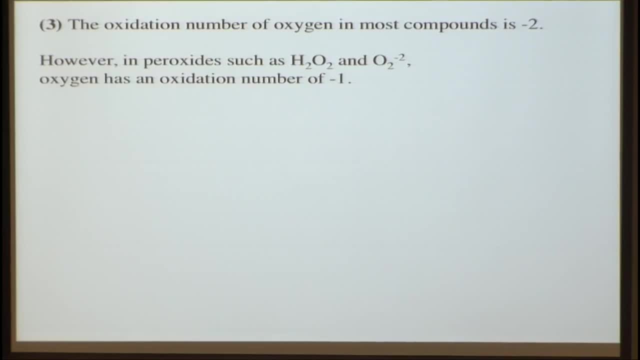 Number three: oxygen. Oxygen in most compounds is minus two. Again, not that surprising That it would want to gain those two electrons. However, there's some exceptions. Oxygen is just an element full of exceptions If it is in peroxides. 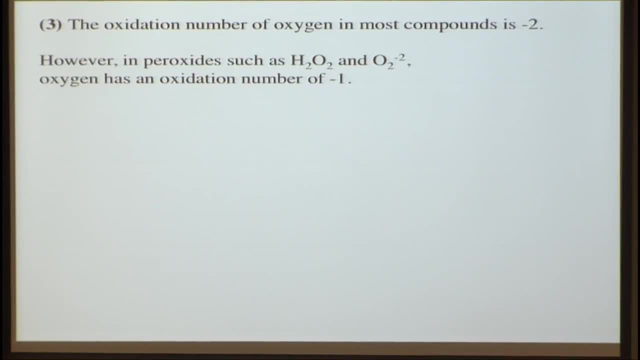 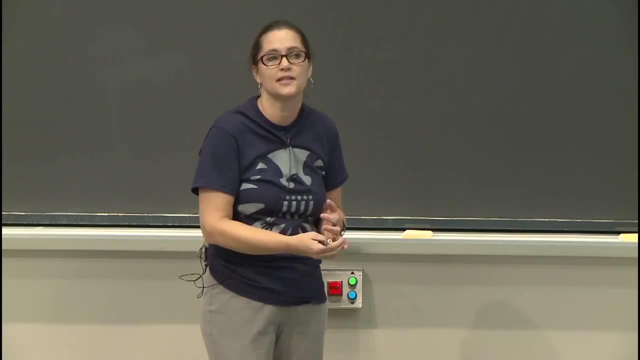 hydrogen peroxide, O2, two minus, then it's going to have an oxidation number of minus one. So peroxides- and later we'll see superoxides- are exceptions, But if it's not a peroxide or a superoxide, 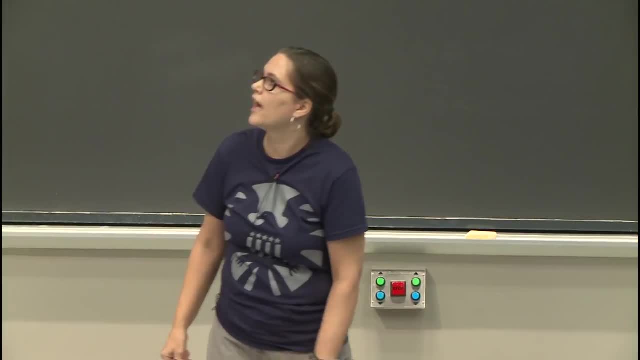 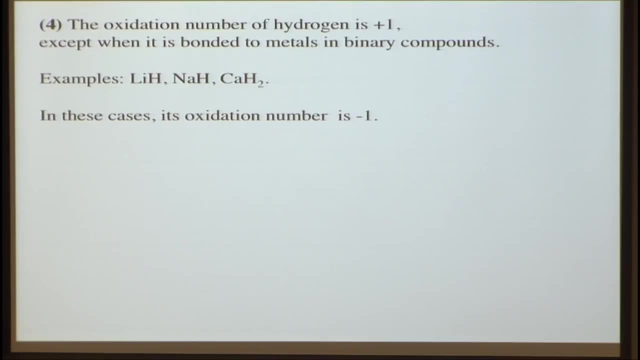 it's going to be minus two, All right. rule number four: Hydrogen. Hydrogen is mostly plus one. You probably could guess that, But there actually are some exceptions for this And you're going to see a lot of those exceptions in this unit. 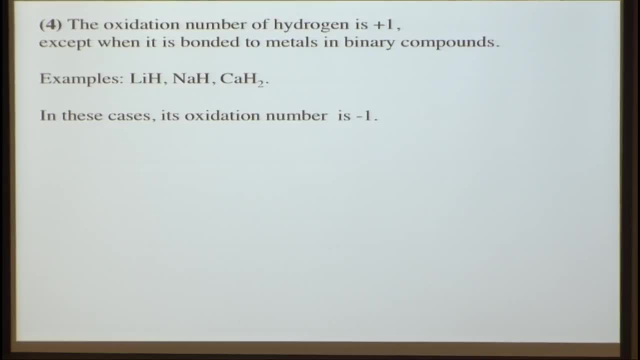 And pretty much after this unit, not so much ever again. The exceptions are for the group one and the group two, So the group one and group two rules supersede the fact that hydrogen is usually plus one. So if you have hydrogen with lithium, 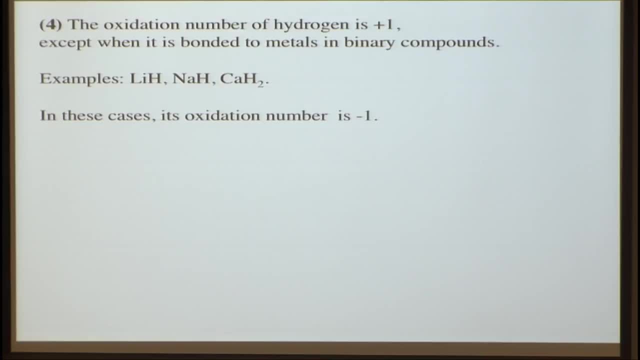 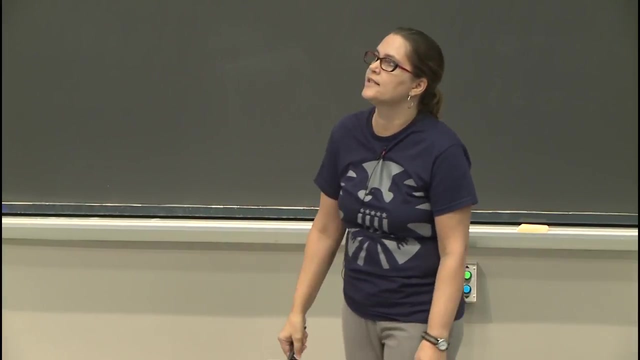 lithium is going to be plus one, So hydrogen will be minus one. Sodium is the same here And calcium, that's group two. Again, hydrogen would be minus one, So group one, group two. rules supersede hydrogen. All right, what about our halides? 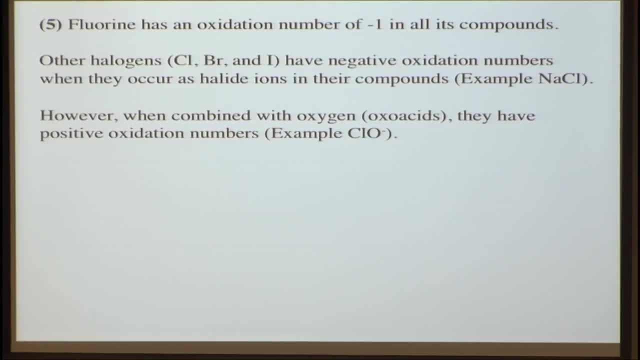 We have fluorine, It wants to be minus one. Other halogens- chloride bromide iodide- are negative when they are in salts Such as sodium chloride. But if oxygen is there, the oxygen rules are the ones that follow. 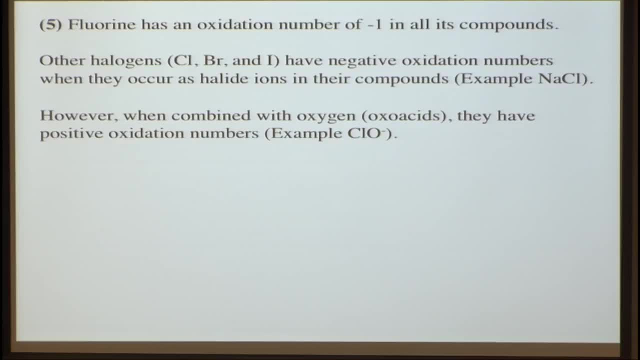 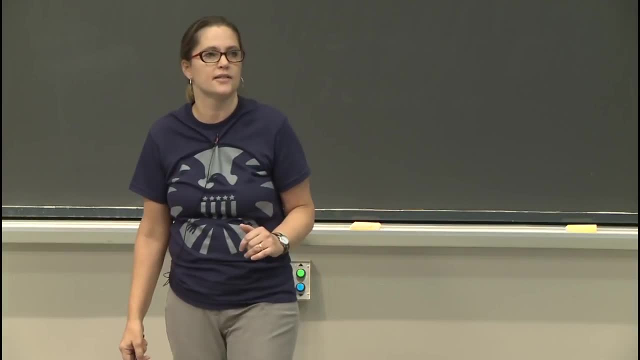 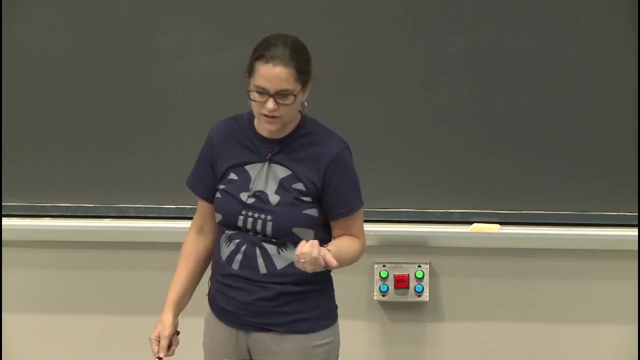 So here, if you have Cl with oxygen, then you're going to have a positive oxidation number for the chlorine, Because oxygen is going to be minus two, All right, and you'll see a number of these so-called oxy acids in this unit. 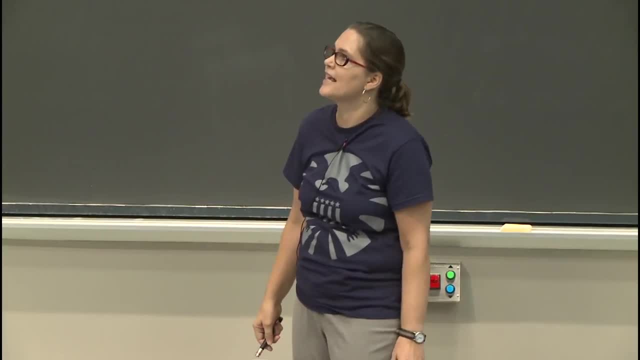 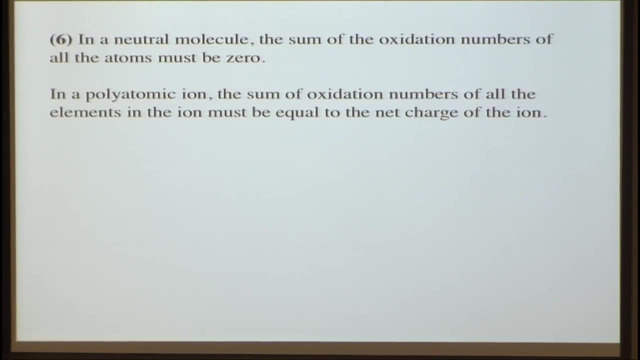 All right, Six. This one you probably already know. but in a neutral molecule the sums of the oxidation numbers must equal zero. So the sums must be neutral if the molecule is neutral And if you have something that is a polyatomic, multi-atom ion. 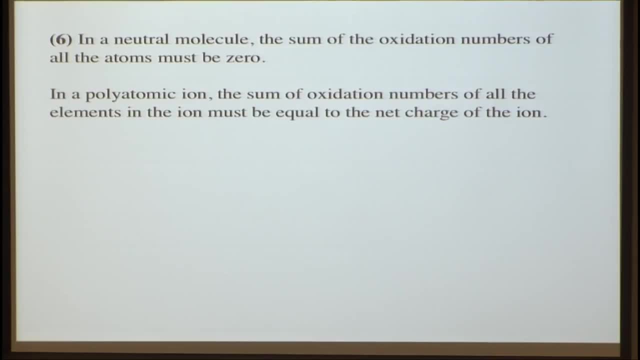 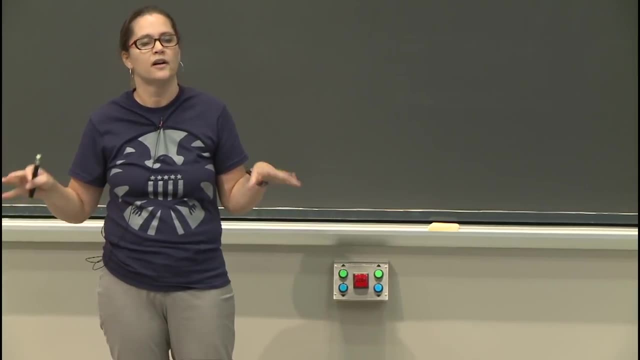 the sum of the individual oxidation numbers needs to be equal to the overall charge on that ion. So again, we've seen things like this before, so we should have no trouble with these rules. Okay, so let's just look at an example of this. Suppose we have our friend NH4+. What is hydrogen's oxidation number going to be in this molecule? It'll be plus one. So it's not with a group one or group two element. so it's going to be plus one. What about nitrogen? 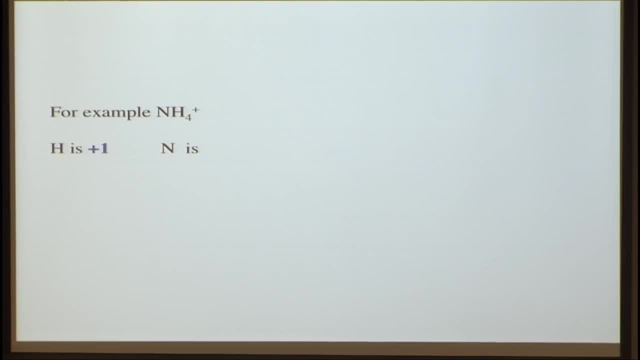 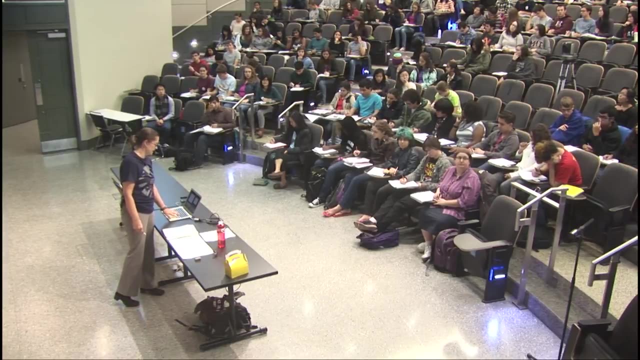 There are no rules about nitrogen, so we have to figure out, based on the other rules, what the oxidation number of nitrogen will be. What is it going to be here? It's going to be minus three, and the reason for that is because of the rule we just talked about. 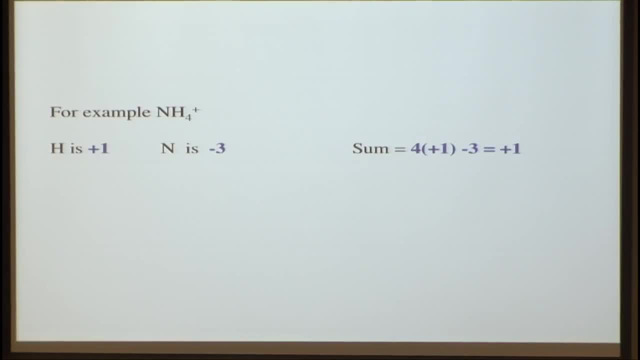 that the sum of the oxidation numbers needs to be equal to the charge on the molecule. The charge is plus one. so we have four hydrogens. four plus one. minus three is going to equal plus one and the nitrogen had to be minus three. 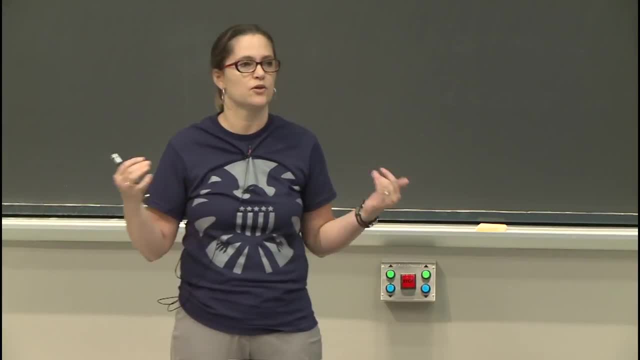 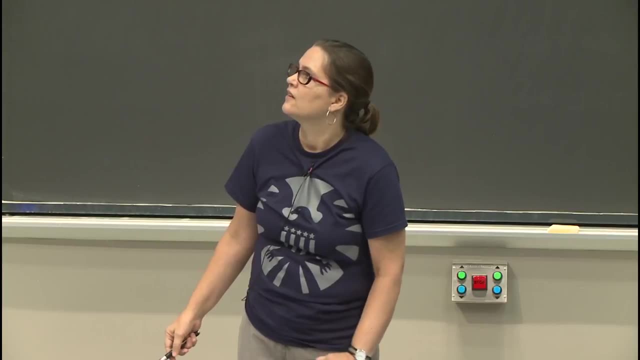 Nitrogen can have a lot of different numbers, so you want to pay attention to what's around it and whether there are rules or guidelines about those other elements. All right, seven Oxidation numbers don't have to be integers. They almost always are. 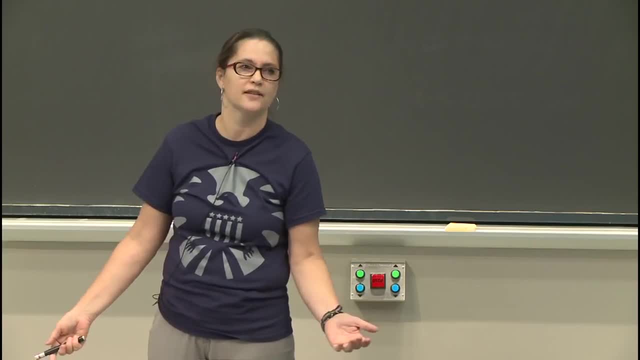 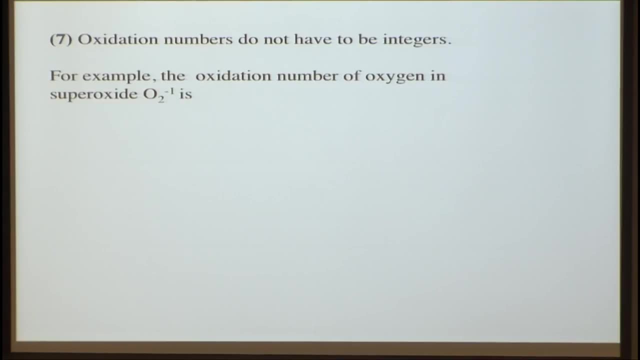 but there is one notable exception and it's from oxygen. Perhaps not a surprise. Oxygen is always causing trouble, So in superoxide you have O2 minus one. So what is the oxidation number on each oxygen in that O2 minus one molecule? 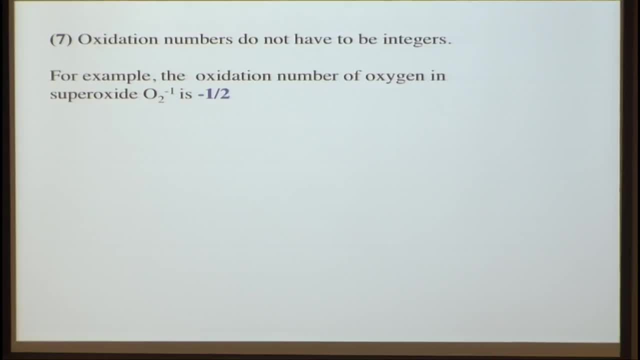 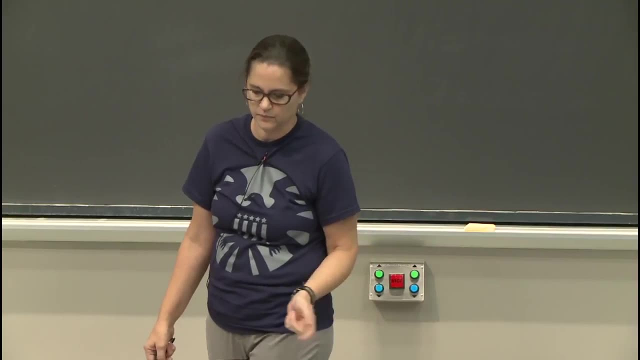 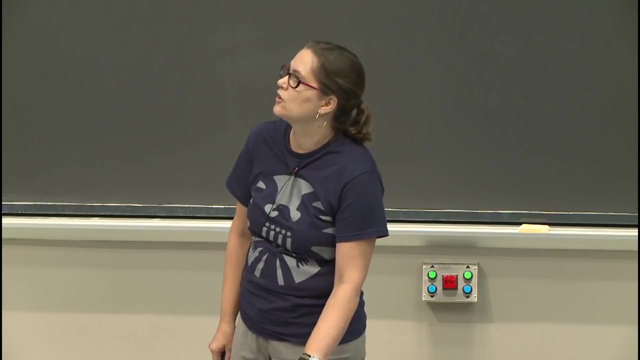 Yup, so it's minus one half. So oxygen is usually minus two, except in peroxides and superoxides. All right, so let's take a look at some examples, and I'll write some of these on the board, and here are all of your rules. 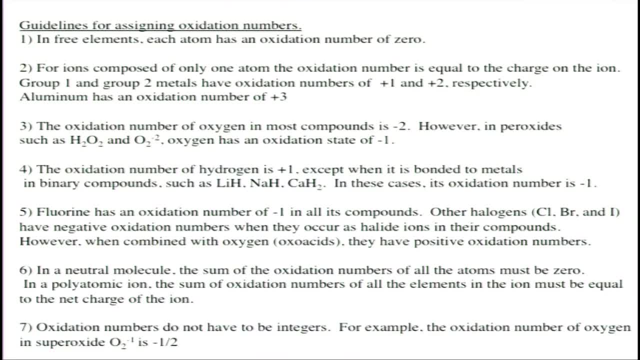 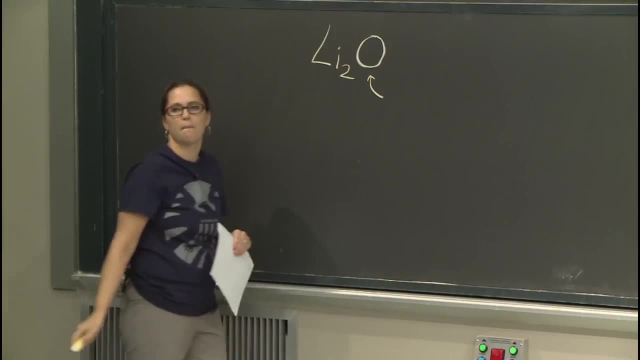 so you can yell out what you think I should be doing with these as we go along. Okay, so we have lithium to oxide, So here we know a lot about this. What's the oxygen going to be? Minus two, The overall charge on the molecule is zero. 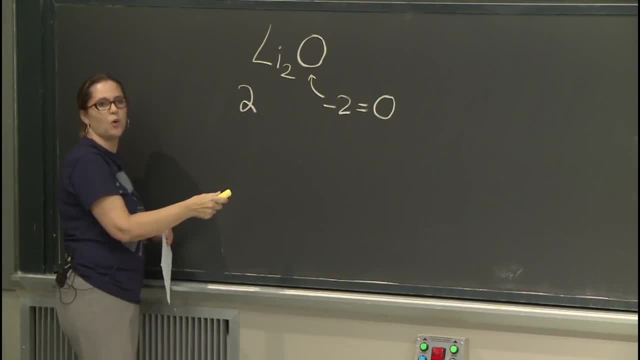 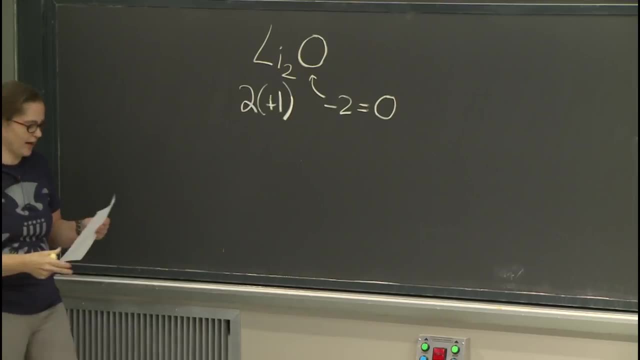 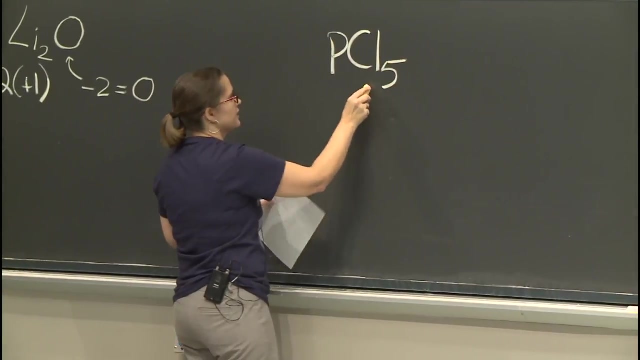 and we have two lithiums, and what's the charge on each one? Plus one, Plus one, And so plus two, minus two is zero. Great, Let's do another one. We'll do PCl5 next. So what do we know about Cl? 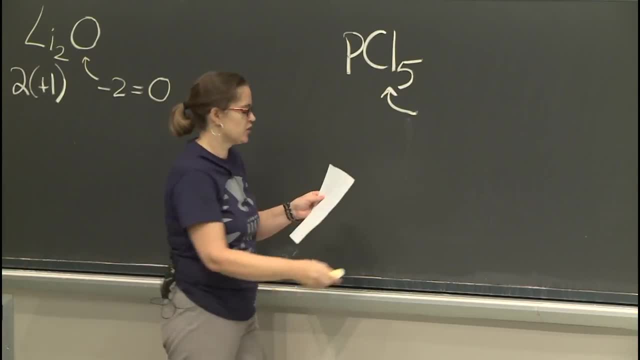 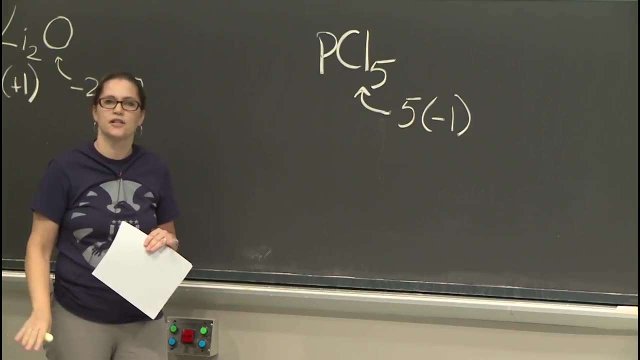 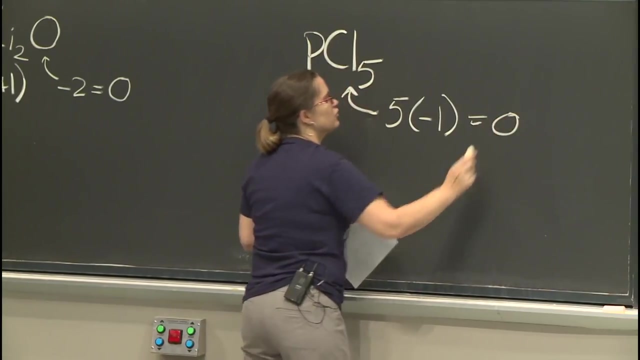 What charge do we expect here? Minus one, and there are five of those. So chlorine likes to be minus one Exception is with oxygen, but it's not with oxygen. here The overall charge is going to be zero because it's a neutral molecule. 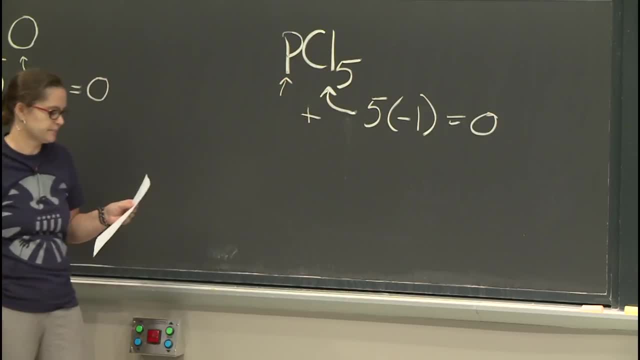 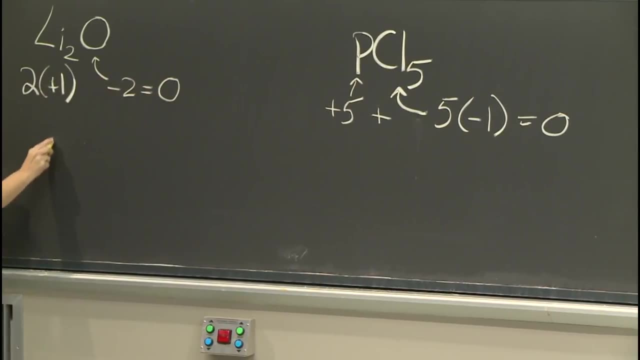 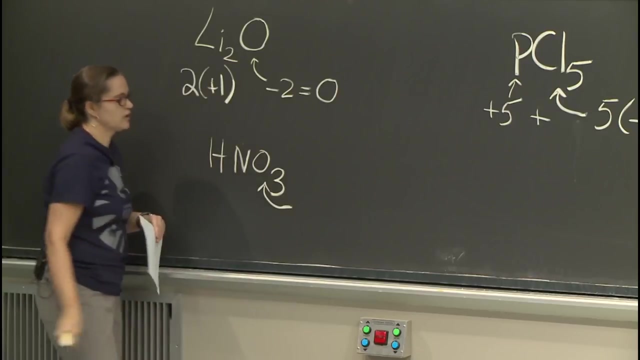 So what does that mean about the charge on our phosphorus Plus five Plus five, Right, Okay? so now let's try HNO3.. So let's do oxygen first. What charge do we expect on oxygen Minus two? 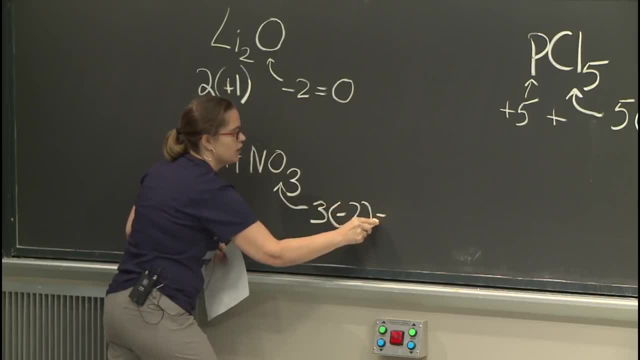 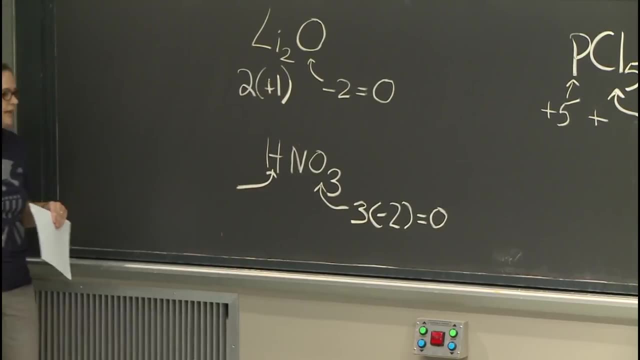 Minus two, So we have three of those minus two. Overall this is going to be zero. Nitrogen can be varied, so let's do hydrogen. What do we expect hydrogen to be? Plus one, Plus one? right, because it's not with a group one or group two. 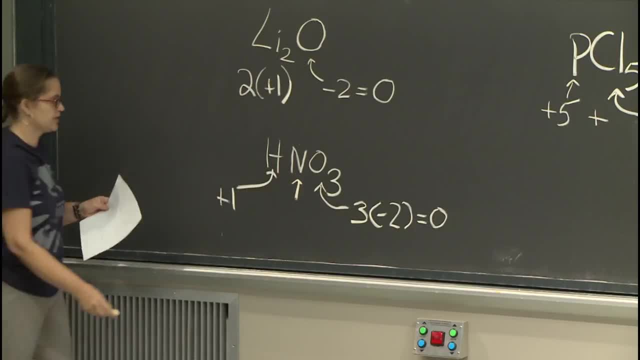 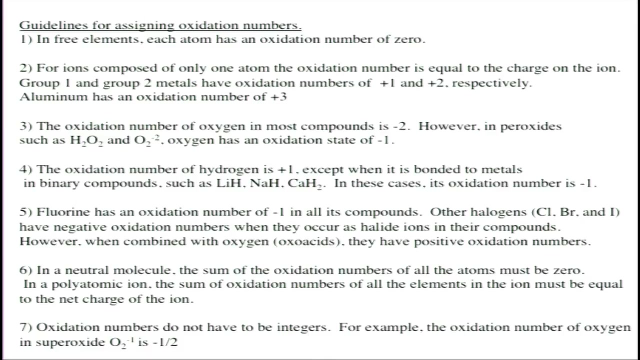 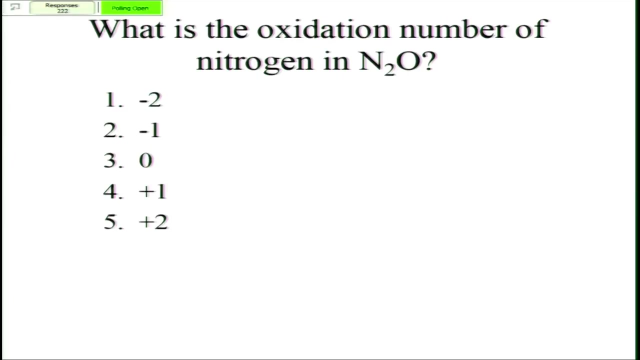 So what does that leave for nitrogen Plus five, So we have plus six, then Minus six is zero. All right, So why don't you try the next one, which is a clicker question? All right, Ten more seconds. So oxygen is minus two. 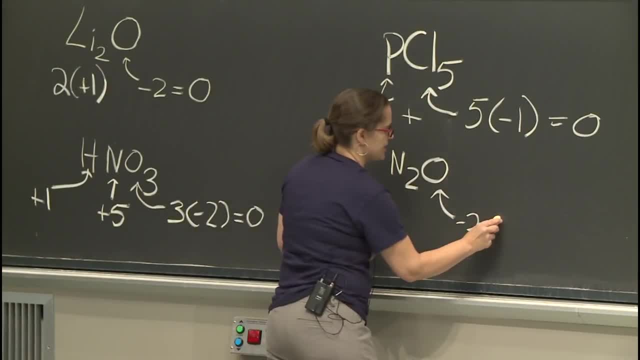 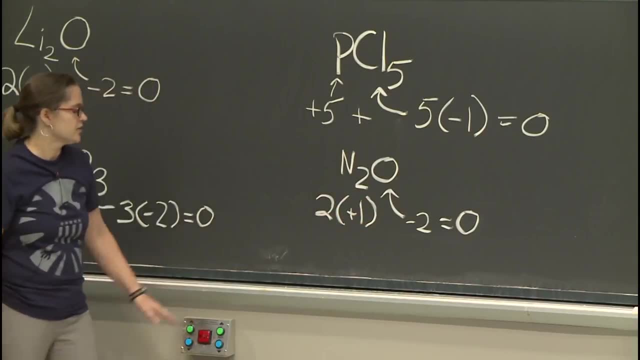 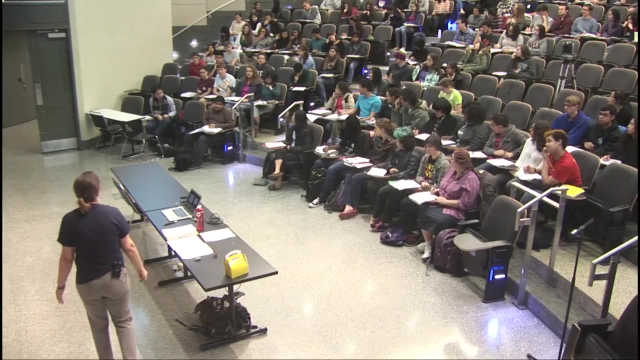 It's not in a peroxide or a superoxide. The overall charge is zero. So that means that each nitrogen must be plus one. So we have plus two, minus two is zero. Yeah, What exactly is a peroxide? A peroxide? 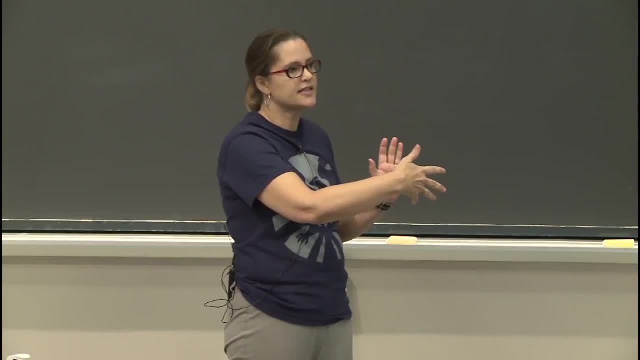 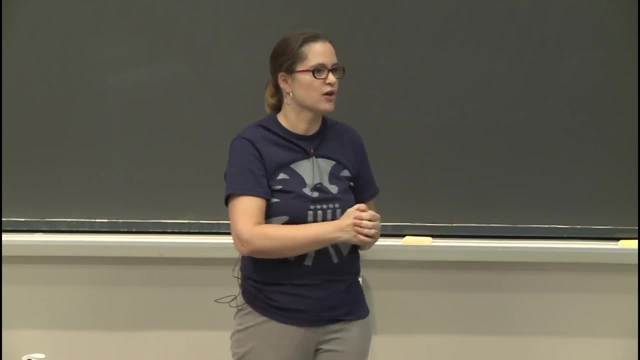 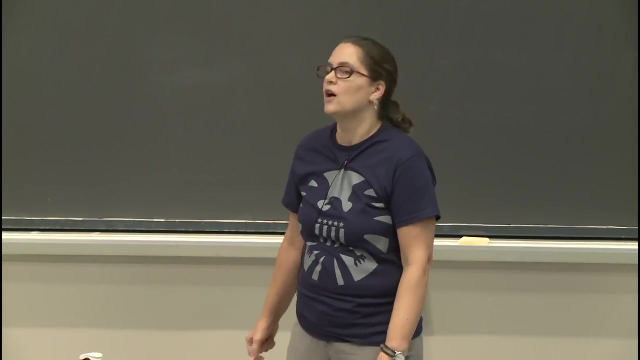 So there really only goes the hydrogen peroxide example. So it'll say that it's a peroxide or a superoxide. Yeah, So you don't have to worry about that, It's going to be clear, Okay, Good, So now let's talk about some reactions. 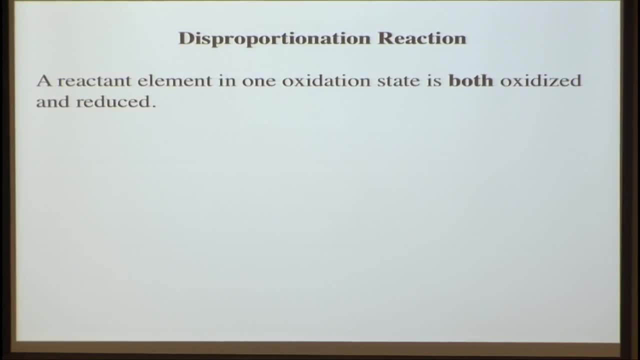 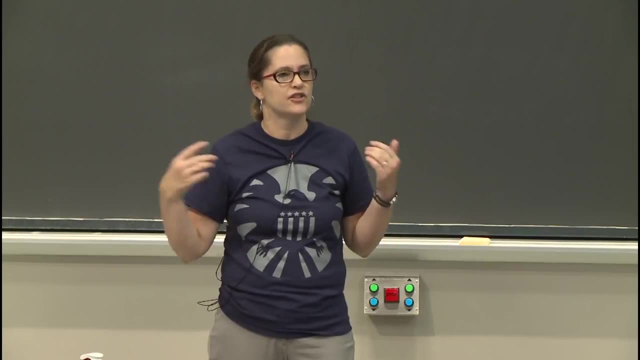 that involve oxidations and reductions, And to talk about these reactions, you need to know how to do this, And then we're going to talk about balancing reactions, And you need all of these skills, All right, So first I just want to tell you about something called 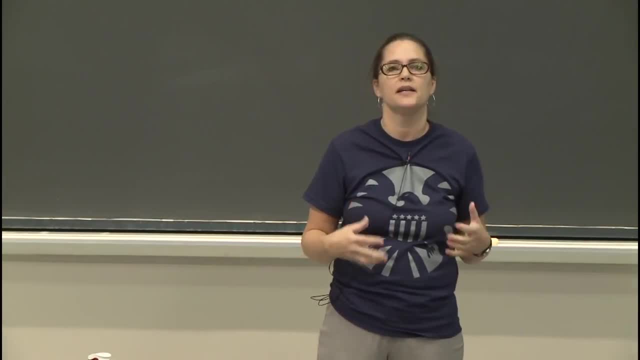 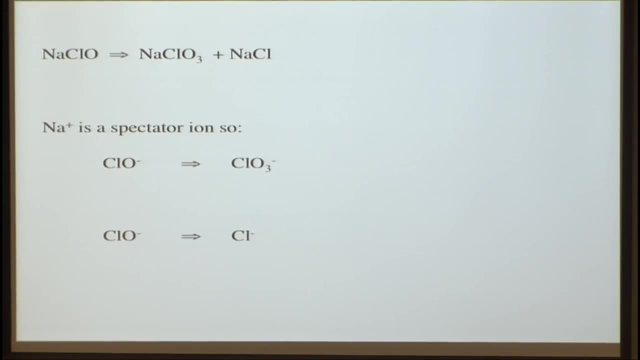 the disproportionation reaction, where you have one element that is going to be both oxidized and reduced, And this is a good example to allow us to think about what's happening in a different reaction. So in this reaction, the element that is going to be 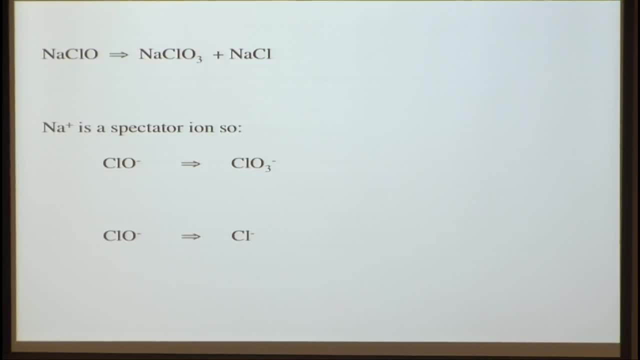 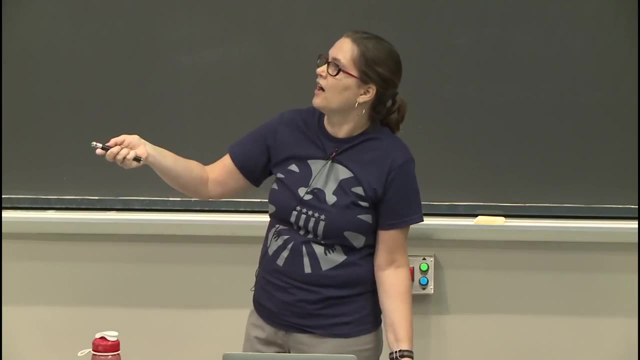 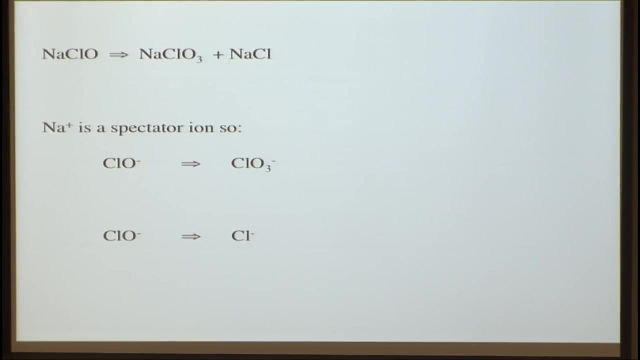 both oxidized and reduced, is Cl. Sodium is going to be a spectator ion And the oxygen is going to stay in its minus 2 form here, And so we have chlorine going to chlorine in this compound and in this compound. So we can break this down. 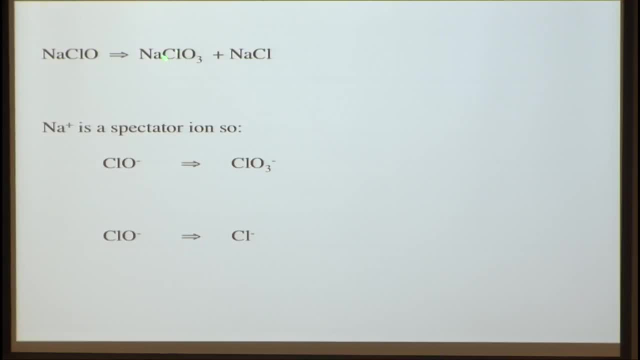 and think about what's happening with this species going to this and then also going to Cl- So let's think about what the oxidation number of chlorine is in ClO-. So first oxygen, I already told you is going to be minus 2.. 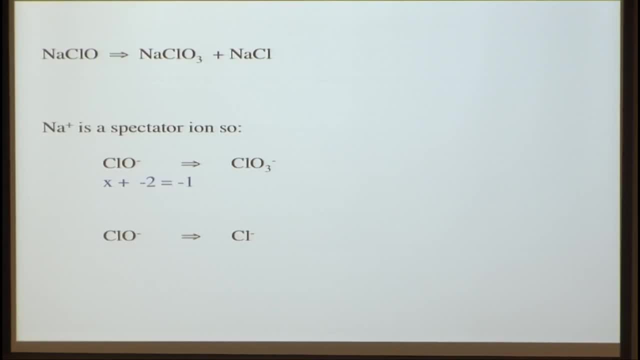 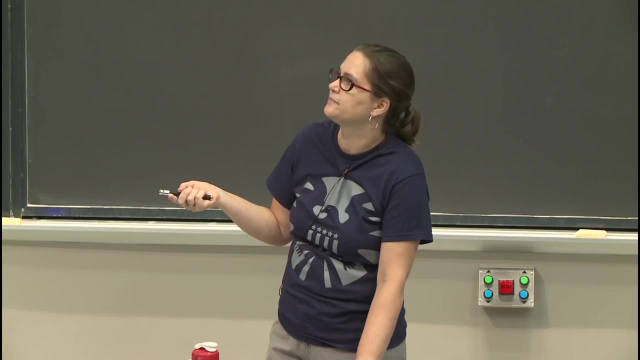 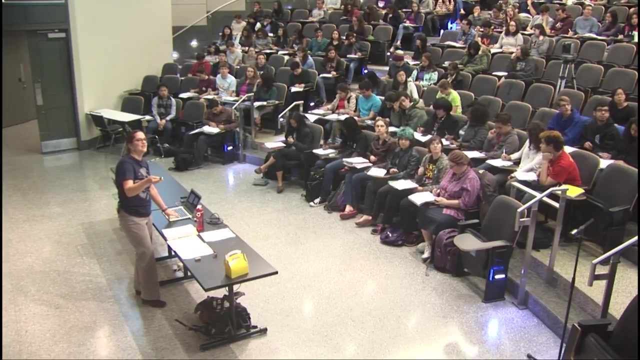 The overall charge on the molecule is minus 1.. So chlorine has to make this equation work. So what is the oxidation number of Cl Plus 1,? thank you. So we have plus 1 here. Now let's take a look at this. 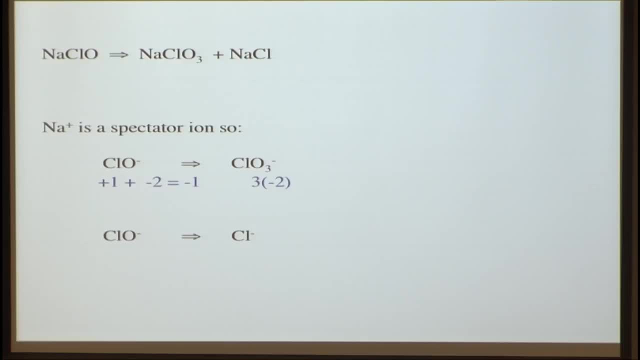 So oxygen we're going to have as minus 2.. There are three of them. That's going to equal overall minus 1.. So what's the oxidation number of Cl here? Plus 5, right. So we have a case now where we're going from plus 1 to plus 5.. 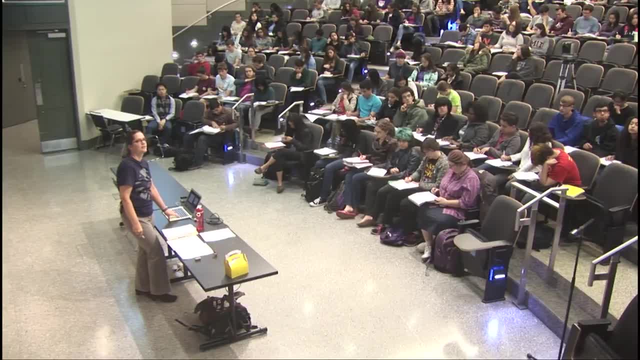 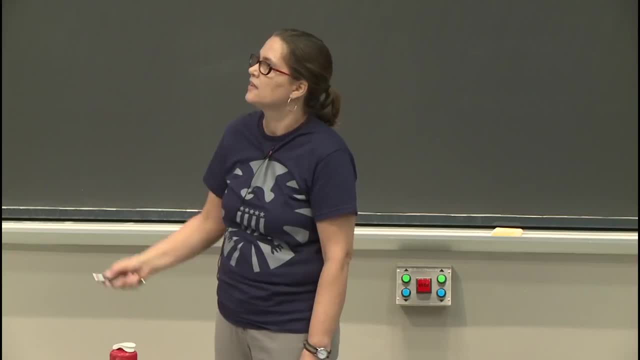 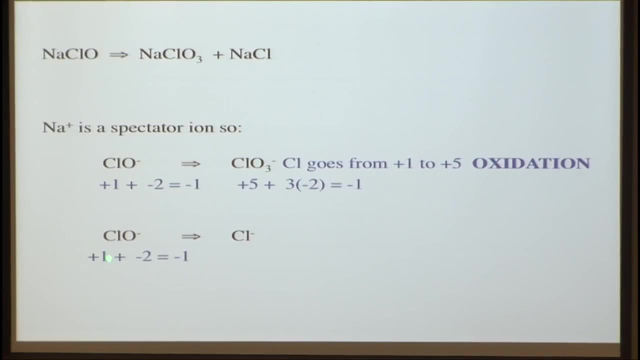 Is that an oxidation or a reduction? That's an oxidation, So we're increasing the number. It is losing electrons, It's becoming oxidized. So down here we already have done all of our work and know that this is also going to be plus 1.. 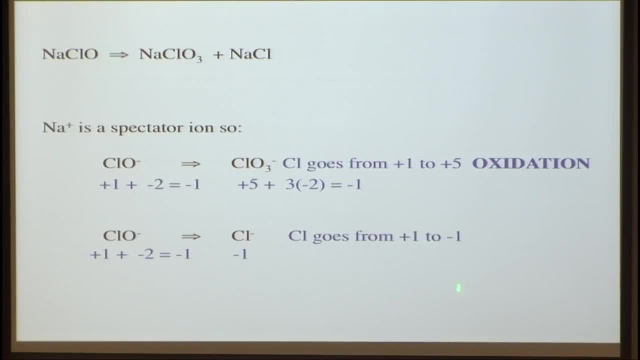 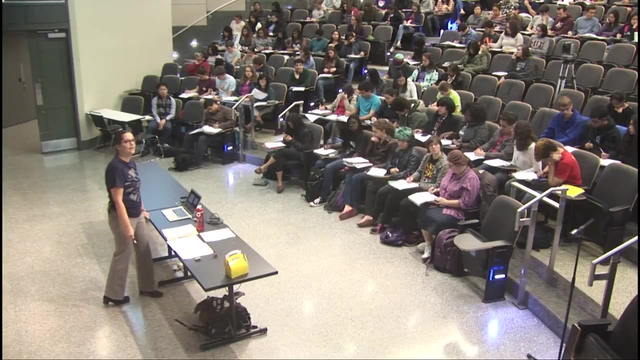 So in this case we're going from plus 1 to minus 1.. Is that an oxidation or a reduction? That's a reduction and that's good, because it wouldn't be a very good disproportionation reaction. Otherwise, something has to be oxidized. 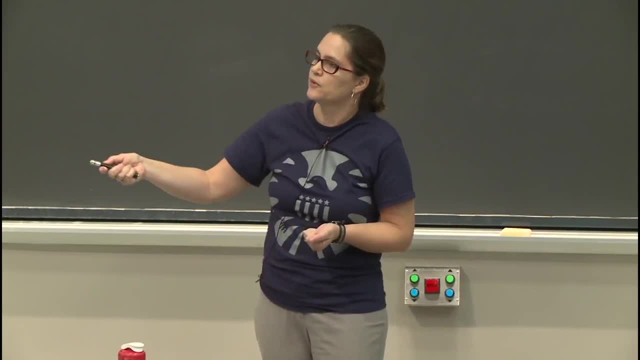 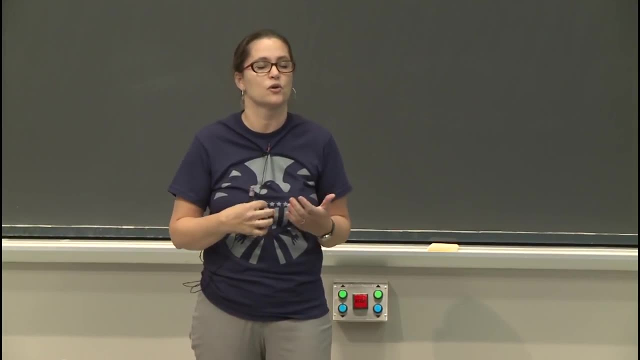 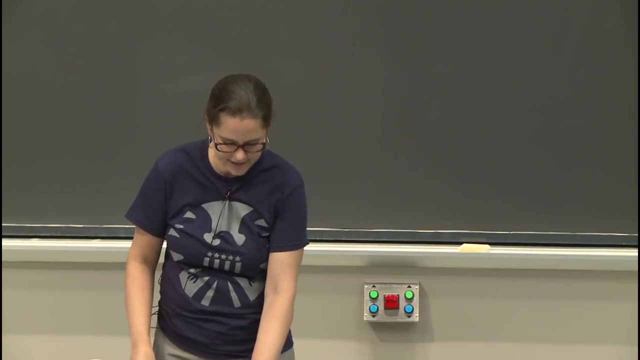 Same thing has to be oxidized and reduced. So this is how you think about this type of reaction. So to consider whether something's being oxidized or reduced, you need to be able to dissect out what the oxidation numbers are. All right, now we're going to balance. 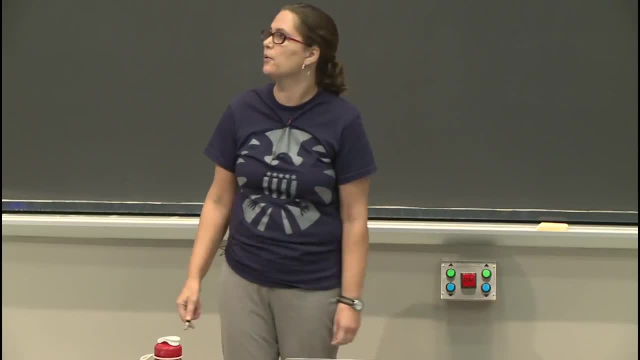 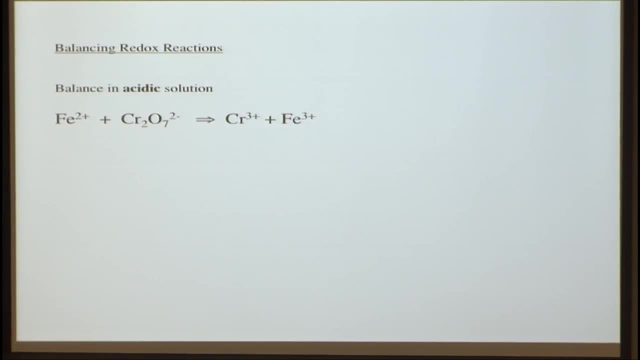 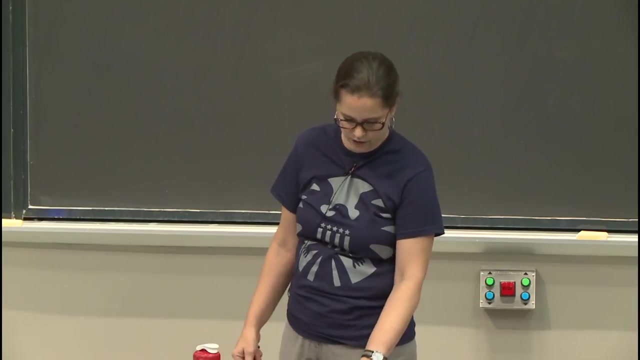 So balancing is going to become very important for doing problems later on, Balancing redox reactions. You balance differently if you're in acidic conditions versus basic conditions. So first we're going to do acidic conditions And we're going to run through the steps for doing this. 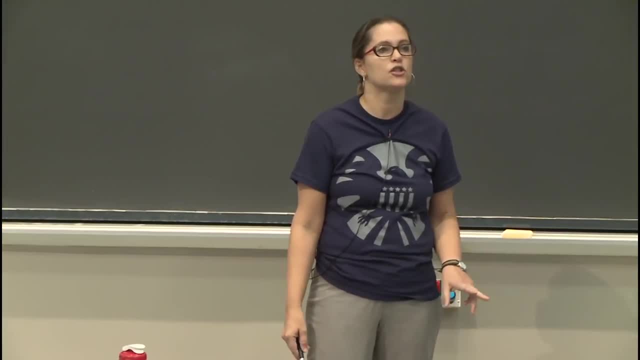 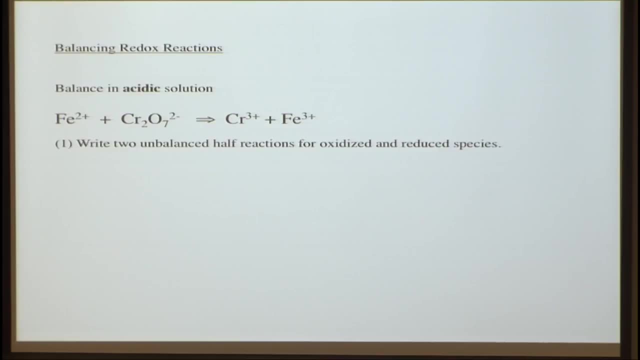 First step is we're going to write two half reactions for this. So we have iron in here and we have chromium in here, And we're going to separate those out because we're going to think about what iron is doing separately from what the chromium is doing. 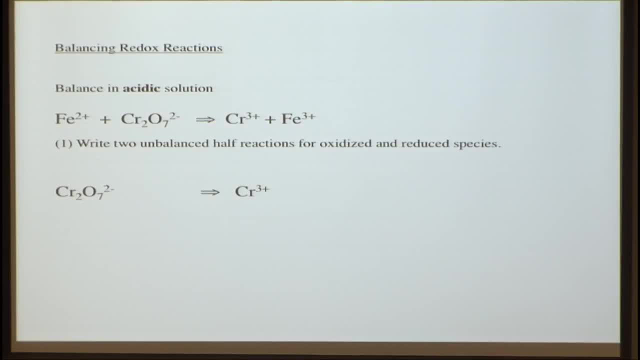 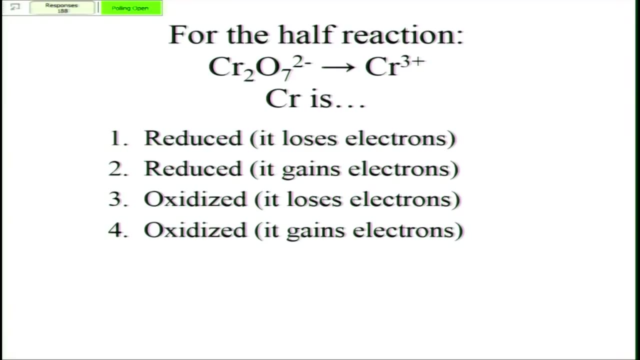 So first let's write out our chromium and think about what is happening to it here. And that is a clicker question. All right, 10 more seconds, Okay. So let's take a look at why two is correct. For one thing, you just have to remember the definitions. 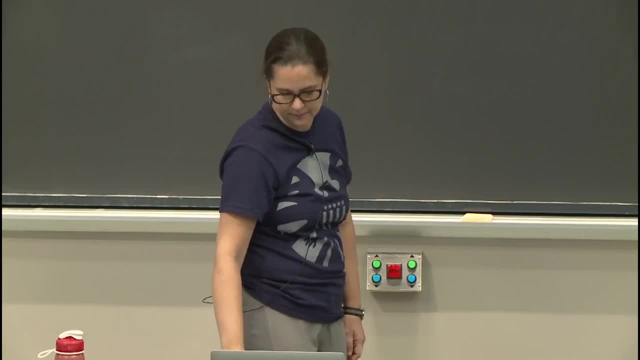 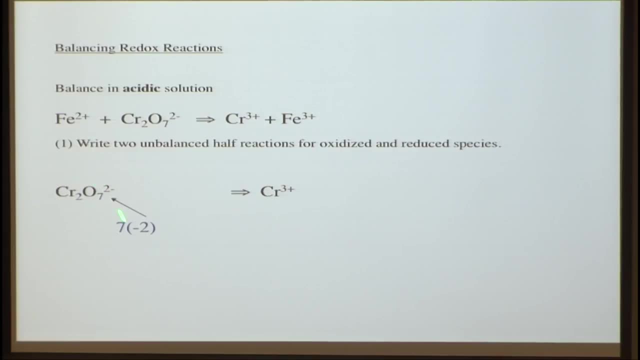 For another. you have to recognize what's happening to the chromium. So let's take a look at the chromium now. So we have oxygen at minus 2.. There are seven of them And the overall charge of the molecule is minus 2.. 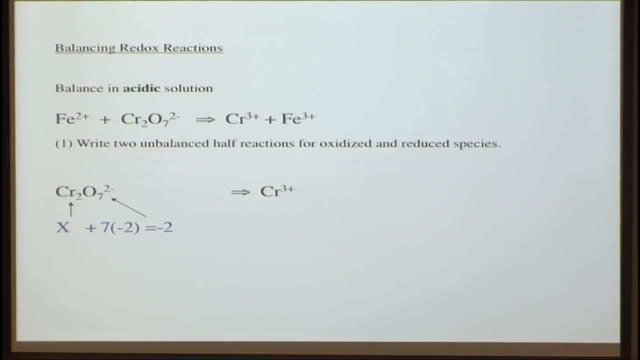 And so what does that mean for the oxidation number of this chromium? It's going to be plus 6, because we're going to have 12 minus 14.. 12 minus 14 equals minus 2.. So we're going from plus 6 over here to plus 3 here. 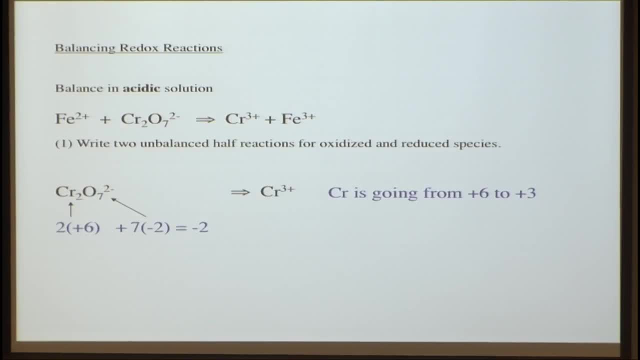 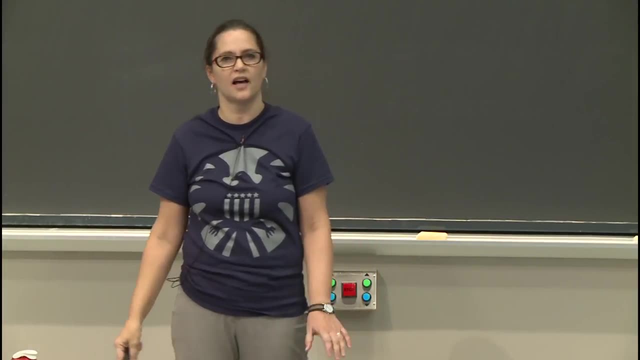 So is that an oxidation or reduction? So that's the reduction. So I kind of like this unit coming after acids and bases, because a lot of those problems, I think, make people's brains hurt a little bit. And you get here and it's like basic math. 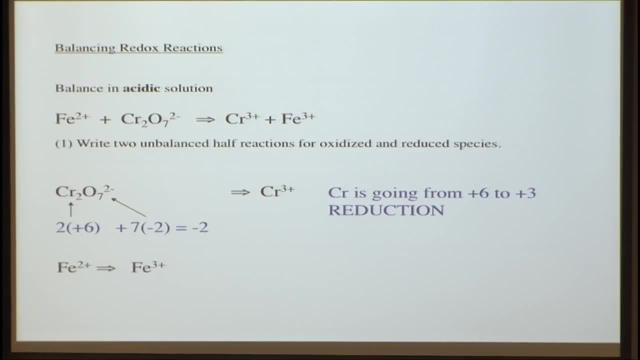 So it's kind of exciting, All right. so the iron is even simpler. We're going from plus 2 to plus 3.. So that's an oxidation. So one thing is being reduced, The other thing is being oxidized. That's what makes it a redox reaction. 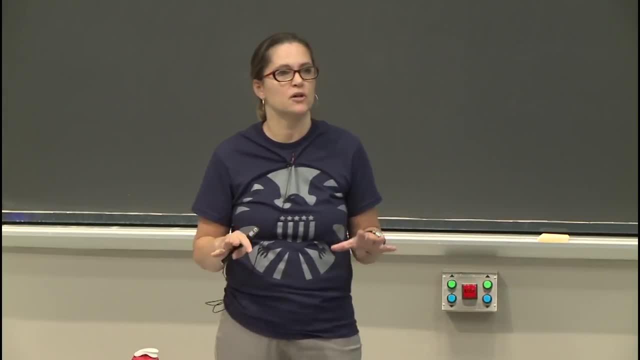 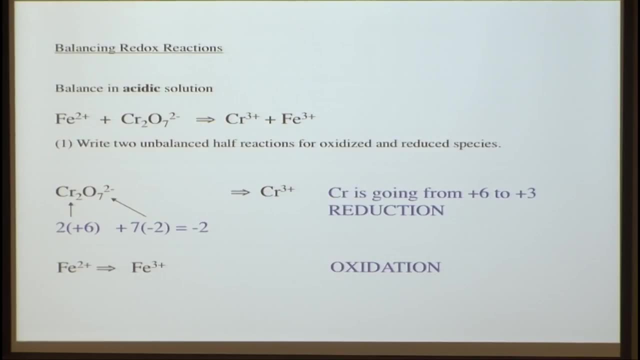 All right. so we know what's happening in terms of what's being oxidized, what's being reduced, And we've broken these into two half reactions. Now we need to balance, All right. so the first thing we're going to do, 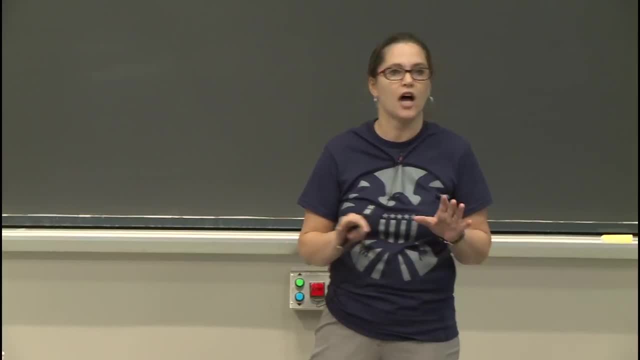 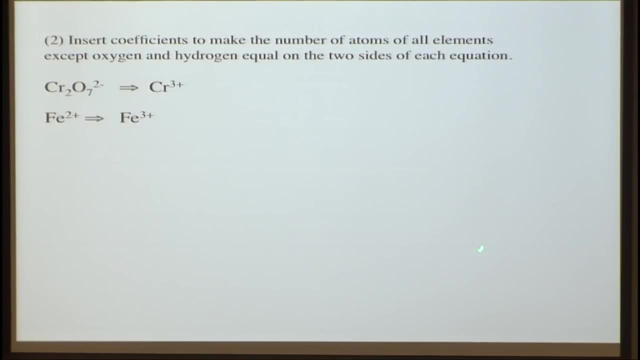 is, we're going to balance our elements that are not oxygen and hydrogen. So we're going to balance chromium and we're going to balance our iron. What do we need to add to this top? to balance chromium, We need to add a 2.. 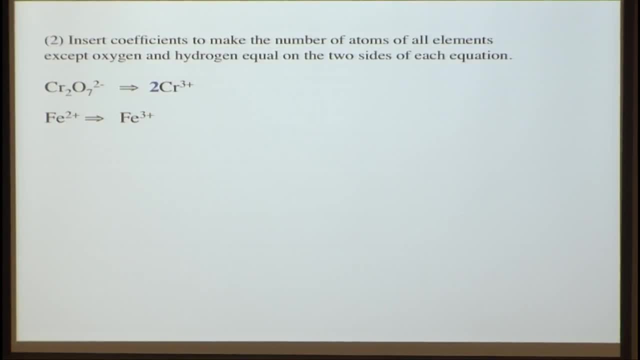 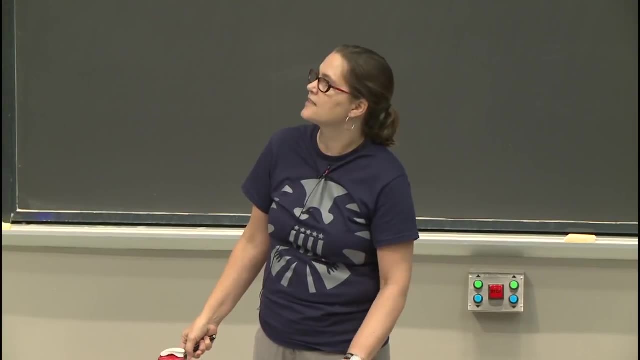 And we don't need to do anything to our iron. We have one iron on one side, one iron on the other side, All right. so all you need to do is insert the 2.. Next step: We're going to add water to balance oxygen. 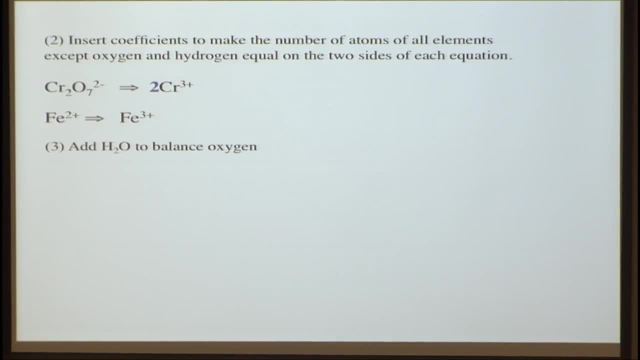 So how much water do we need to add to the top reaction to balance the oxygen? So here we're going to add 7 waters to balance the oxygen And again we have nothing to do down there. All right, so let's keep going. 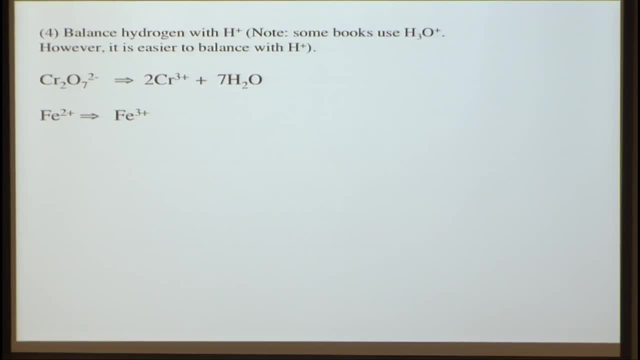 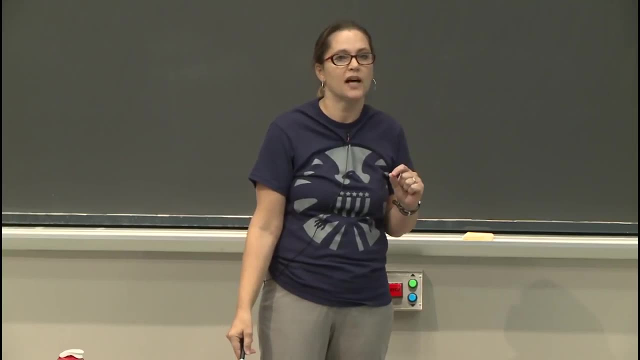 Next, we want to balance the hydrogen. We just added those waters And so now we have to balance hydrogen. So we're going to balance the hydrogen by adding H+. Some books have you balance the hydrogen by adding a more correct species, which is hydronium ion. 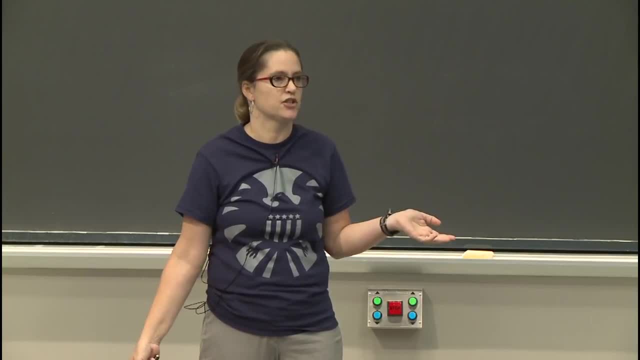 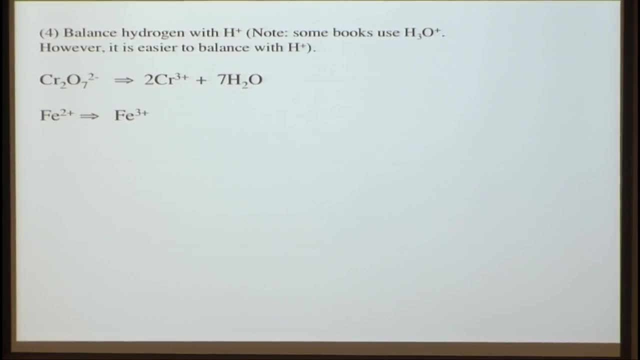 But when you do that you screw up your oxygens that you just balanced. So that is infinitely harder to balance equations that way. So I say let's not do that, So let's just use that. So let's just use H+. 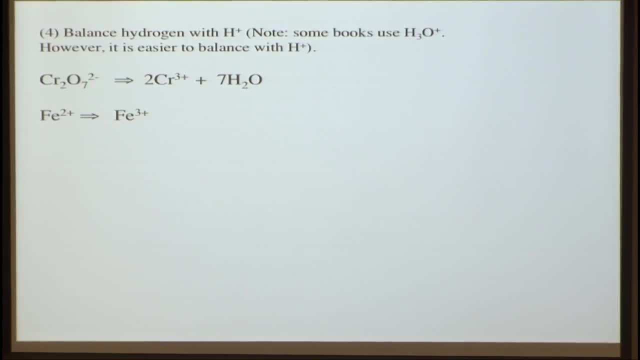 So how many H pluses do we need to add over here to balance the hydrogen 14.. We've added 14. And again, we don't have to do anything to the bottom expression. Next, we are going to balance the charge. 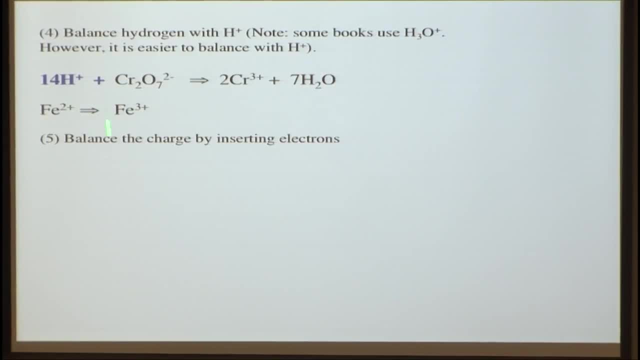 by inserting electrons. So over here we have 14 minus 2 plus 12.. And over here we have plus 6.. So how many electrons are we going to need to add? We're going to need to add 6.. 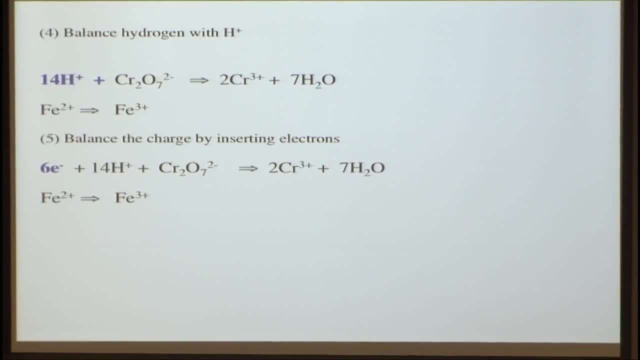 So we've added 6 over here, So they have a negative charge. So now we should be balanced on both sides And now we finally get to do something with the bottom expression And we can add an electron over here to balance the charge. 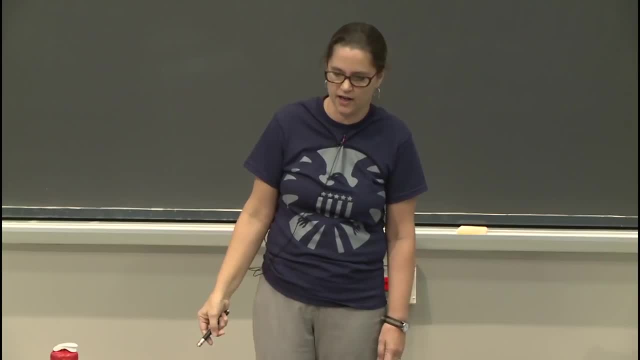 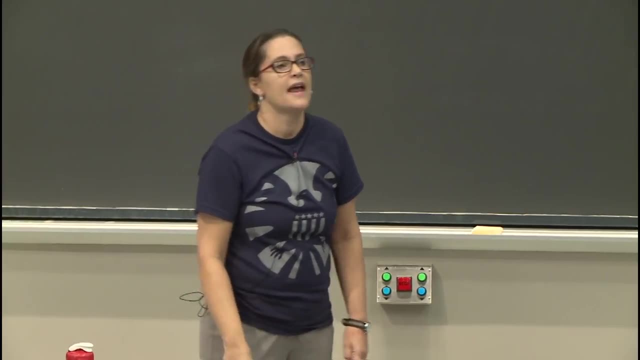 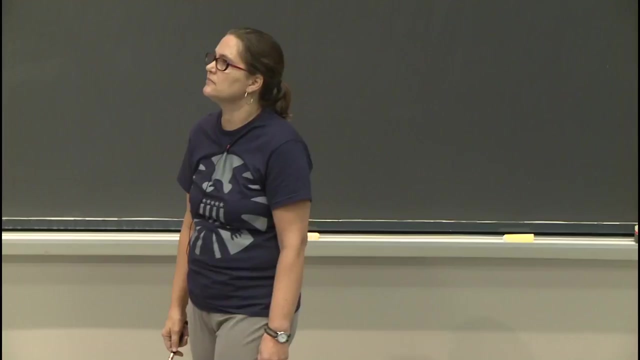 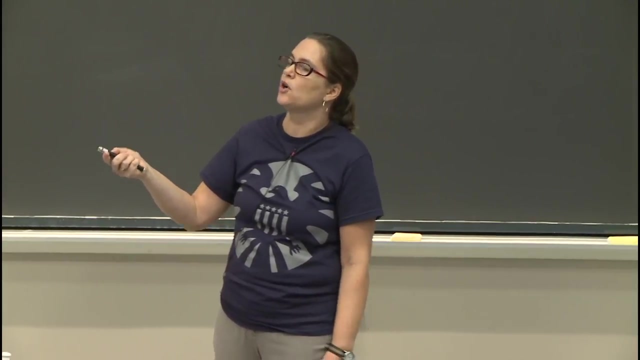 So plus 2 here, plus 2 net on the other side. All right, Now we want to multiply so that the electrons are going to cancel, Because this is an overall oxidation-reduction reaction and our electrons should cancel. So what do we need? to multiply the bottom equation by: 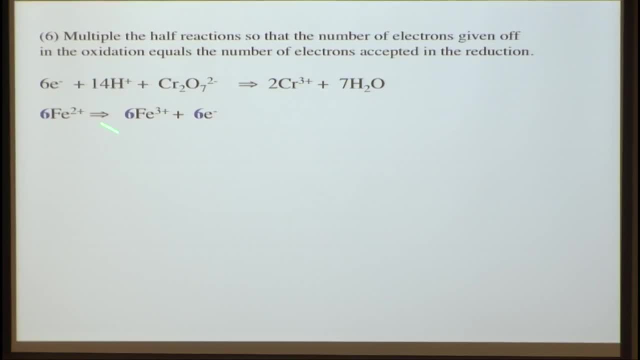 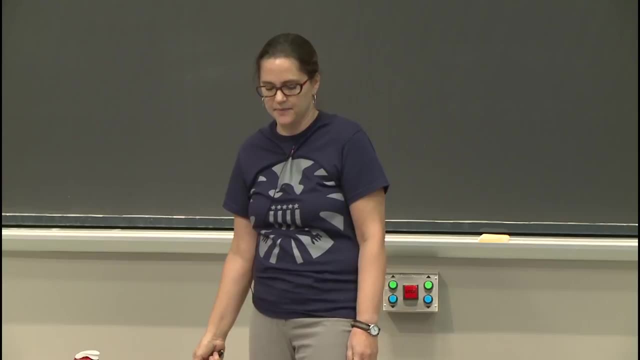 6. And there we go: 6 here, 6 here and 6 here. Now, this is one of the places where people often in exams make a mistake, where they write 6 and then put parentheses around it. 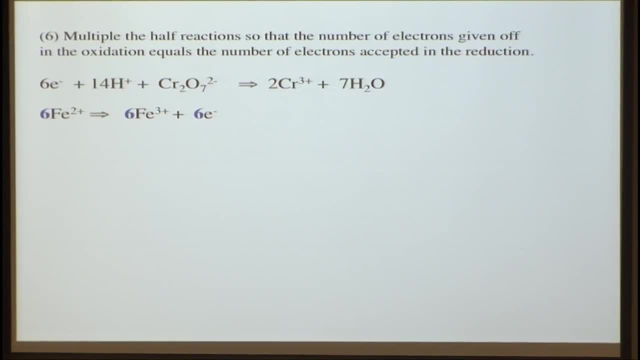 indicating that you're multiplying the whole thing by 6, which is fine, But then they forget to actually carry that out on the next step. So when you multiply, make sure that you continue to, if sometimes it's better just to write it all out. 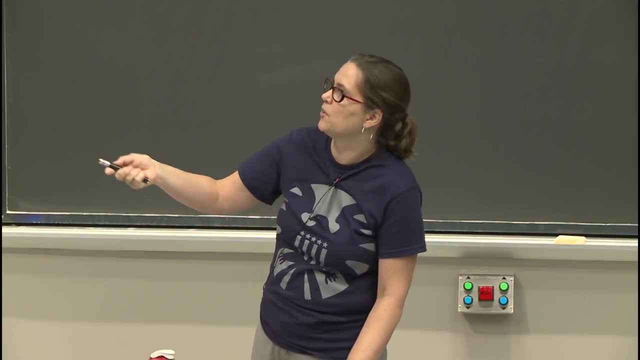 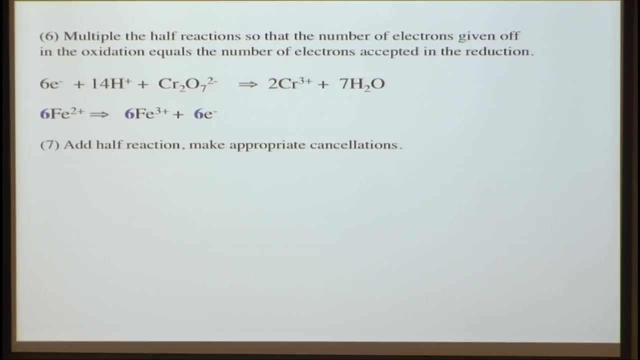 because otherwise it's really easy to forget and not multiply and then things won't make sense at the end. All right, So now we can add the half reactions and make the appropriate cancellations. So we've now added it all together: 6 electrons 14H+. 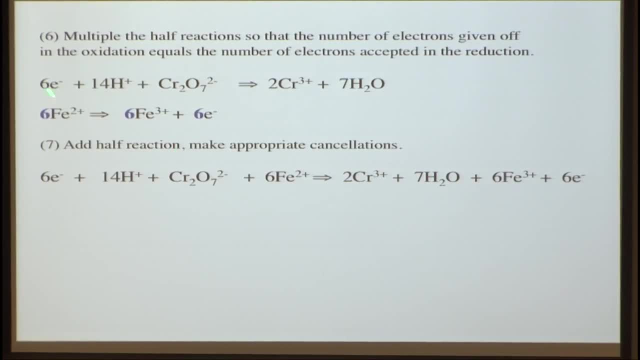 We have our chromium oxide compound. We have now our 6 iron plus 2s, our 2 chromium plus 3s, our 7 waters, our 6 iron plus 3s and our 6 electrons. And if we did everything right, 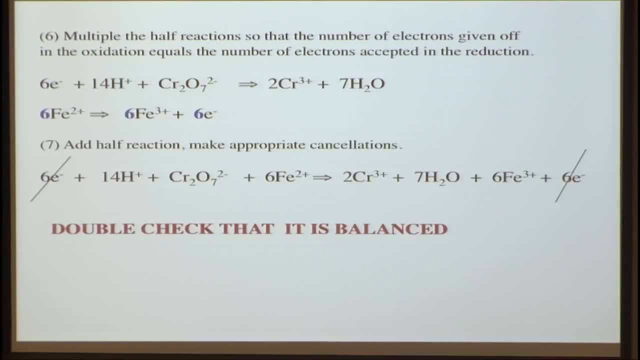 then the electrons should cancel and we can double-check. It's always a good idea to double-check that it's balanced. So we have 14Hs here, 14Hs there. Chromium 2, 2.. Oxygen 7, 7.. 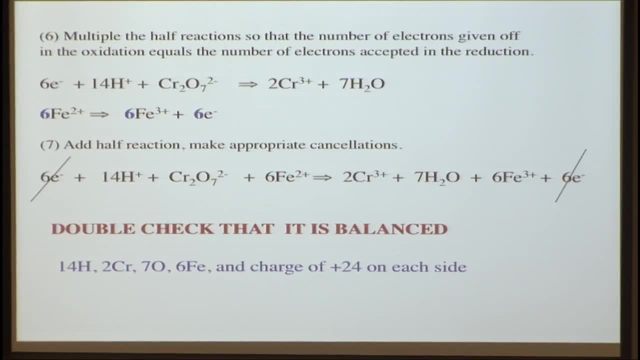 Iron 6, 6. This can catch a mistake that you might have made And then check the charge: Plus 14, minus 2, plus 12 on one side, plus 6, plus 18.. So 24 on both sides. 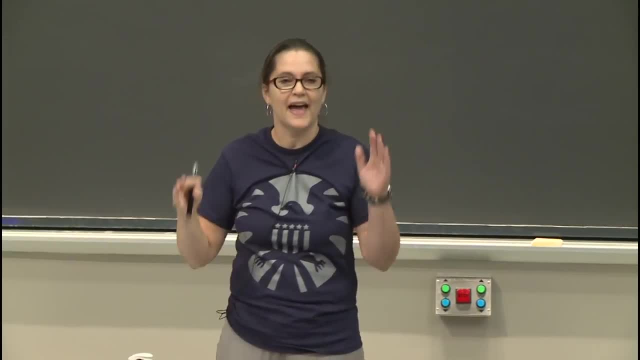 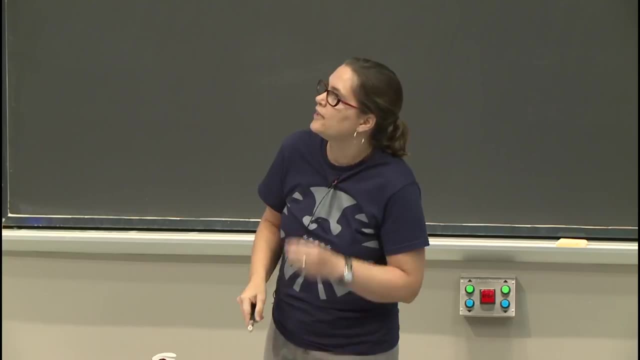 It's pretty good, right? That's pretty simple. So balancing: That's an acidic solution. We know it's an acidic because we have 14H+ That feels quite acidic. What do you do for basic solution now? So for a basic solution. 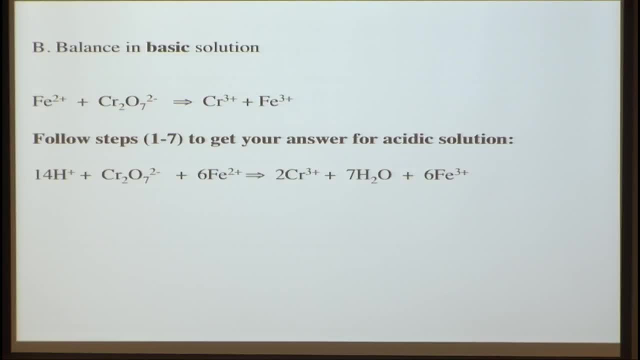 what I recommend is just do the exact same thing that you did for your acidic solution- And here again was the answer that we have- And then quote: neutralize the acid and make it basic. Adjust your pH by adding OH-, our hydroxide ion concentration. 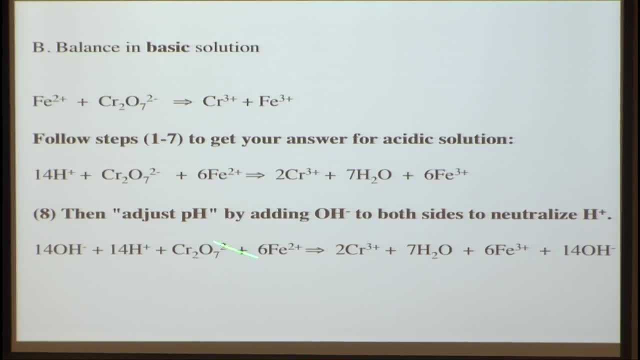 to each side. So if we do that now, we're going to add 14OH- to this side and 14OH- to that side. Now 14OH- plus 14H+ are going to give us 14 water molecules over here. 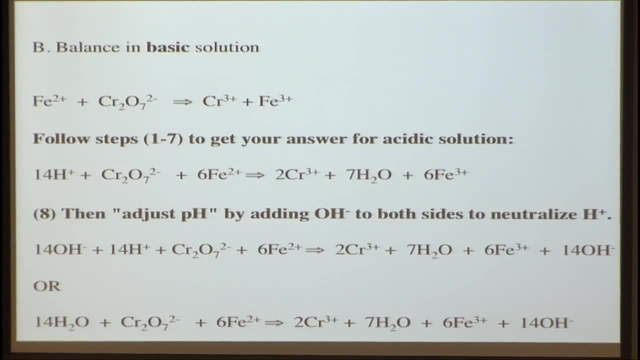 And on this side we still have 14OH. Now we have 14.. This is not simplified, because we have 14 waters on one side and 7 on the other side, So we can take that, cancel out these 7,. 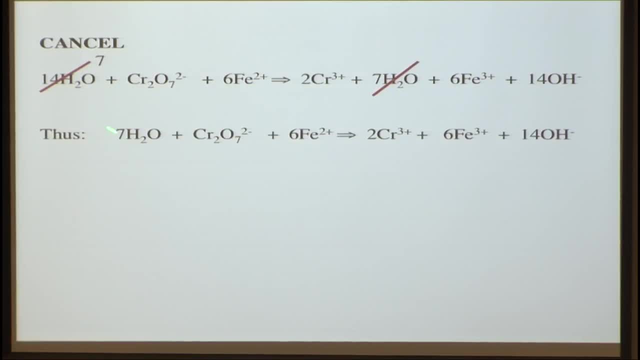 and we have 7 left over here. So we have 7 waters now on one side and 14 hydroxides on the other. So if we look at both of these expressions in acidic solution and in basic solution here, in acidic solution- 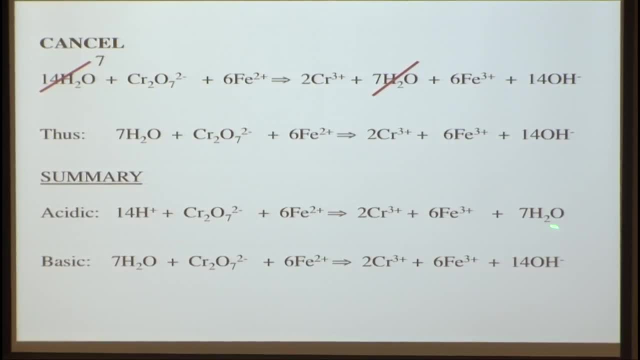 we have 14H-plus on one side and 7 waters on the other. In basic, we have 7 waters on this side and 14OH- on this side. Everything else should be the same and they should all add up. 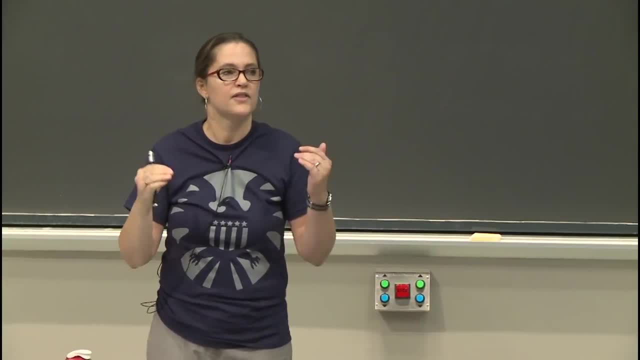 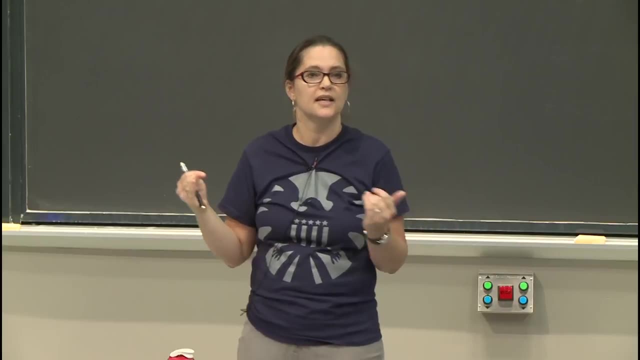 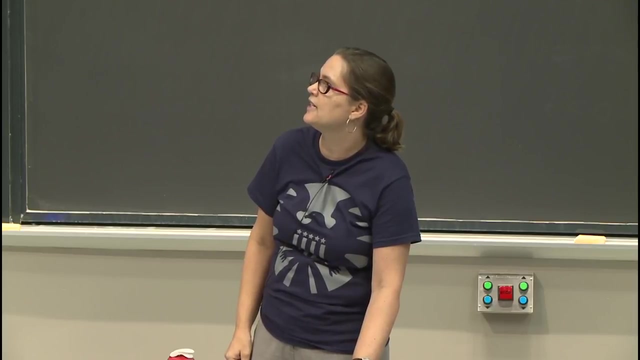 All right, so there we go. That is balancing oxidation reductions. It seems really straightforward, but it's very important. We'll see next week that we need to use this information to be able to do problems. All right, so end of 14.. 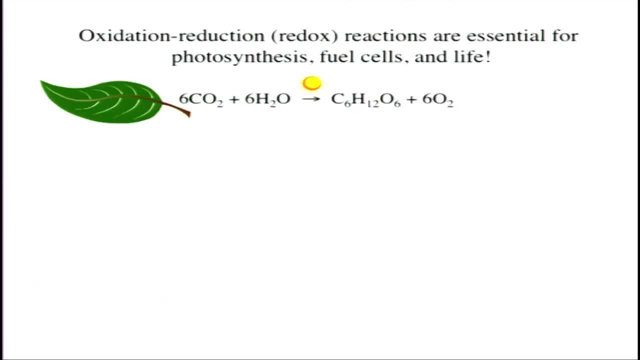 Now to electrochemistry. So today's handout. So we've been talking about oxidation reduction. We're continuing talking about oxidation reduction. I just want to remind you how really important oxidation reduction reactions are. So we've talked about photosynthesis in this class. 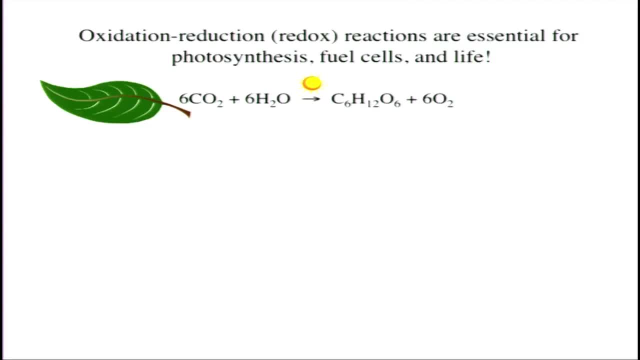 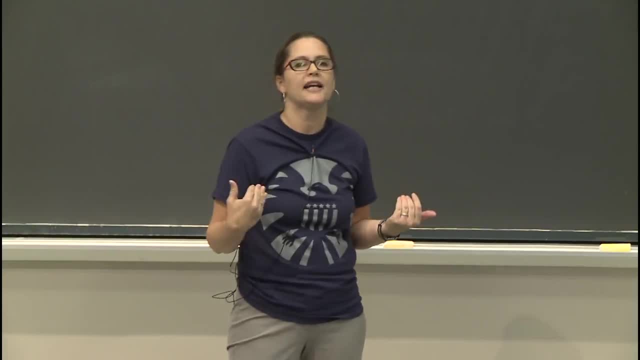 We've talked about fuel cells. All of these reactions that make energy involve oxidation reduction, loss of electrons, gain of electrons. Basically, the human body is a big battery. We have lots of oxidation reduction reactions going on inside of us. This is how we live. 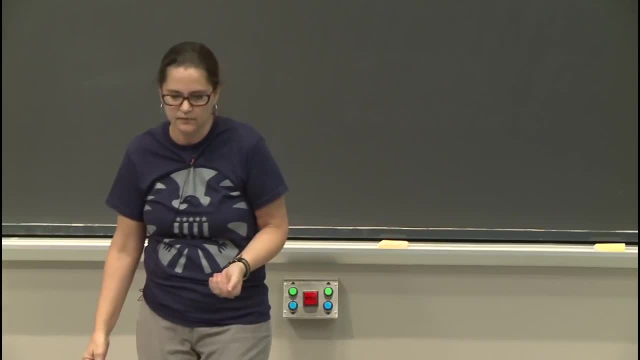 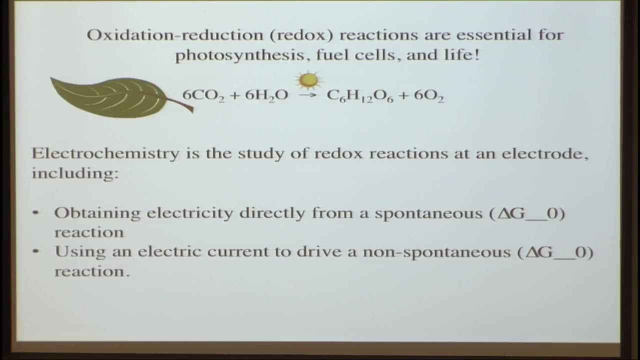 This is how we make energy, This is how we survive, All right. so electrochemistry is the study of redox reactions, usually thinking about how they occur at an electrode. So there are two types of reactions that you will be considering. You might be considering: 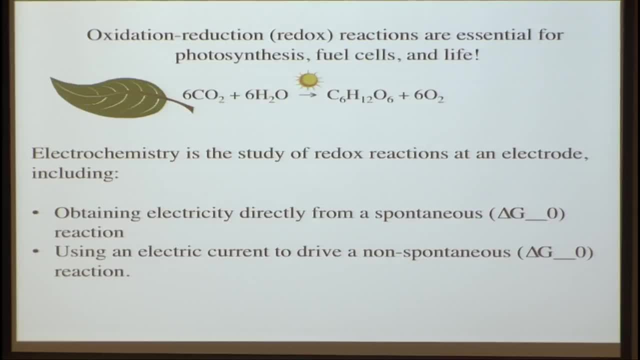 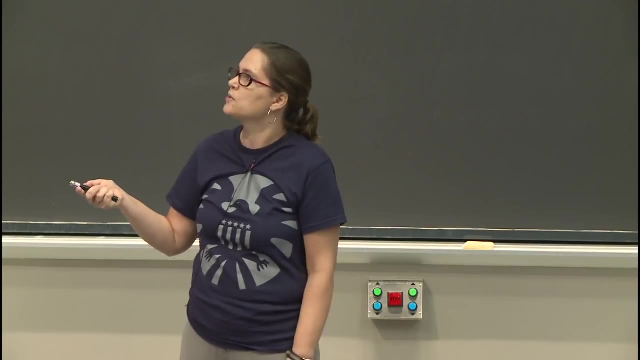 a reaction that generates an electric current, electron flow or electricity from a spontaneous reaction, And you might consider one where you need to drive a reaction that is non-spontaneous using an electric current. So a spontaneous reaction. delta G is what. 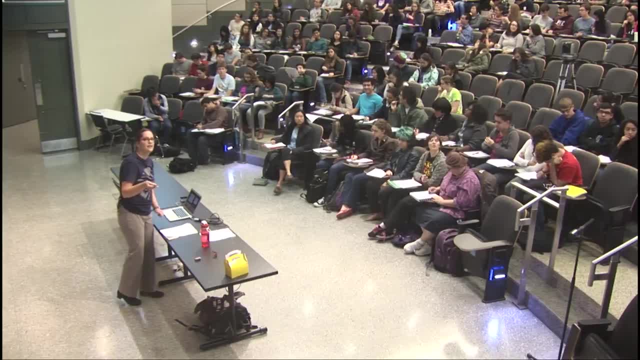 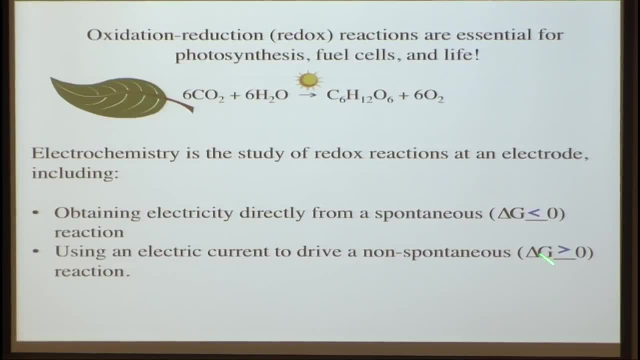 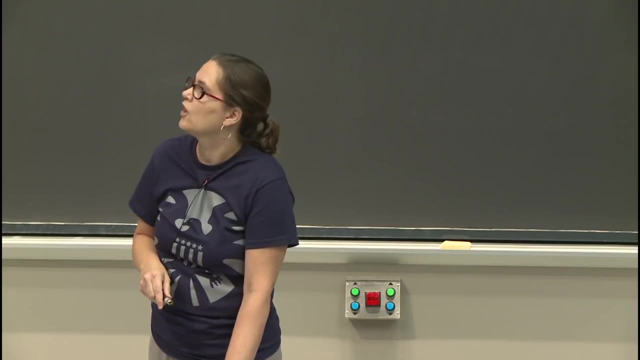 Positive or negative. Right So spontaneous reaction: delta G is negative, It's less than zero. A non-spontaneous reaction is positive. Just a little review there for exam three, All right So electrochemistry study of these redox reactions. 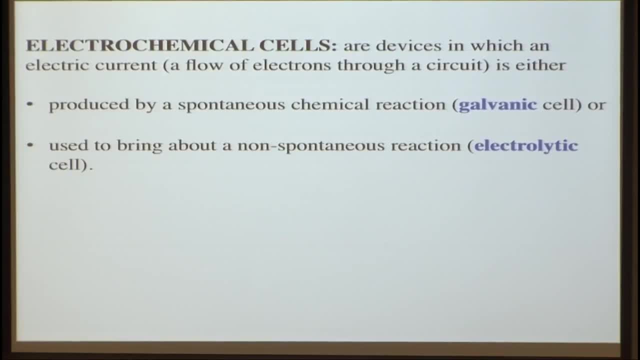 Electrochemical cells are devices where you generate electrons and they flow through the cell And so you have the flow of electrons through a circuit And again, that can be generated by a spontaneous reaction And if it is generated by a spontaneous reaction that's called a galvanic cell. 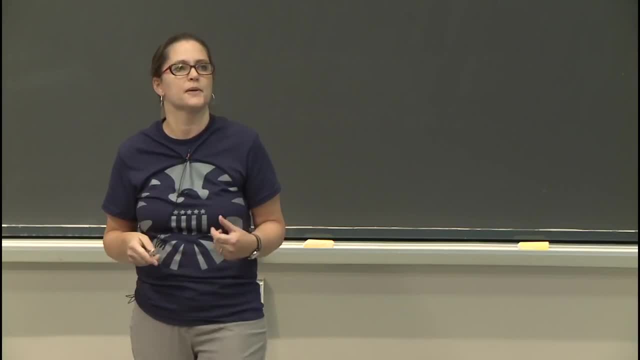 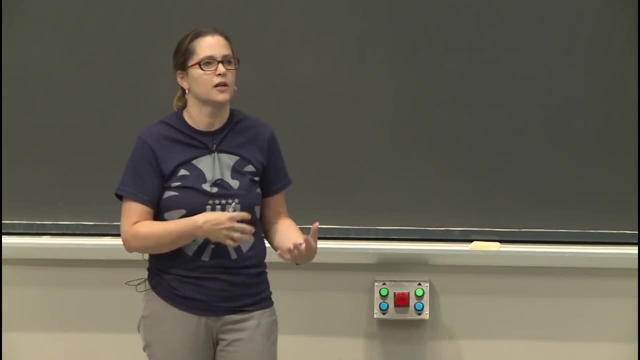 Or you can use an electric current to force a non-spontaneous reaction to go and that's called an electrolytic cell. And it's important to remember those definitions because a lot of problems tell you: oh, in this electrolytic cell. 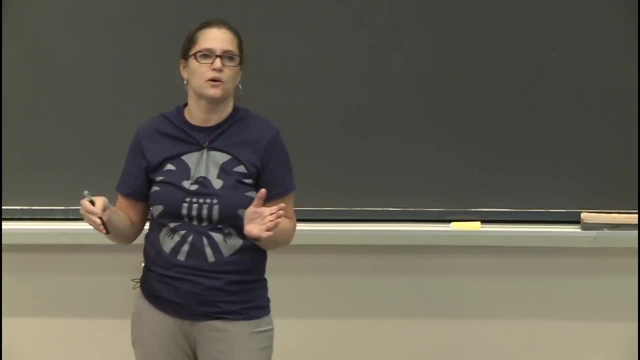 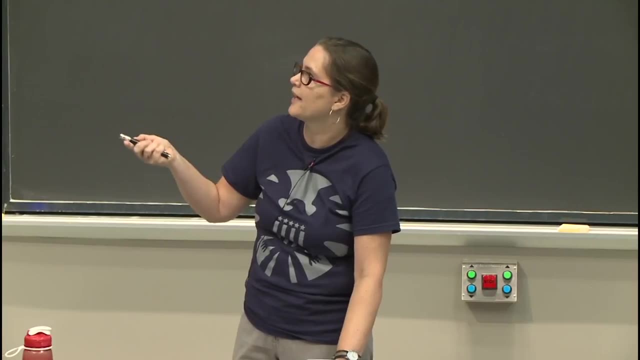 and without that's telling you key information about what's going on in that problem. So if you don't have these committed to memories, you will find yourself in trouble. But it's not too bad, It's just two terms, All right. 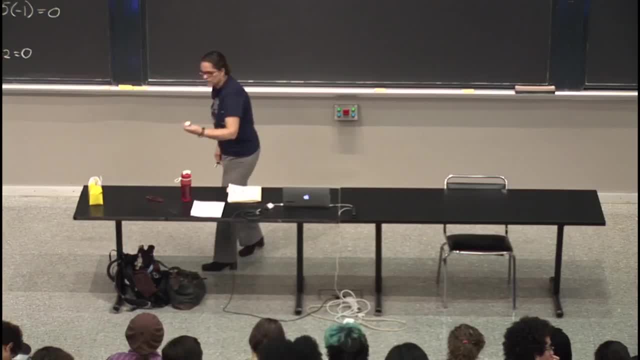 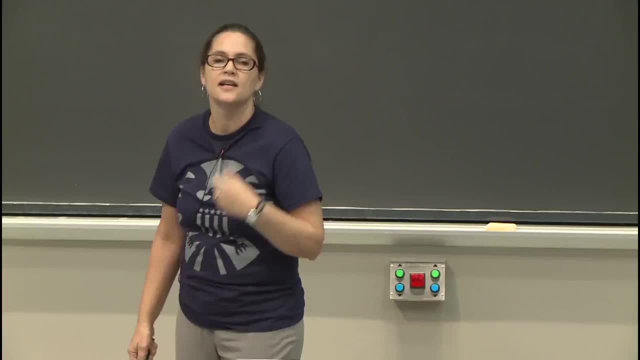 So a battery then? So I have a battery here. A battery is a collection of galvanic cells And it's going to give us, it's going to use spontaneous reactions to give us an electric current. All right, And again electrodes. 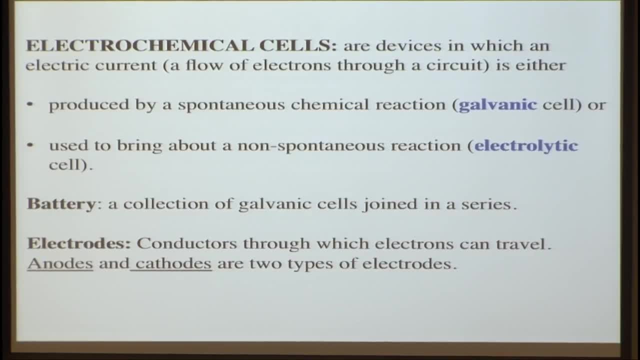 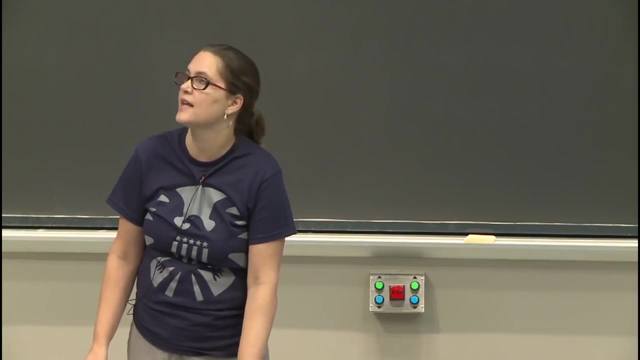 the definition for those. they're just the conductors through which the electrons travel, And there are two types. Let's quiet down again. I hear the noise. Two types of electrodes: We have anodes and cathodes, All right, So let's look at an electrochemical cell. 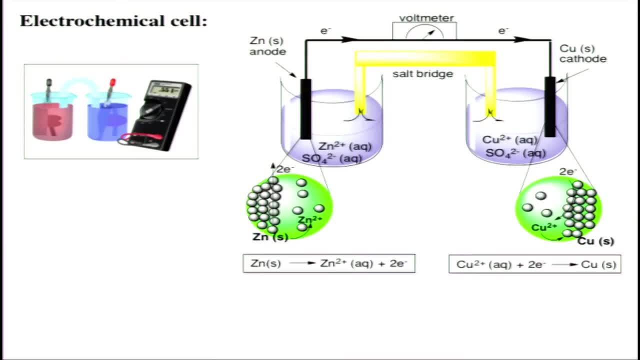 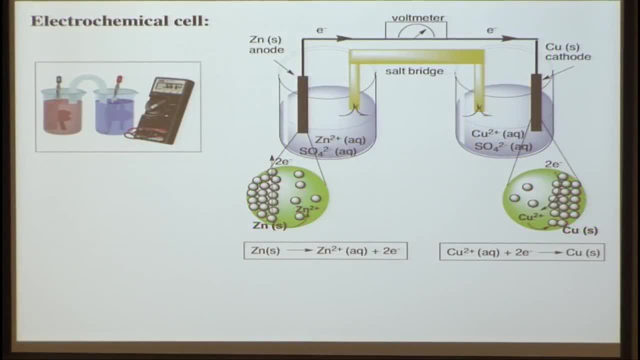 and consider again the anodes and the cathodes. So this is my beautiful depiction of an electrochemical cell. This might be a better depiction of what it looks like, but I think mine is not bad, Just to help you out. 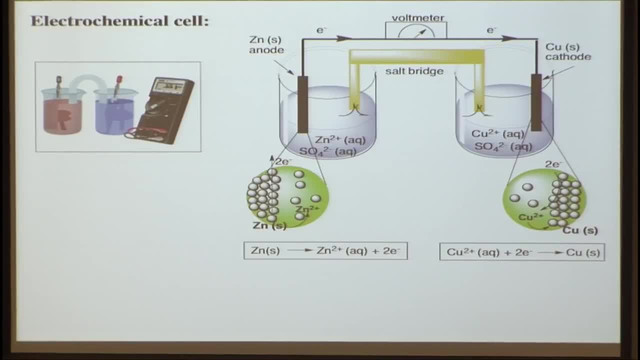 that's supposed to be a beaker that has fluid in it. This is also a beaker that has fluid in it And this is my electron. This is my electrode. that is an anode in this case. There is the anode there. 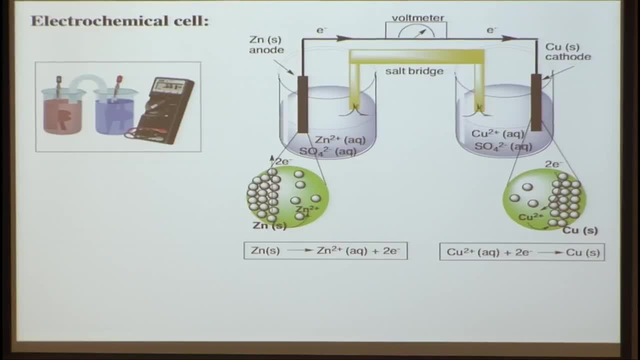 or the electrode there. Here's another one, That's the cathode, another type of electrode. It's over here. This is my salt bridge, The salt bridge here is this plastic tube And here I have a wire connecting my electrodes. 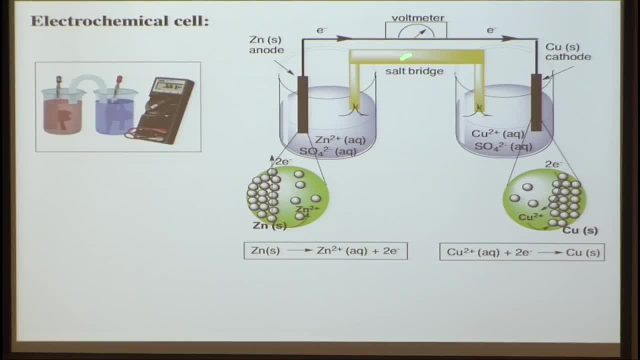 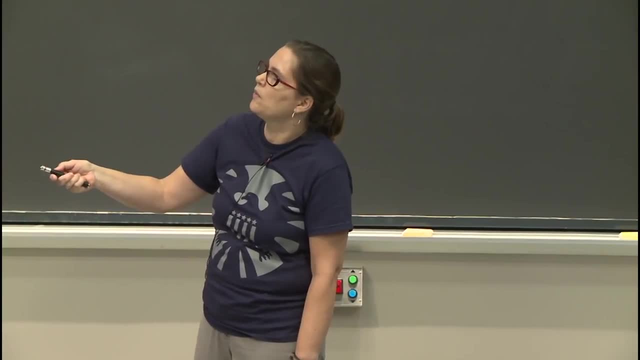 Here you can't really see the wire, but in both cases it goes through some kind of voltmeter that measures the electric current. All right, So now we'll get rid of this better picture, but you can think about this picture as that picture, if that helps. 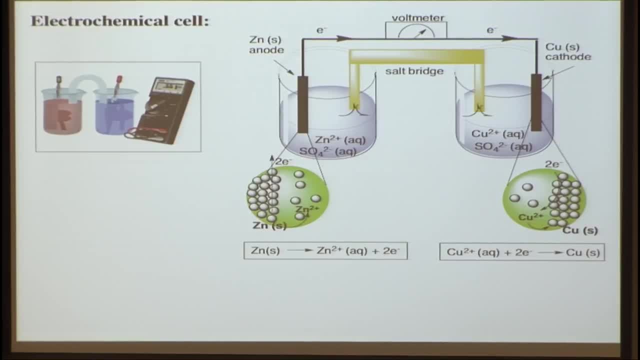 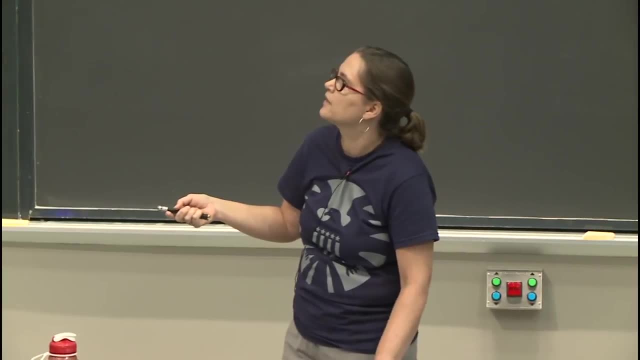 And I always like to joke that you think you have it bad here at MIT. in the old days, Before you could do your problem set at 2 o'clock in the morning, you had to build your own batteries to be able to do it. 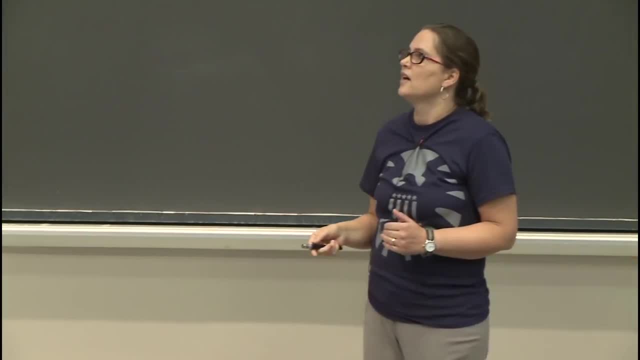 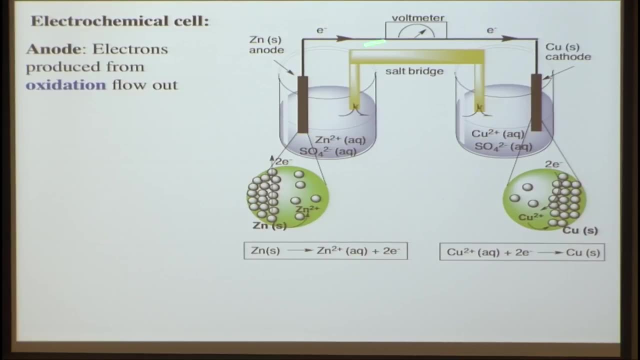 All right. So anode Electrons are produced from oxidation at the anode. So the electrons produced here flow out of the cell, And in this particular type of electrochemical cell, zinc solid is oxidized to zinc plus 2.. So if we look at this over here, 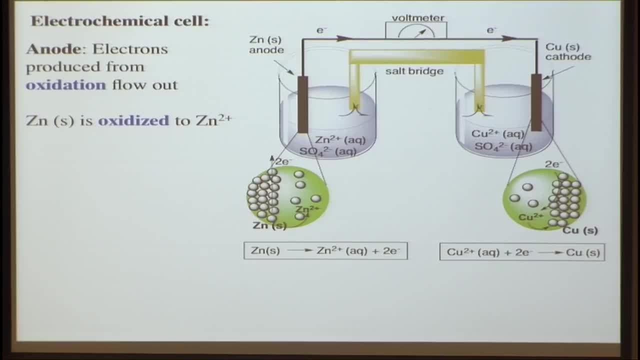 this is my little beautiful depiction of the blowup of the electrode. We have our zinc solid here and we have zinc plus 2 in aqueous solution. So when the electrons leave the zinc solid, so that the zinc then leaves the electrode and goes. 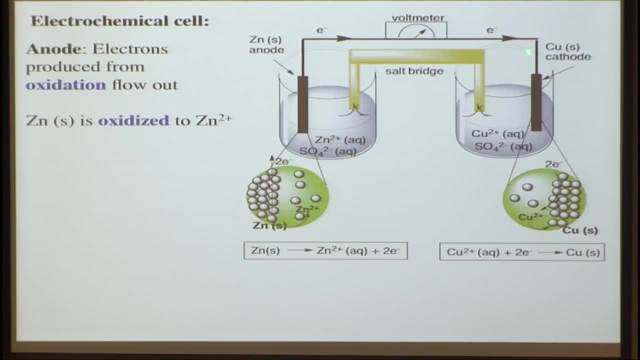 into solution forming zinc plus 2, those electrons go out. So the electrons will then go into the cathode And notice I had a typo in the handout. I find this cut pretty funny. I don't know if it's me or spell check right now. 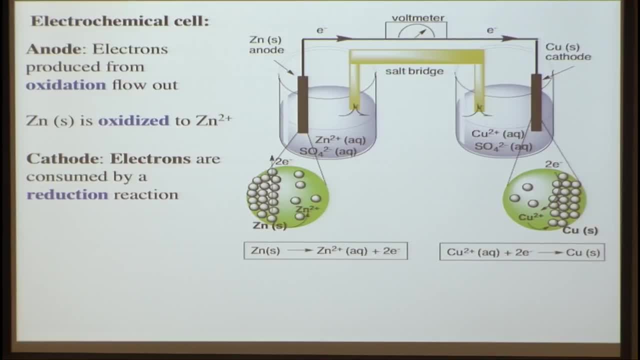 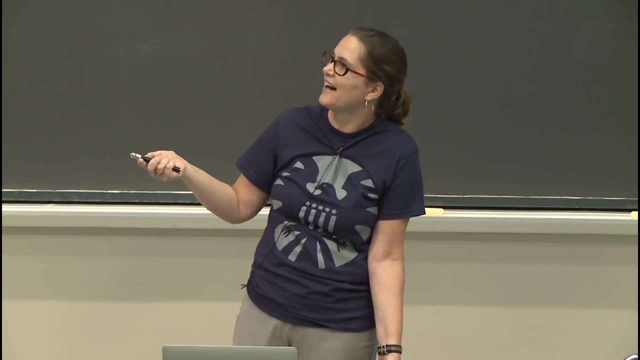 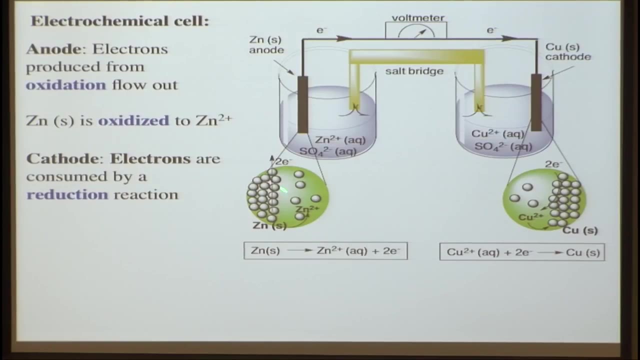 I wrote elections are consumed. Oh man, it's been a long week Between the national elections and our T-shirt elections. Anyway, I didn't mean elections, I meant electrons. Yes, of course, Electrons. Electrons are consumed. 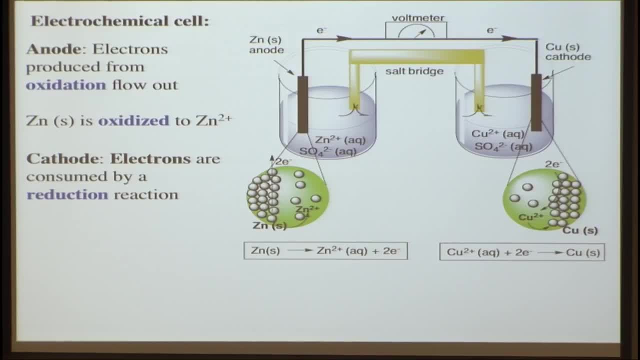 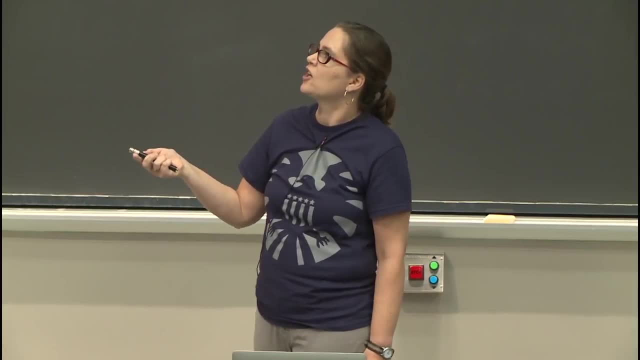 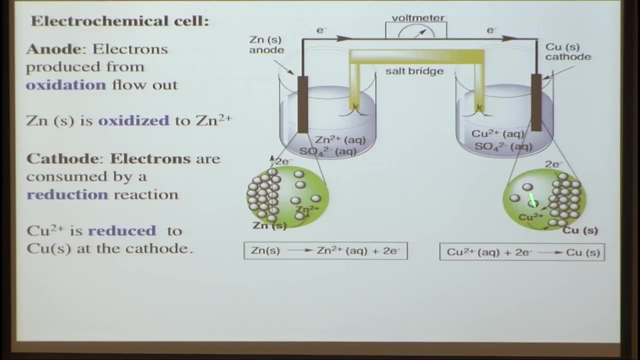 by a reduction reaction, Of course. I noticed that after I had printed hundreds of copies. OK, And this particular reaction: here copper plus 2 is reduced to copper solid And if we look over here we have copper plus 2 in aqueous solution. 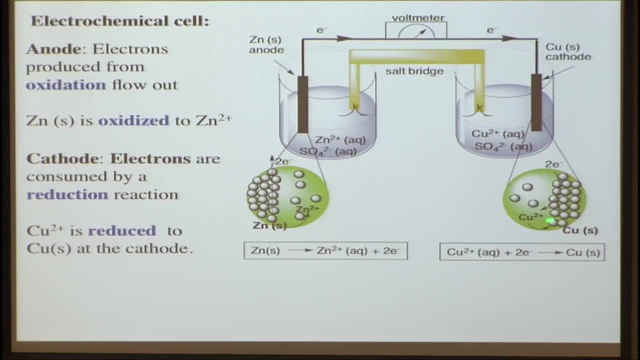 When electrons- two electrons- come in, those two electrons go to the copper plus 2 and reduce it to copper solid And the copper solid actually plates on the electrode. So we can measure the flow. We can have a meter that measures the bolts. 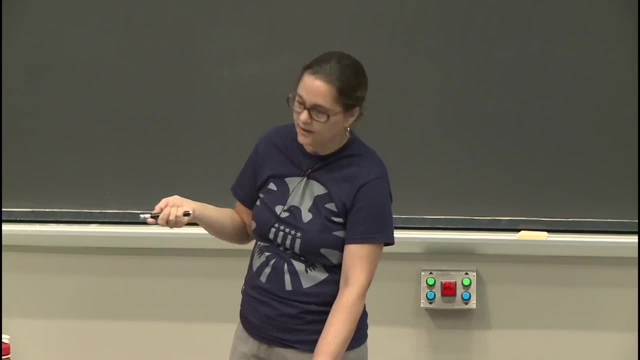 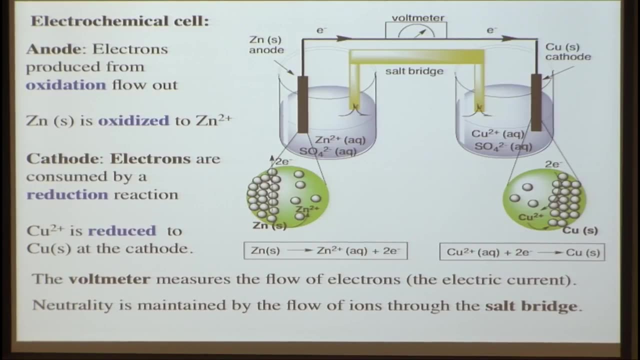 or the flow of electrons, the electron current, And also what's that salt bridge doing? Well, the salt bridge can help maintain the neutrality in the system, because over here we're generating plus charge And over here we're losing plus charge. 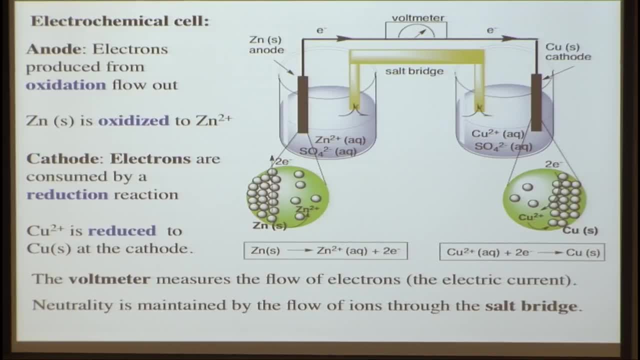 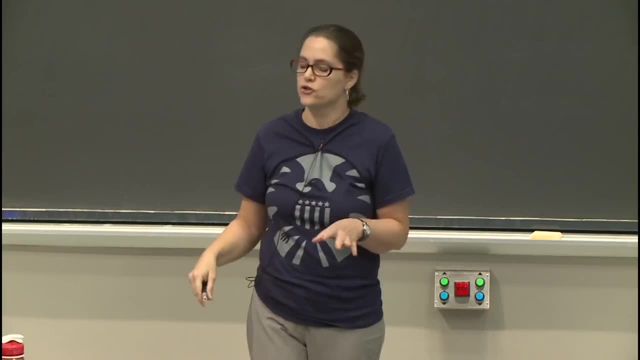 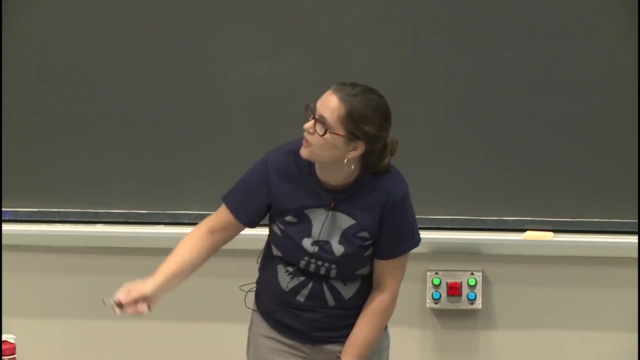 And so ions can flow through the salt bridge and keep the charges more similar in our two different beakers. All right, So I know my pictures are gorgeous, but I have a little animation to show you that will also show you what I was talking about. 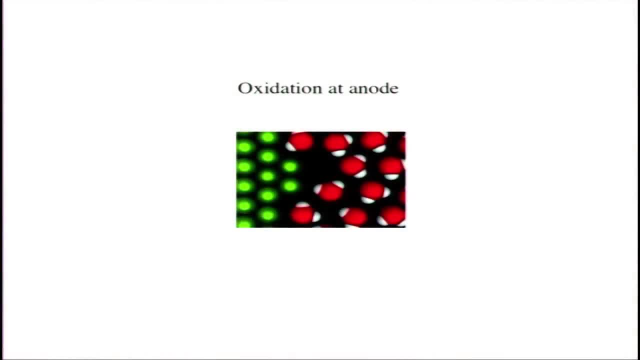 oxidation at the electrode. So zinc solid is going to lose electrons and form zinc plus 2.. And let me just show you that happening. So there are the electrons going away And here is zinc popping off as zinc plus 2.. And then the zinc plus 2. 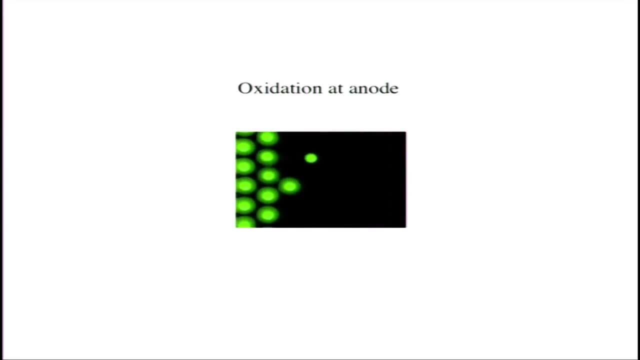 is going to be in solution. So there, the electrons go again And the zinc solid pops off as zinc plus 2.. All right, So now let's consider reduction at the cathode. So here we have our copper solid, Here we have a copper plus 2.. 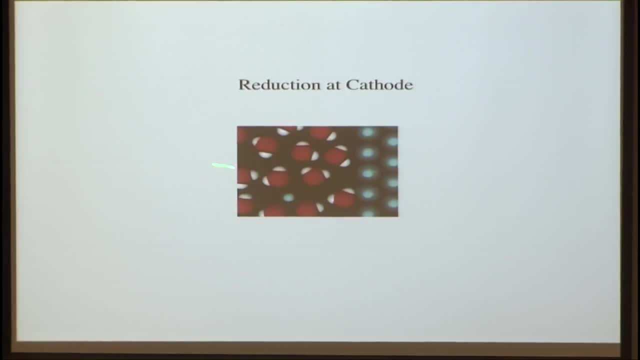 And here the electrons are going to come in and join up with our copper plus 2.. And it's going to plate on to the electrode. There come the electrons, There they come again. And now we have added solid copper to our electrode. 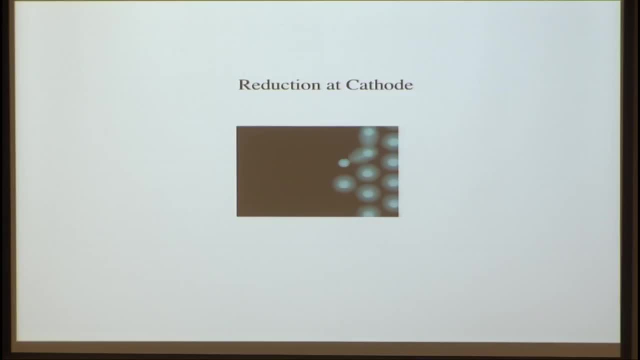 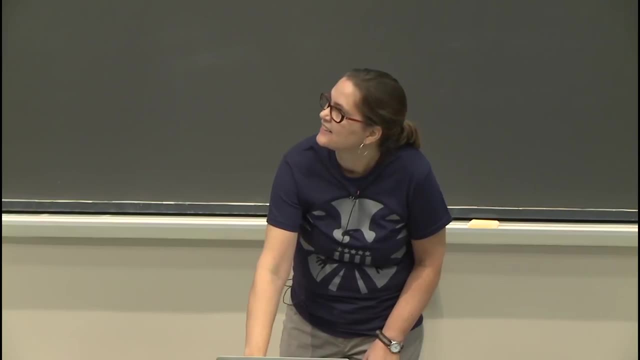 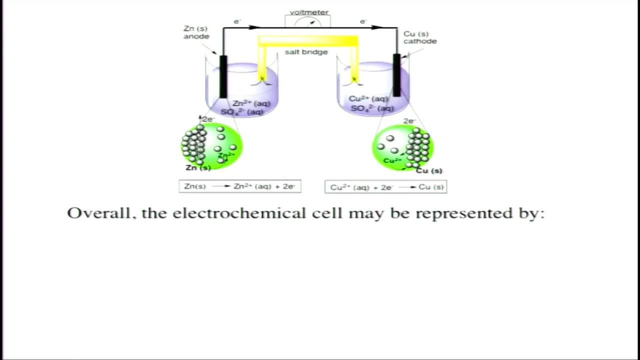 And just one more time. And I think it's so cool that we can just watch those electrons move like that. Okay, All right. So there's our electrochemical cell, Where we have an oxidation and a reduction reaction. Instead of drawing this, 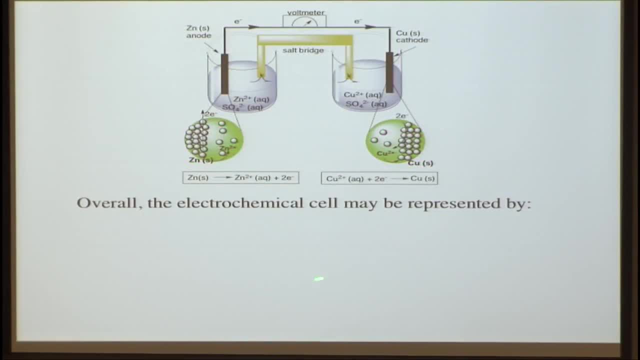 admittedly, beautiful picture. every time we can have a shorthand representation for this. So we can say: zinc, solid, And then we have a little line here. That little line indicates we have a phase boundary. So that means we're going from solid to a different phase. 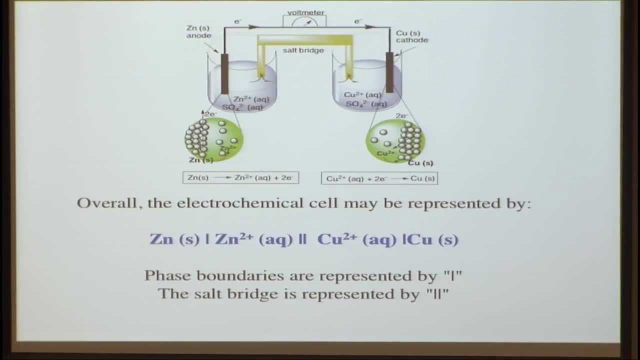 And in this case we're going to aqueous, So solid zinc to zinc plus 2. The two lines here indicate the salt bridge. So this tells us that the reaction on this side is in one beaker and the reaction on this side is in our other beaker. 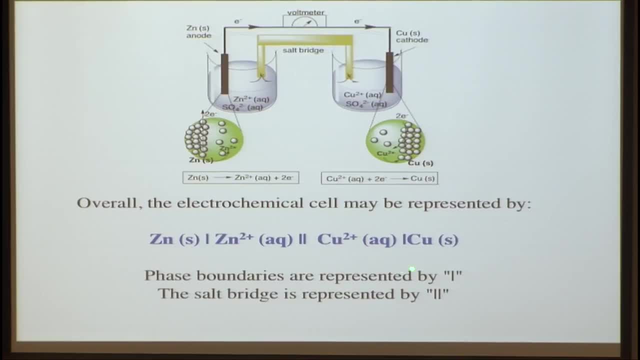 The reaction in the other side is: copper plus 2 aqueous, A single line for phase boundary going to copper solid. Now if we had, say, two aqueous species, we wouldn't have a phase boundary, We'd just have a comma. 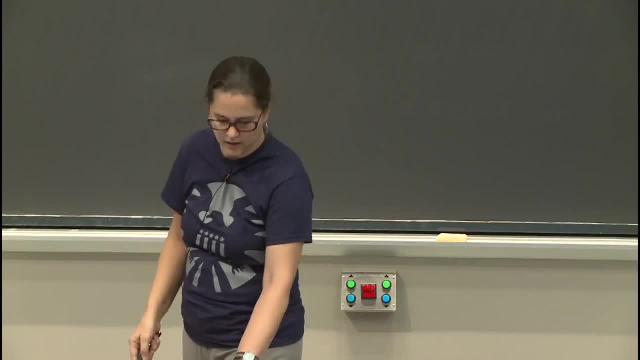 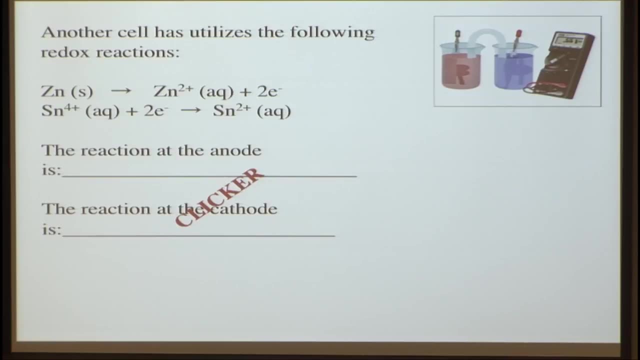 But if you have a phase boundary, you get the line All right. So it's a clicker competition. Let's consider another cell. It still has zinc, but now it has tin. Why don't you tell me which reaction is at the anode? 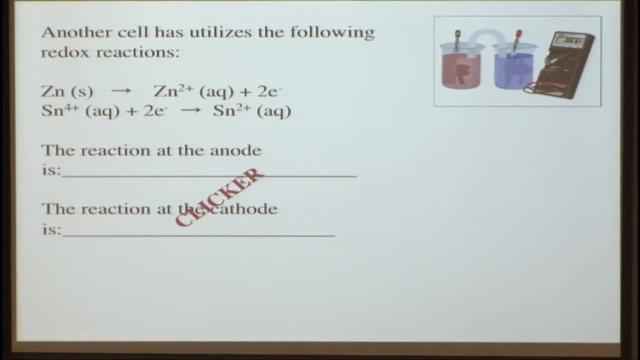 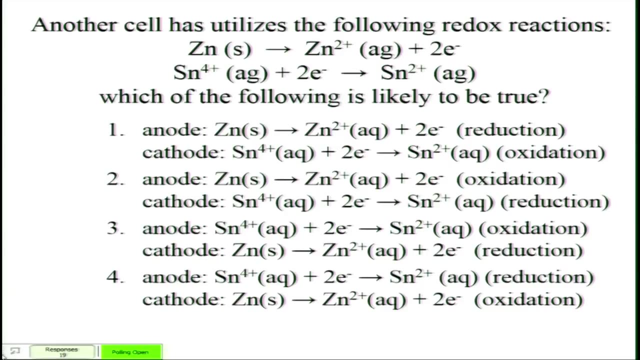 and which reaction is at the cathode, And also which of those is oxidations and which is reductions. All right, We'll just do 10 more seconds. Great Okay. So some of these had parts of it, right, but there was a mistake. 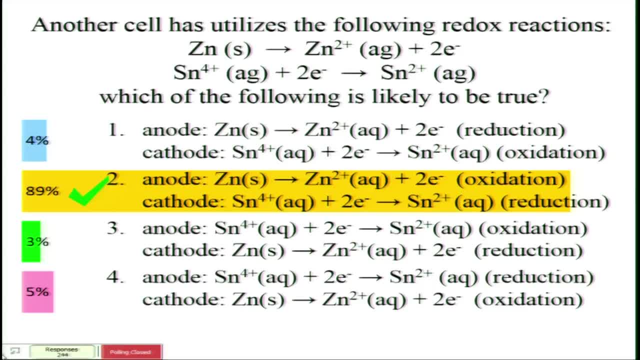 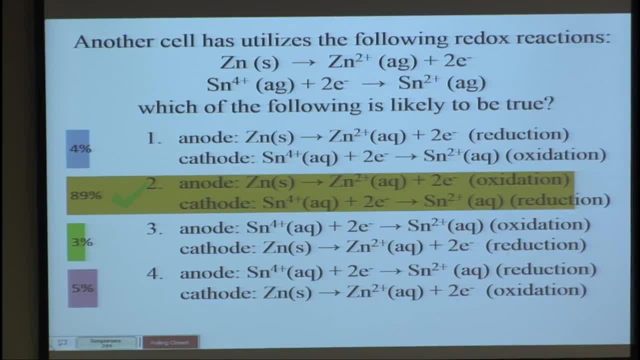 We have an ox, so that is wrong. So you have to pay attention to whether these match and then also that the reaction is written consistent with the words. So only number two had all the various different parts. right, Okay, So we can come back here. 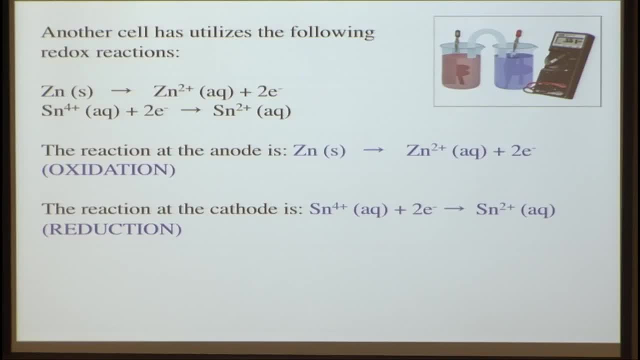 and you can enter. So the reaction at the anode was the zinc reaction and that is an oxidation and ox. The reaction at the cathode is the tin reaction: tin plus four, two electrons. tin plus two aqueous and that's a reduction. 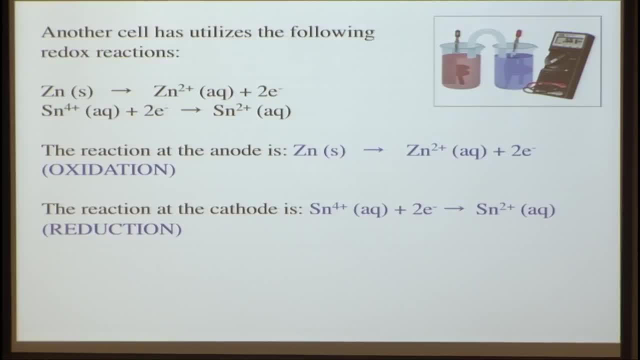 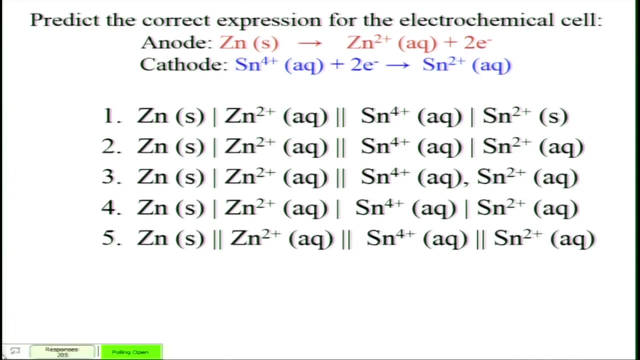 And while you have your clickers out, why don't you tell me how you would represent that electrochemical cell? All right, Let's just do 10 more seconds, So right. So I mentioned this very briefly. This was my tricky clicker question. 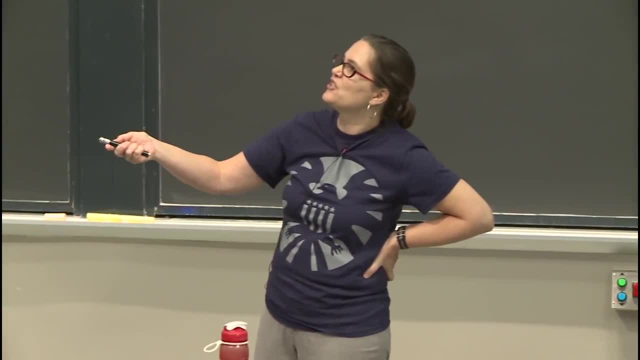 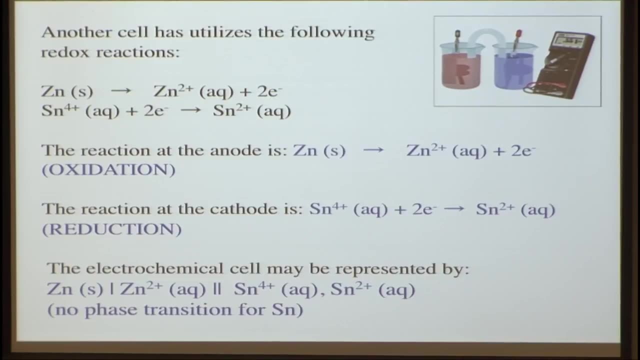 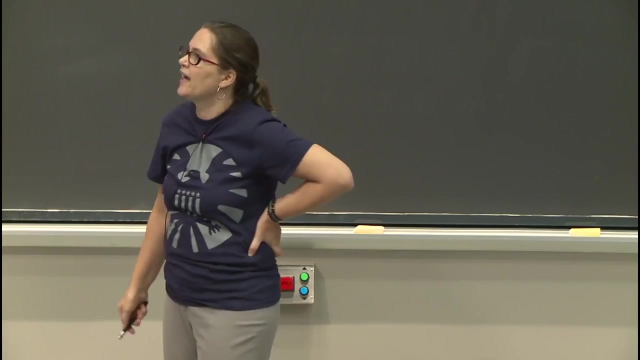 because it's a competition. So there's no phase transition here. so you have a comma And the top one a few people put down but it's not solid here, so that one is not correct. Okay, So here you can write down. 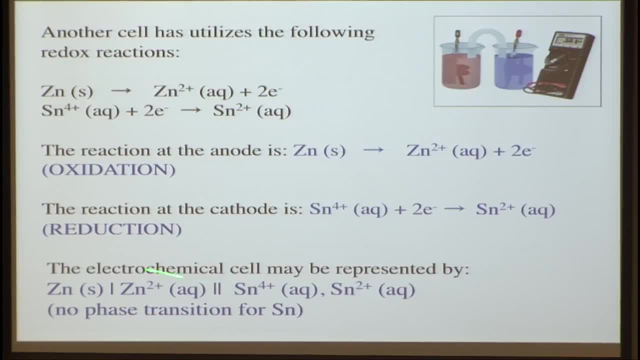 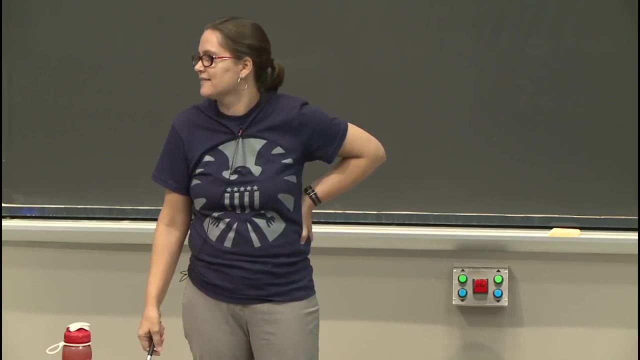 in your notes. you have the zinc phase transition: zinc plus two- aqueous, and then we have our salt bridge: zinc plus four- aqueous, comma, or zinc tin plus four comma, tin plus two. And now we're ready for winners. 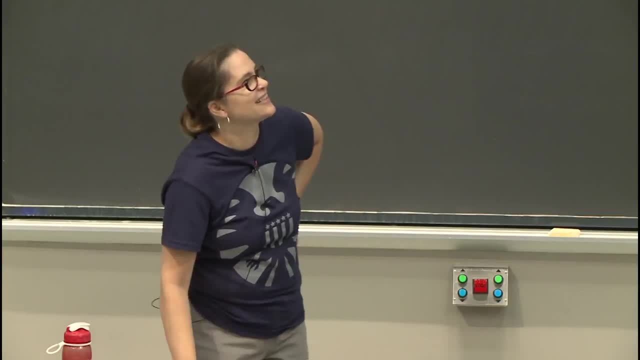 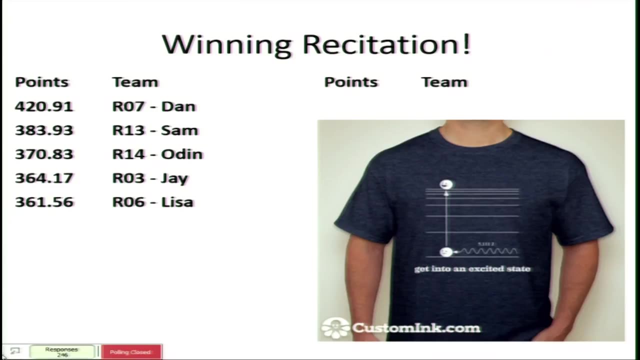 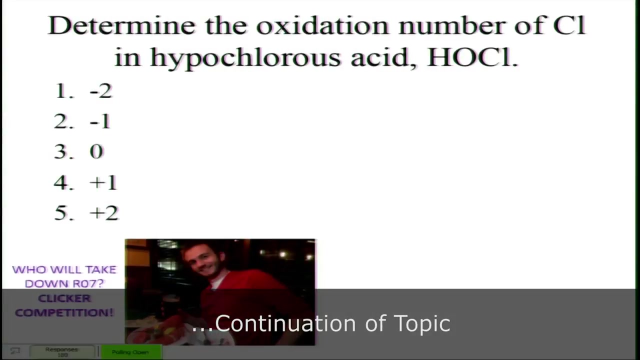 Let's see if Sam's also ready to present the winners. All right, We need a strategy to defeat Dan's recitation, but we know what T-shirt we're playing for now. All right, Have a great weekend everybody. All right. 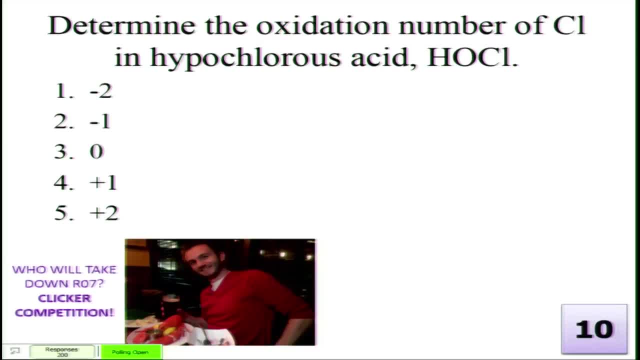 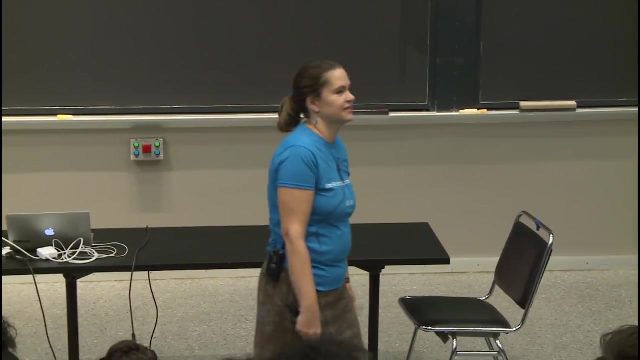 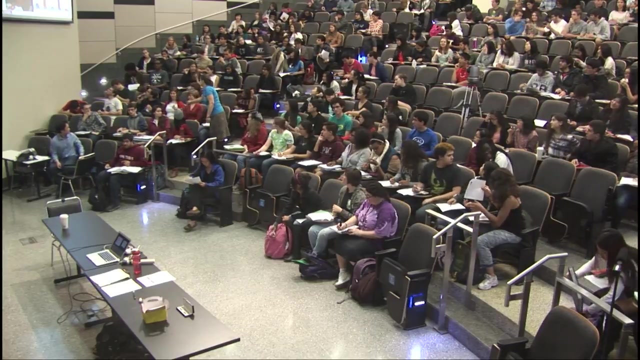 Let's just take 10 more seconds, All right, All right. Does someone want to tell me how they got the right answer? Yep, You know that your hydrogen will have a plus one charge and your oxygen will have a minus two charge. 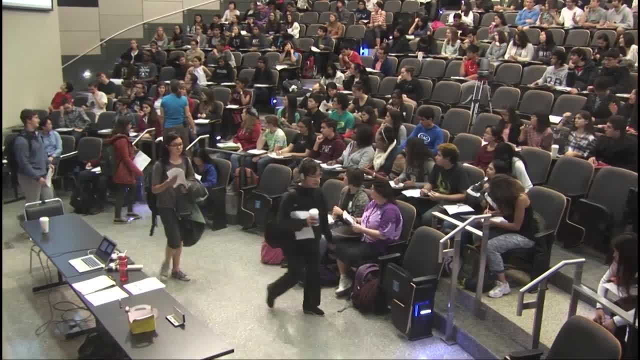 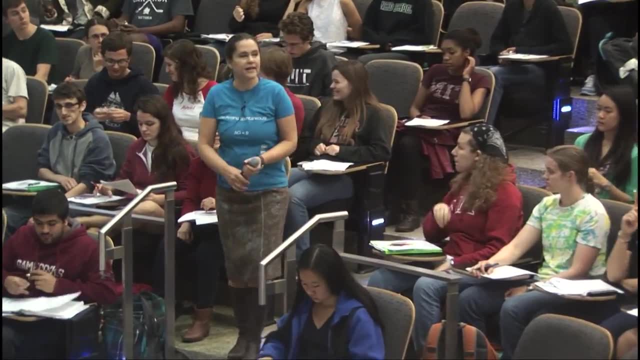 because it's not a peroxide and you know your sum is going to be neutral, so you add one. Yep, That's right. So this one. chlorine is usually minus one. The exception is when it's with oxygen, and so oxygen is always minus two. 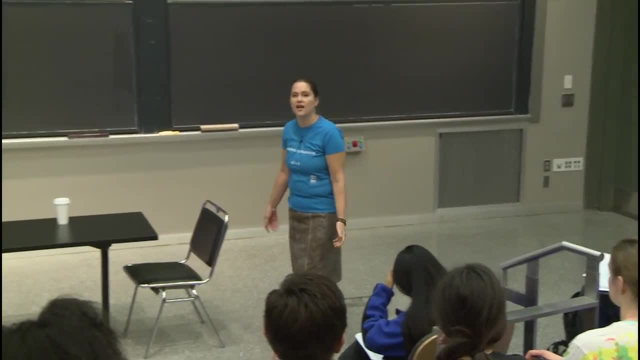 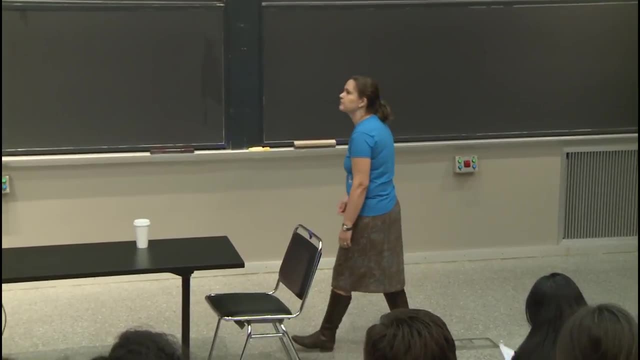 unless it's in a peroxide or superoxide, and hydrogen's always plus one, except when it's with a metal like sodium, something group one or group two. OK, So today take out lecture 25 notes. We're just going to wrap. 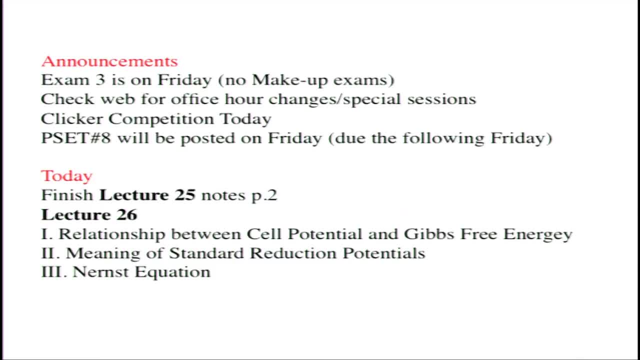 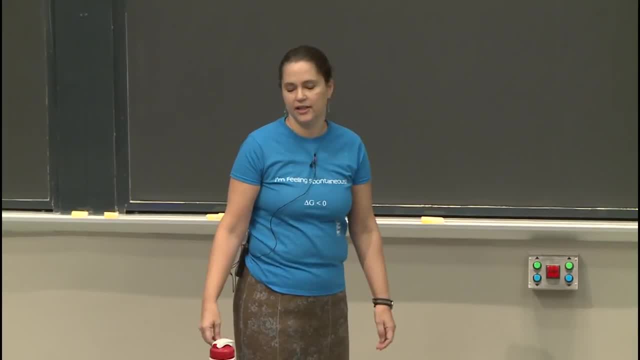 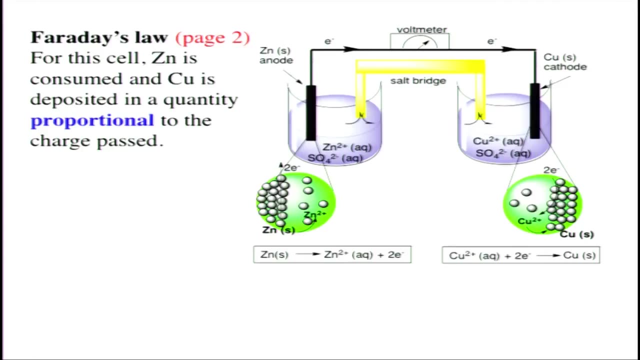 those notes up, That shouldn't take too long, and then keep going with lecture 26.. So we were talking about this cell and we're going to talk about this electrochemical cell a lot. So we had zinc on one side, zinc at the anode. 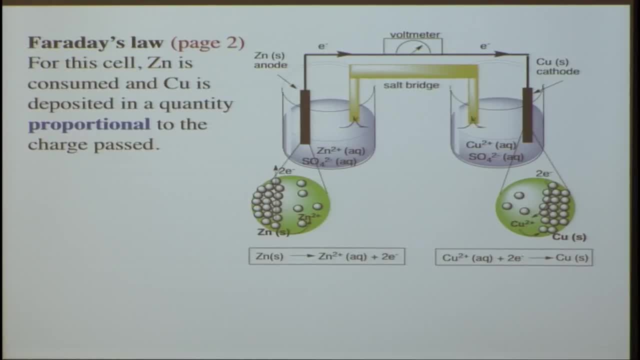 and the zinc was being oxidized, generating electrons which come around to the copper, and then the copper plus two ions were being reduced to copper solid. So the zinc anode was being consumed and the copper cathode had copper solid being plated onto it. 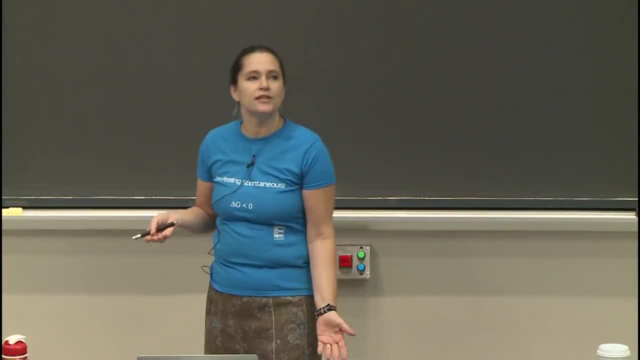 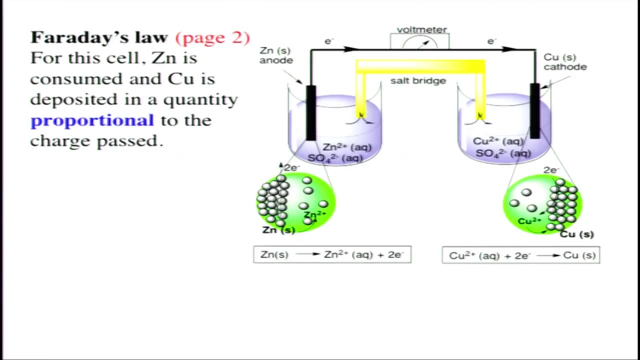 So Faraday's law says that the amount at which an anode like the zinc anode is consumed and the amount of copper that gets plated on at the cathode is proportional to the charge that passes through the system. So according to Faraday's law, 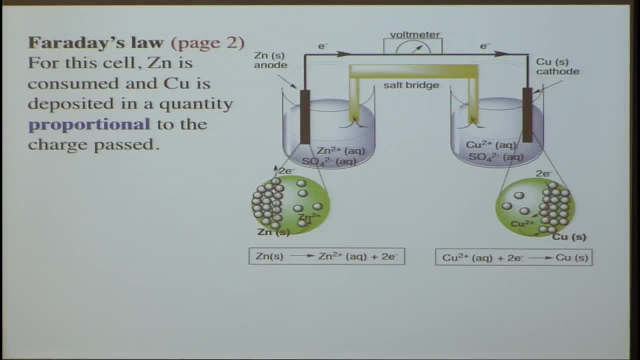 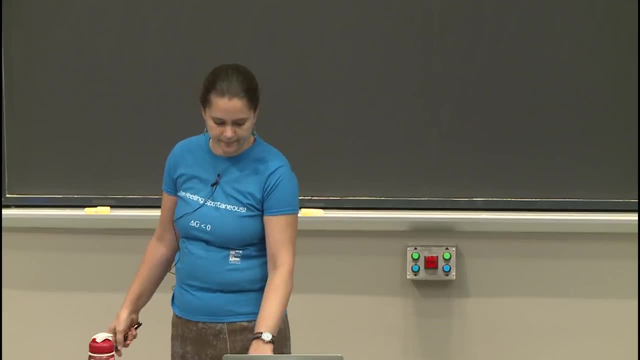 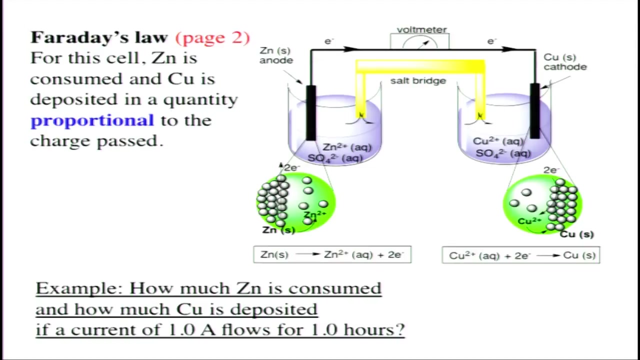 there's a proportionality between the consumption and also depositing of metal and the amount of charge going through the system. So we can think about how much zinc is consumed and how much copper is deposited on its cathode or its electrode, if you have a current. 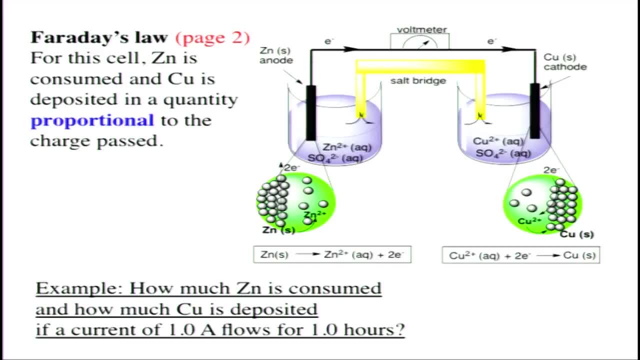 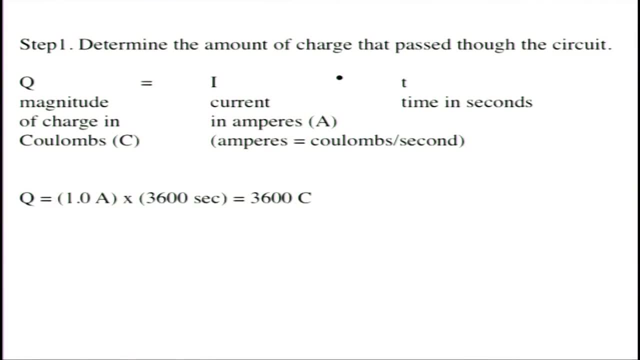 of one amp flowing for one hour. So let's just take a look at how we do a problem like this. First step is we want to think about calculate the charge that's going through the system, And so Q. here we have another Q. 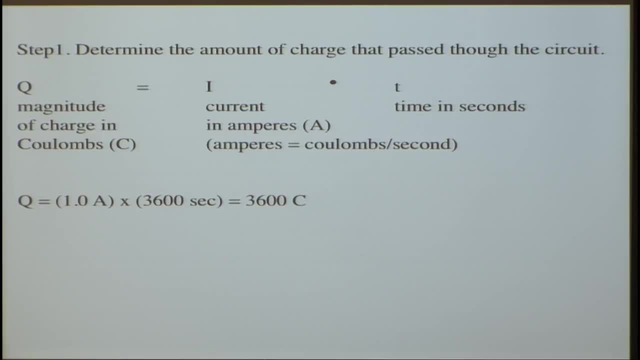 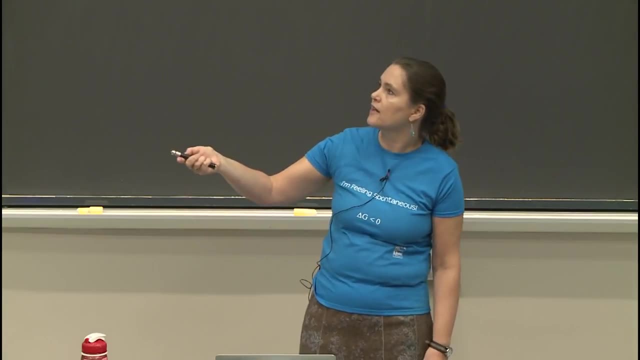 not the reaction quotient but the magnitude of the charge, and that's in coulombs and that's going to be equal to the current times, the time. So we have the current I and the current is in amps and T is in seconds. 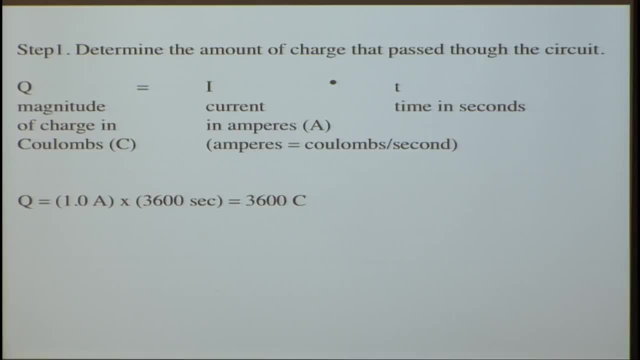 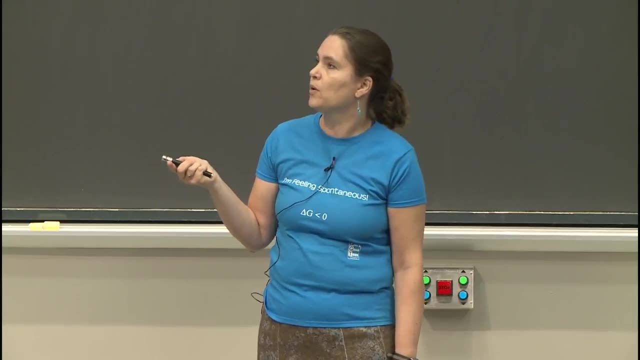 and conveniently, amps equal coulombs. So this equation works out. our units will work out. So Q is going to be equal to. we have 1.0 amps and it was one hour, so that's 3,600 seconds. 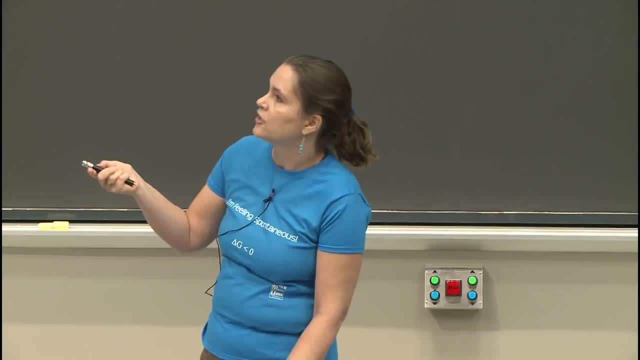 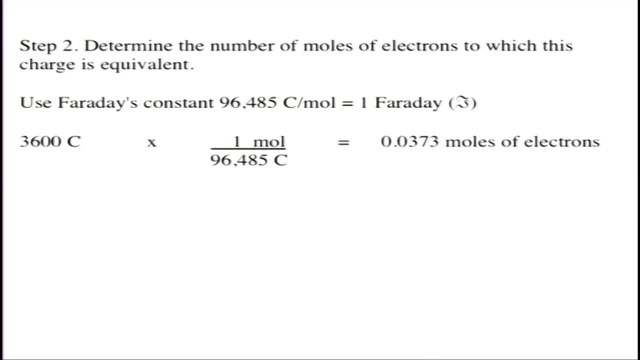 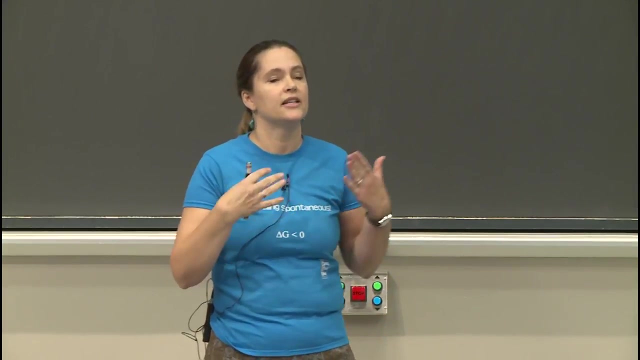 or 3,600 coulombs, because we have an amp times second. And then here we have this number of coulombs and now we want to convert to the number of moles of electrons that that is equivalent to that, that charge in coulombs. 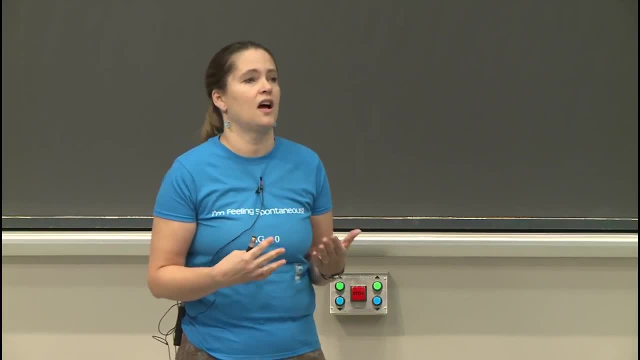 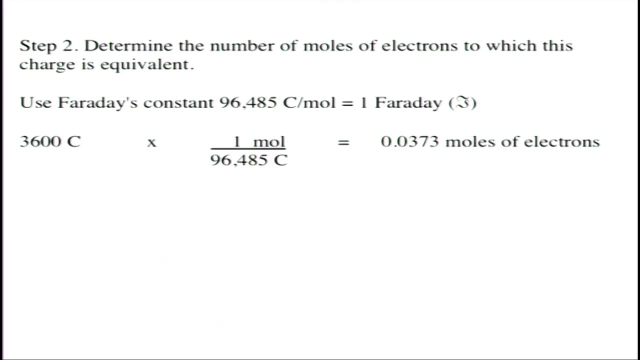 is equivalent to: And here our Faraday's constant is our conversion factor. So Faraday's constant- we have 96,485 coulombs per mole- is one Faraday, and it's this kind of funny-looking F over here. 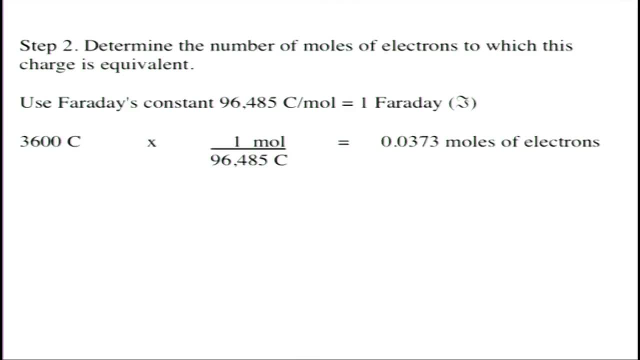 So we have our coulombs, so we can use now the Faraday's constant to convert and we get 0.03, 0.073 moles of electrons. So that's the number of moles of electrons that would be going through our system. 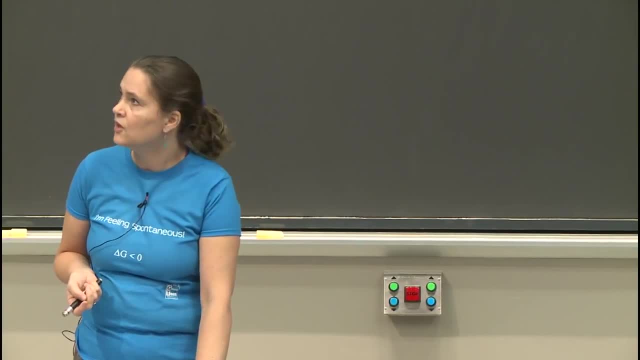 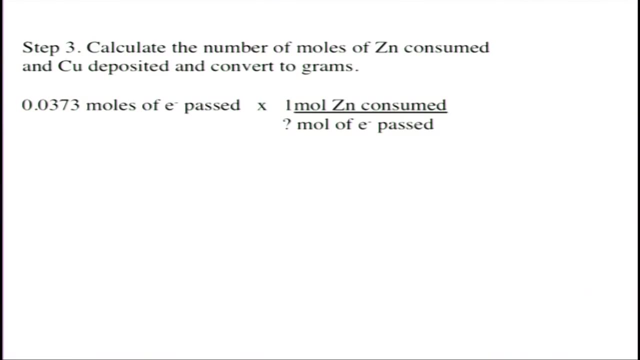 that correspond to that amount of charge. All right, so now we need to relate this back to the zinc and the copper. So step three: we want to know first the number of moles of the zinc and copper involved and then convert that to grams. 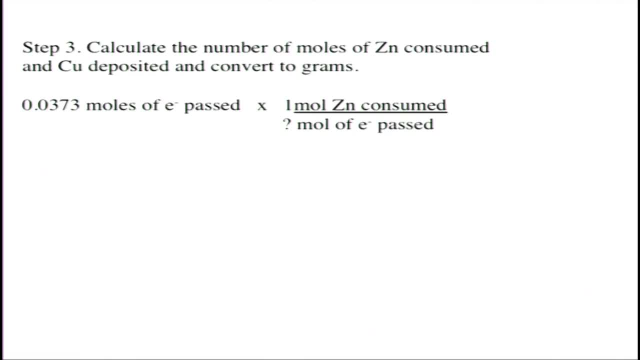 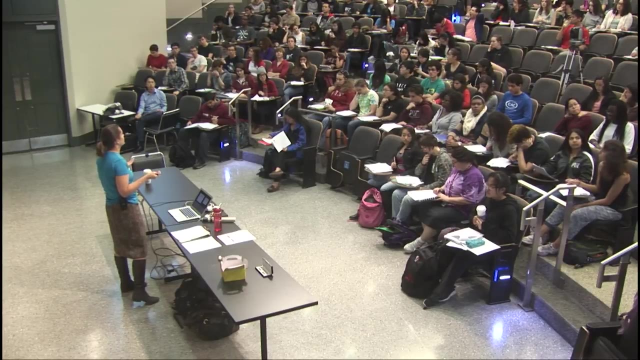 because the problem asks us for grams. So we have the number of moles of electrons that are going through the system. so for every one mole of zinc consumed, how many electrons go into the system? What's the ratio One- two, how many electrons? 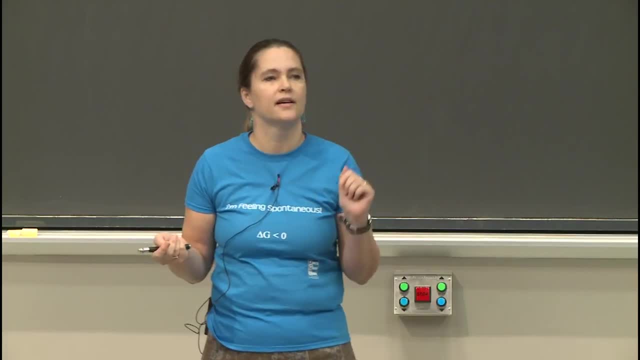 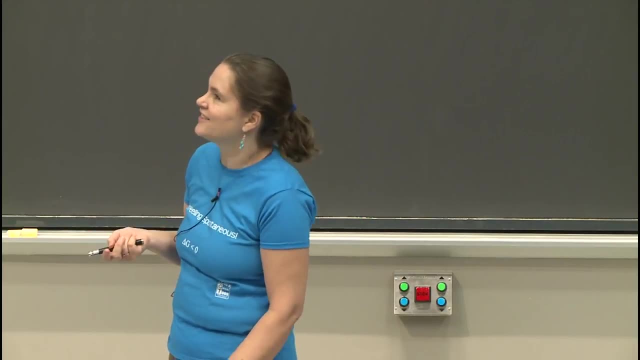 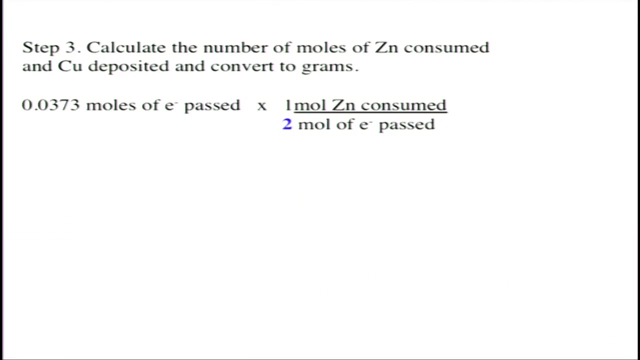 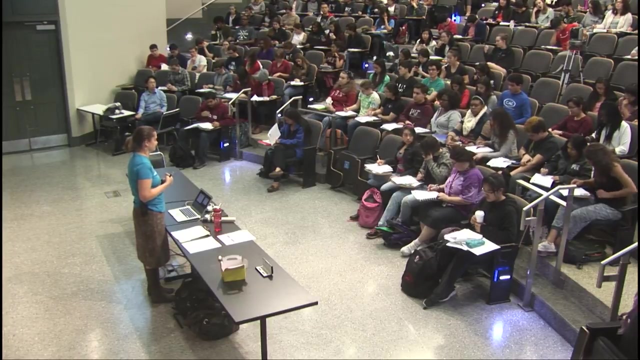 So one zinc solid going to one zinc plus Two, Two, So that's going to be two moles of electrons. And then we need to look up how are we going to convert our moles to grams? What are we looking up? 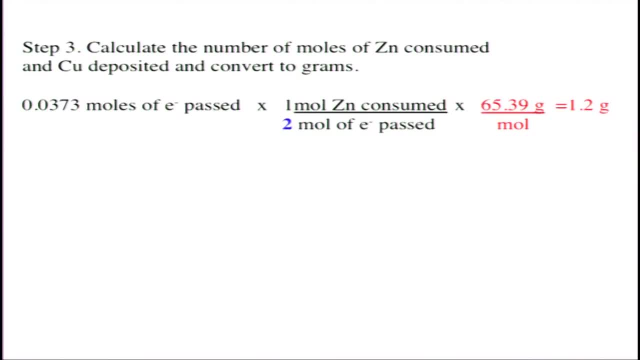 Yep: Molar mass, molecular weight, atomic mass. So in our periodic table grams per mole, and so we get 1.2 grams here for this equation. All right, so for copper. so we have the same number of moles of electrons. 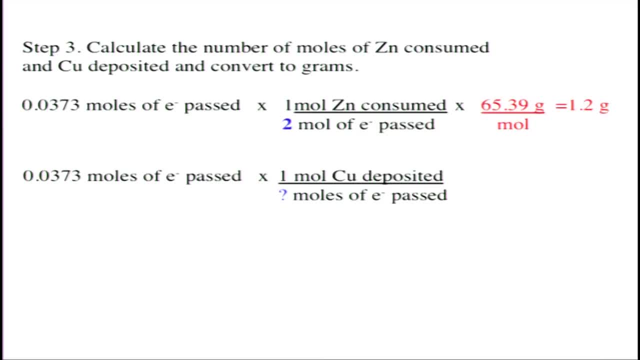 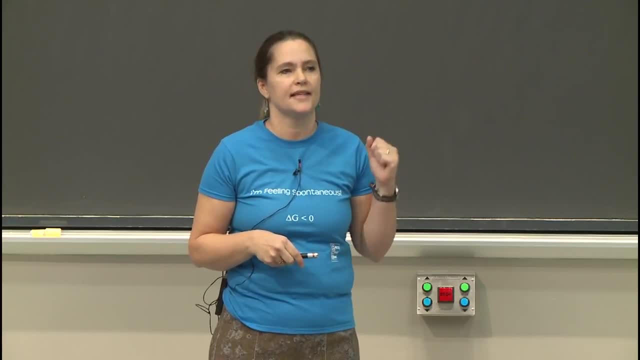 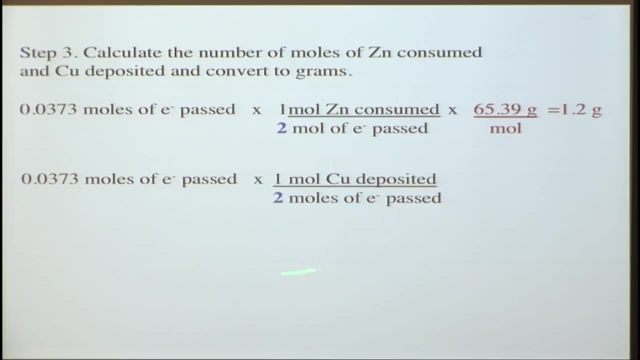 that are going through the system. so for every one mole of copper solid deposited on its electrode, how many moles of electrons have to come into the system Louder? Two, Two, yes, So that's two as well. And then we look up again. 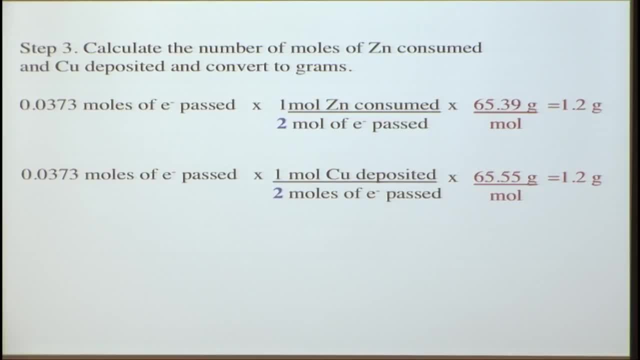 in the periodic table, the atomic weight, molecular weight, and it's almost the same copper and zinc. So to the number of significant figures, it's the same amount of grams. Now, this will not always be the case, They're just very close to each other. 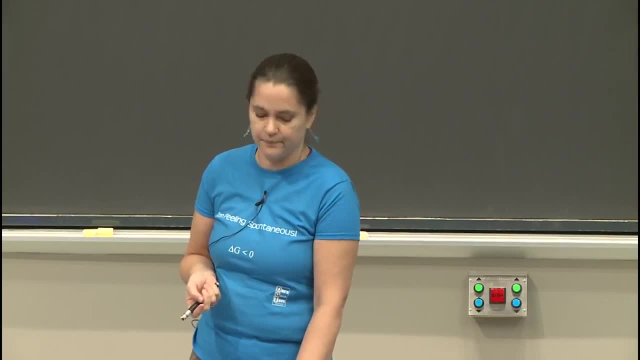 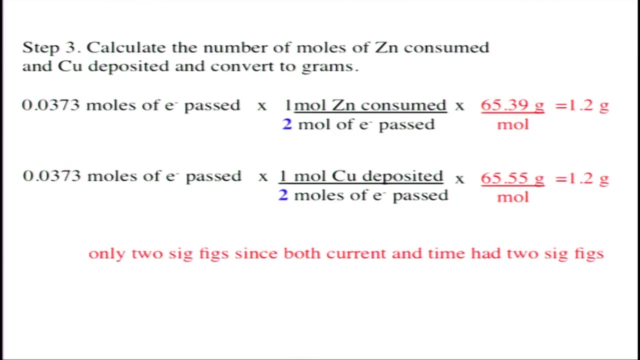 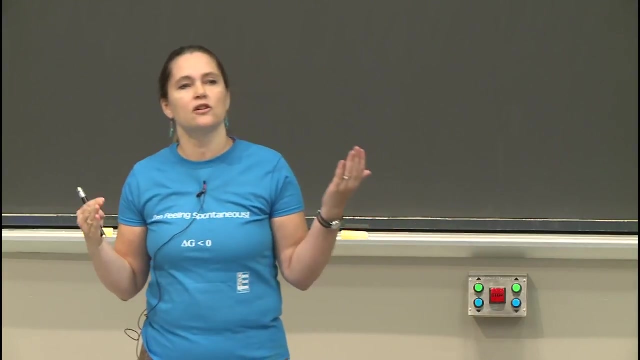 in their molecular or atomic weight. OK, so we have two significant figures. Also, our current and time only had two significant figures. so we only have two significant figures in this problem. All right, so in this particular electrochemical cell again. 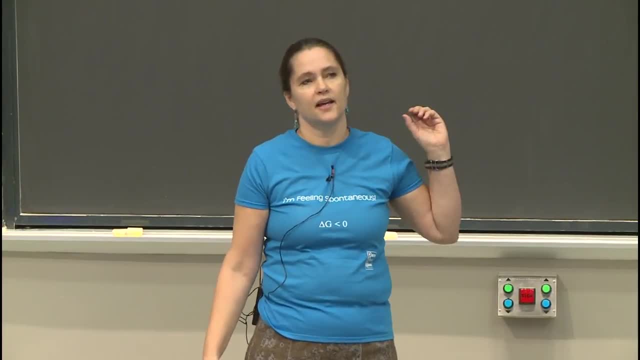 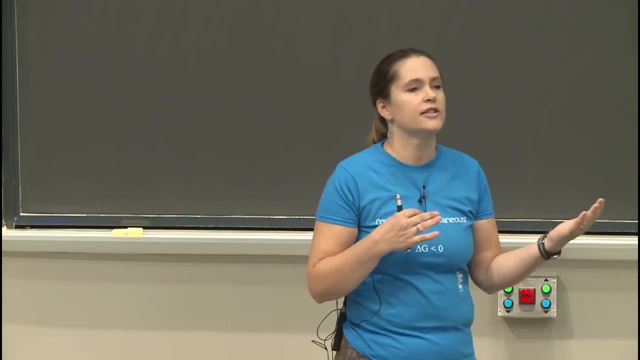 we had, our anode was being consumed and the electrons that were generated ended up plating the copper on. Sometimes you're not going to want to do that. Sometimes you're just going to want to actually plate something with copper, for example. 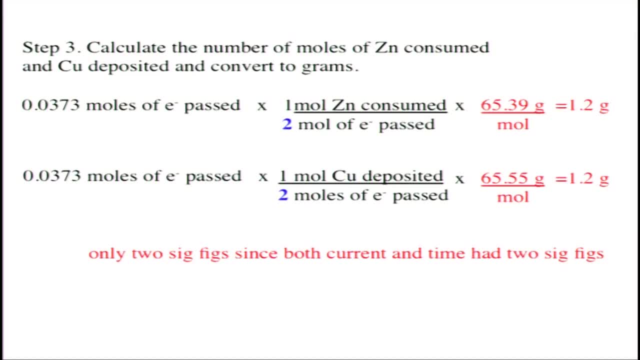 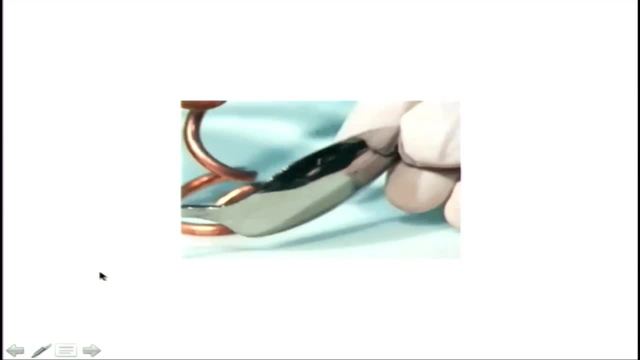 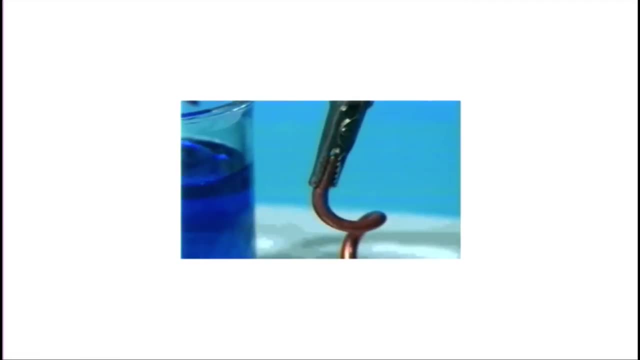 And so let's look at some of the uses for this kind of chemistry. So here's some electroplating. This steel spoon will have a thin coating of copper deposited on it. The cell consists of an anode of pure copper, a solution of copper sulfate. 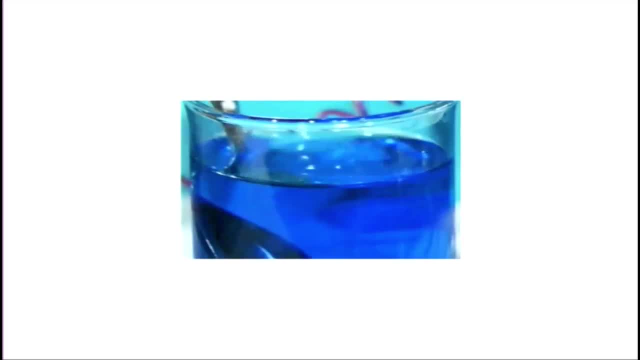 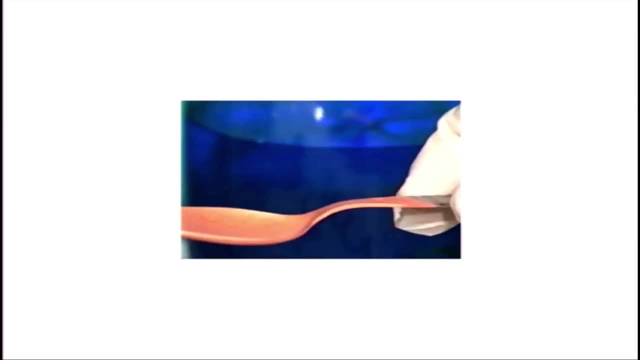 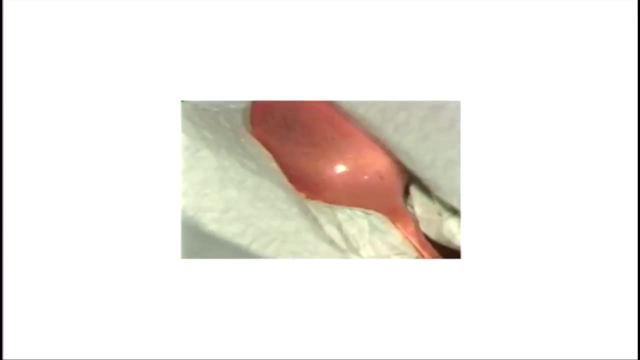 and, as a cathode, a spoon. There is no net reaction, but copper metal is transferred from the anode to the cathode. That's pretty nice, OK, so this kind of electroplating is pretty common where you use these kind of reactions. 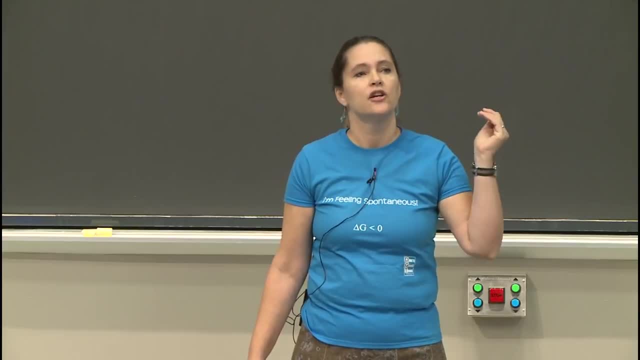 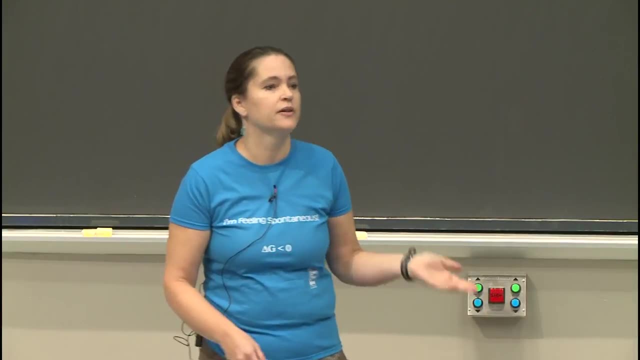 to get your copper, which is in that solution, to plate as copper solid onto something. So it could be a spoon, it could be electrode. Yeah, Why is it dangerous? Why is it dangerous? You know, I've seen these demos before. 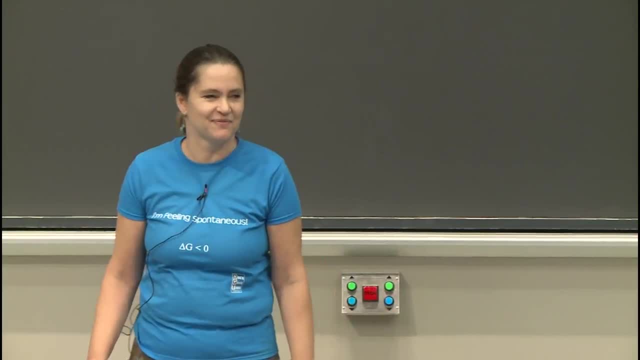 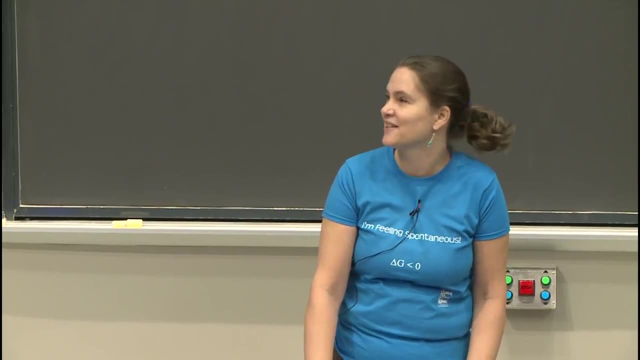 so I'm not, I'm not, I think that they that's just like security regions to say, to say that I don't think it's like incredibly dangerous, frankly, but I probably shouldn't say that I'll get myself into all sorts of trouble. 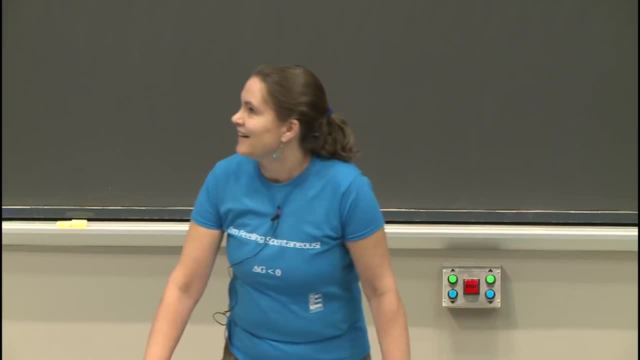 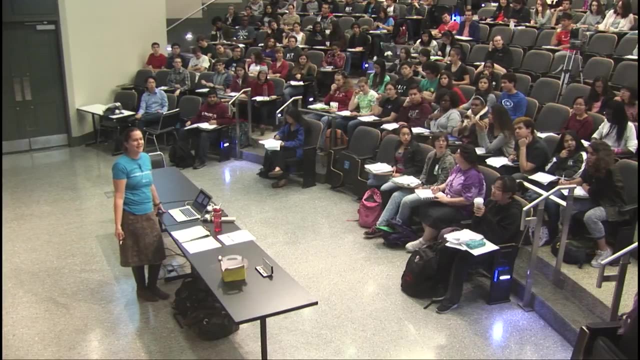 Don't try this at home, I don't know why. All right, Usually, when you're doing the plate, the chemicals that you use are Yeah, but not like, not that much worse than a lab solution. Yeah, Elena makes jewelry. 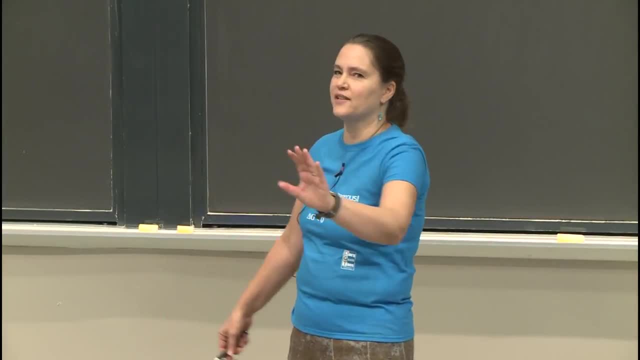 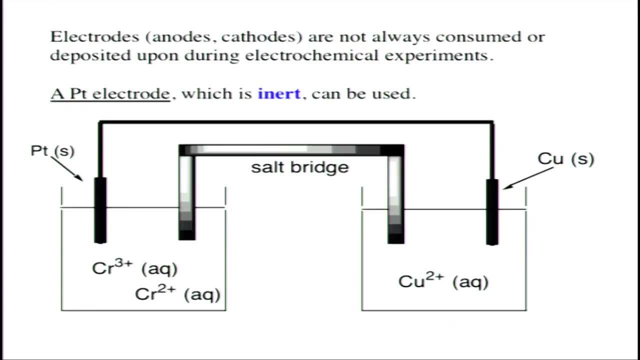 so she knows all about this, But she doesn't, she doesn't. she does it very safely, very safely, Okay, All right. So let's look at a couple other kinds of electrodes. It is not always the case that electrode is consumed. 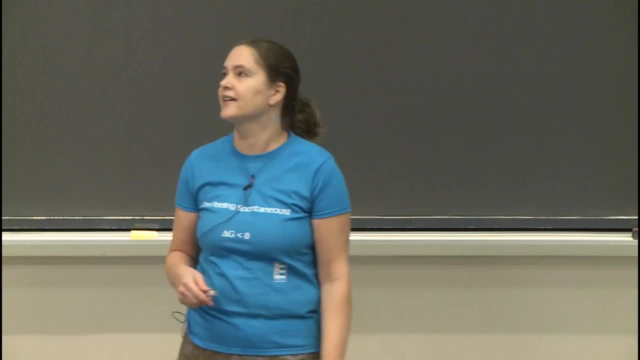 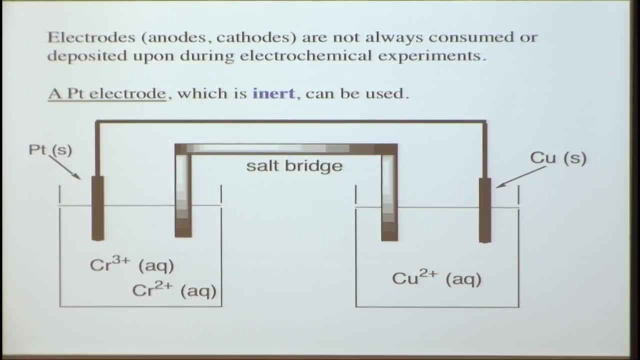 or that an electrode gets stuff deposited on it. Some electrodes are inert. An example for this is a platinum electrode. It is inert, so it doesn't get consumed and it doesn't get reacted onto during the reaction. And so here's an example of a cell that uses this. 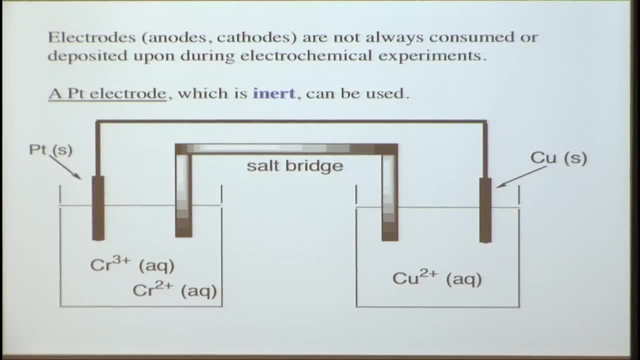 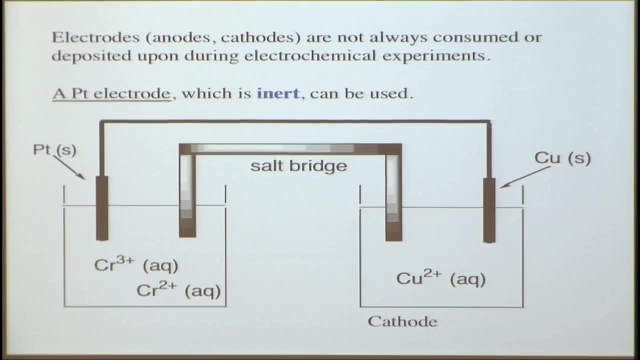 So over here now we have still our copper system. So this is our cathode again over here, And a cathode does what? Oxidation, or reduction, Reduction, Reduction. And so this is our same reaction: copper plus two. 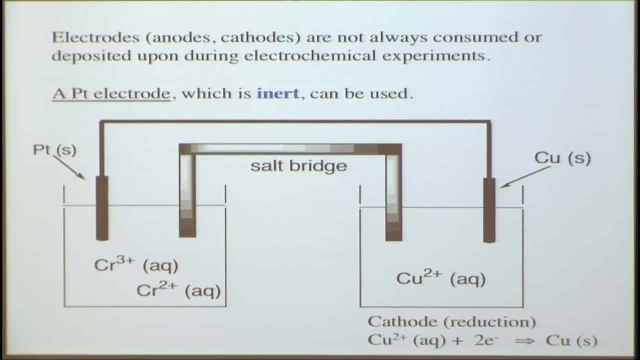 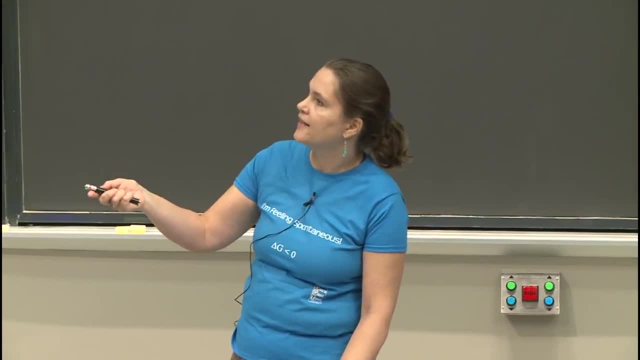 two electrodes coated copper solid. So this is doing the plating again, But in this time it's different. Before we had the zinc electrode that was being consumed, but now we have this platinum and the reaction that happens at the anode. 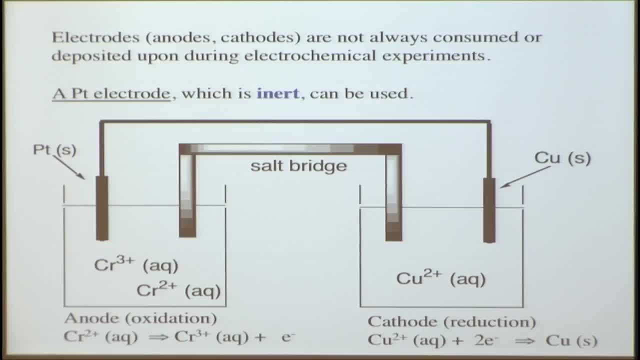 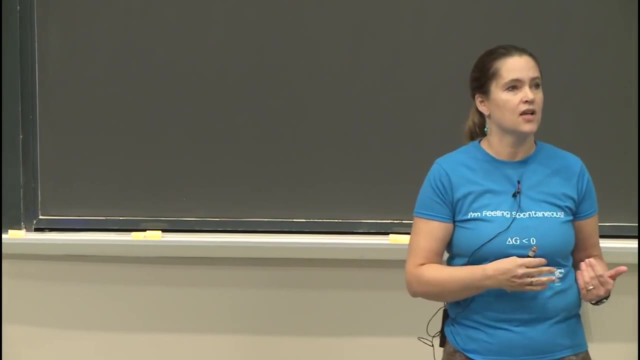 it's still an oxidation, always an oxidation at the anode, but the oxidation reaction is chromium plus two going to chromium plus three in an electron. So here the electrode is inert and the reaction is all happening in the same phase, all happening in solution. 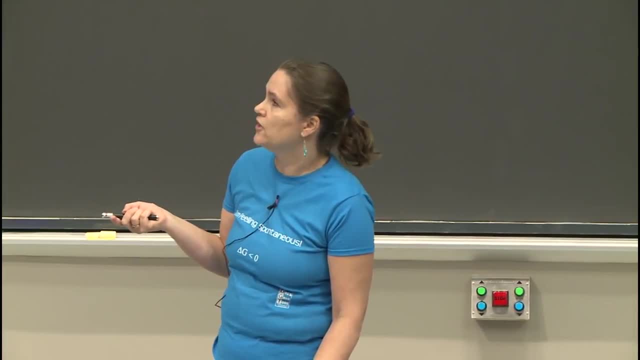 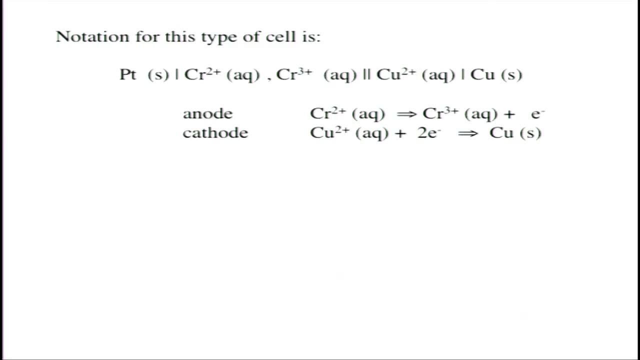 So we can also write the notation for this kind of cell. And so here we would have platinum solid, the single line, which means the phase difference: chromium plus two aqueous comma, because now there's not a phase transition between these, chromium plus three aqueous. 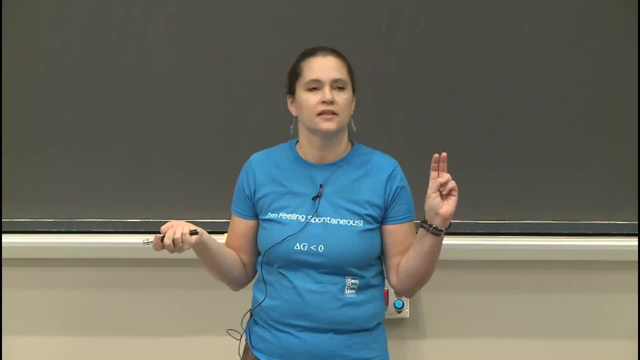 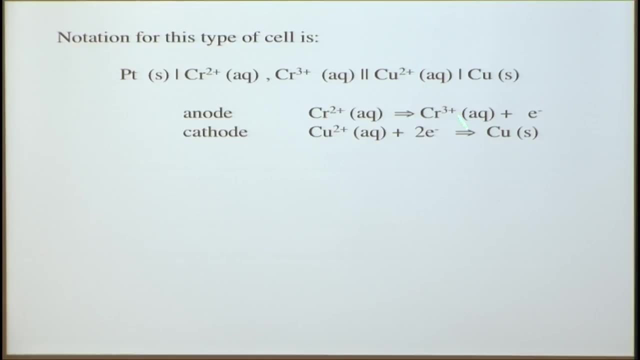 the two lines. that means what? What do those mean? again, Salt bridge, Salt bridge. So this indicates, that's one beaker, this is the other beaker, And here we have the copper plus two aqueous single line for phase change and copper solid. 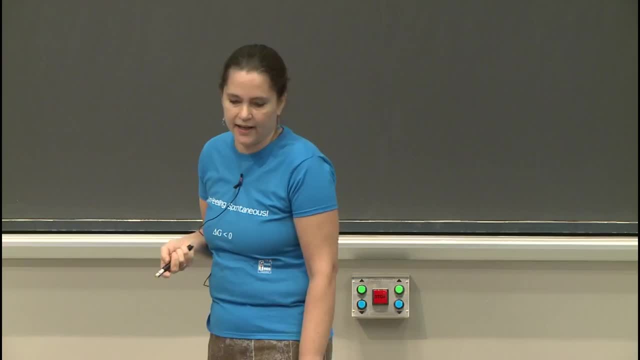 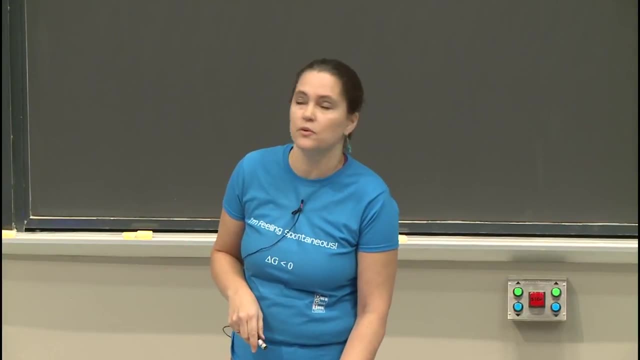 So again, our anode reaction and our cathode reaction. All right, So this is another kind. You can also use platinum electrodes in combination with what's known as a hydrogen electrode, So these are often together, the platinum with the hydrogen. 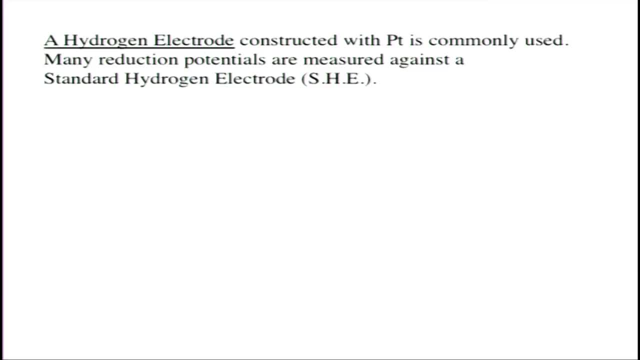 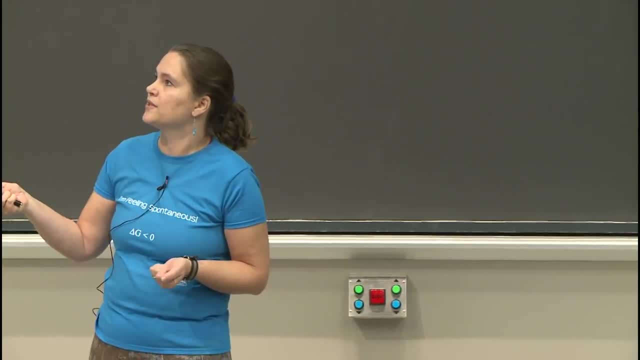 And many reduction potentials and when you get problems at eight you're going to be looking up in your book a lot of standard reduction potentials and many of them will say measured against SHE. And a lot of times a lot of people say like: 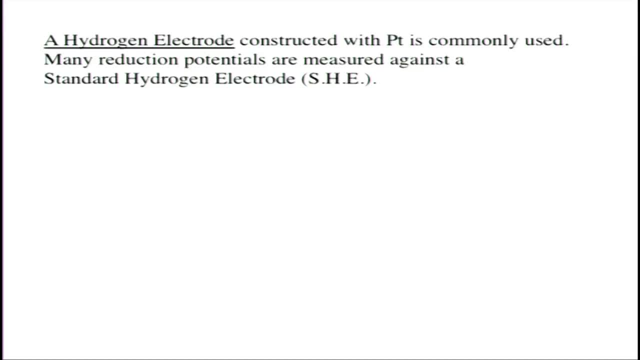 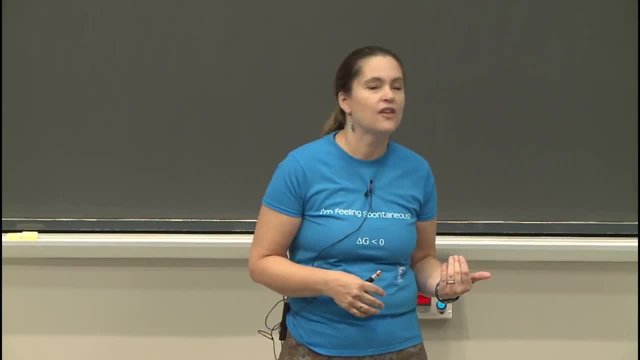 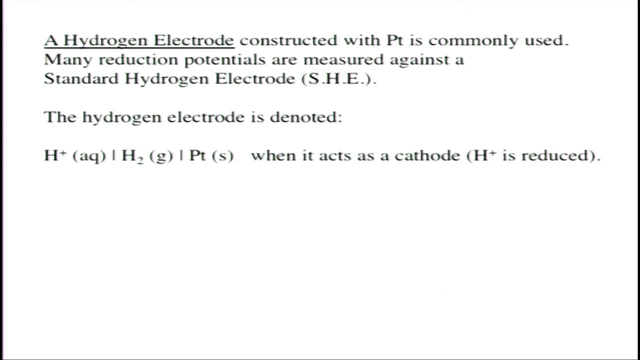 who is this SHE that measures all of these potentials in the back of books And that SHE is the standard hydrogen electrode? All right, So let's think about how this electrode is being used. So when it's used as a cathode, we have H plus aqueous phase transition to H2 gas. 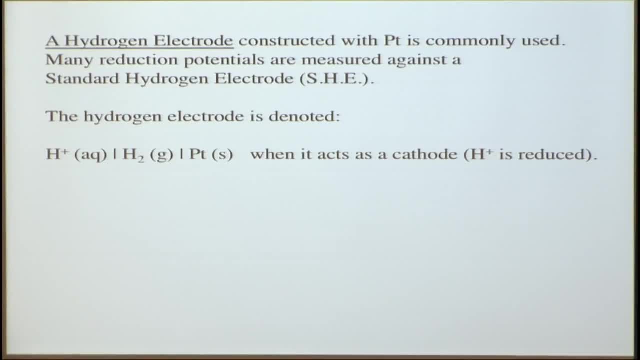 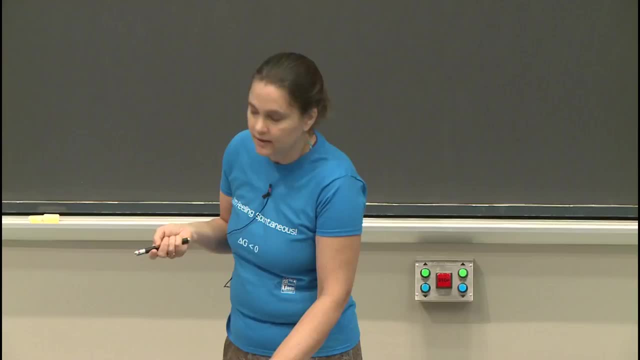 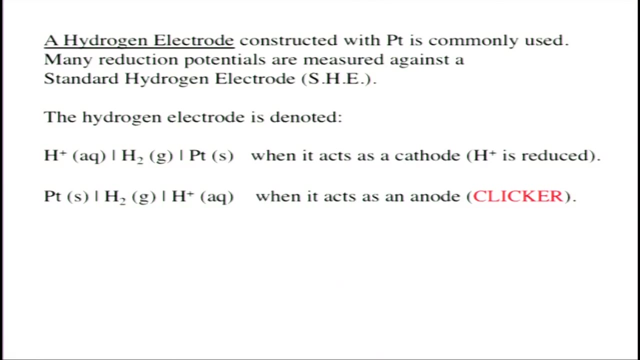 and then another phase transition to our solid platinum inert electrode. And here, when it's used as a cathode, H plus is being reduced, but it can also be used as an anode, And this is a clicker question. Why don't you tell me what would be happening? 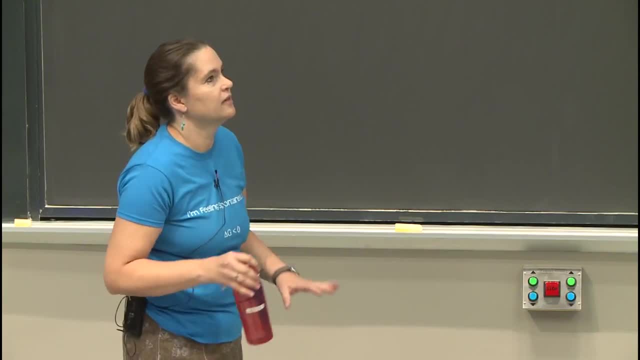 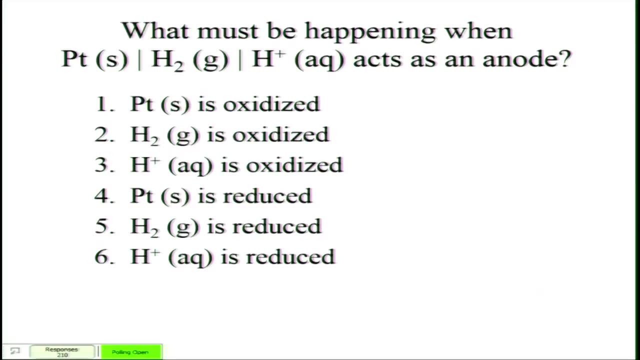 when the hydrogen platinum electrode is being used as an anode or reaction is being used as an anode. 10 seconds, Let's see if we can get 90%, 89%, 89%, Oh, Far away. OK, That is the right answer though. 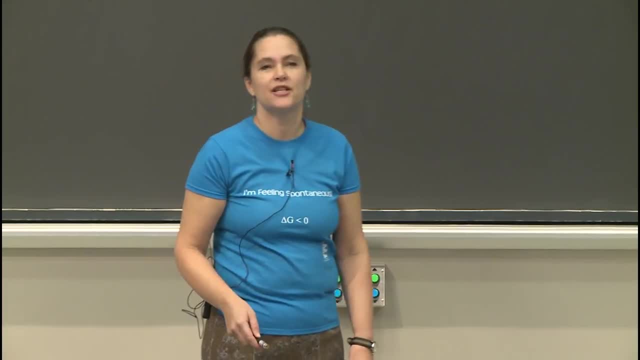 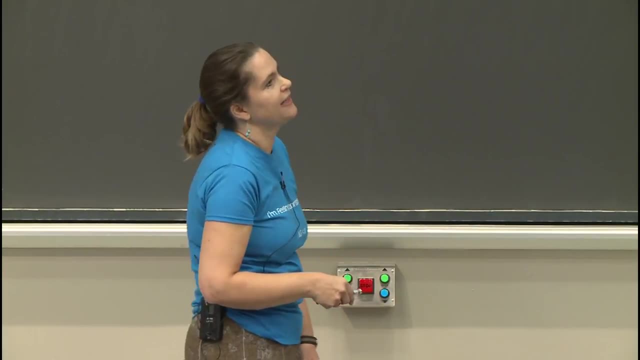 OK, So some of these: the platinum is inert so it's not doing anything, And it's over here, so it's not doing anything. So we can rule out all the things that platinum are doing stuff. All right, H plus being oxidized. 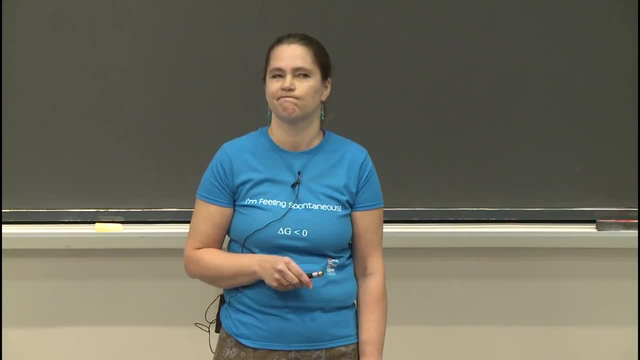 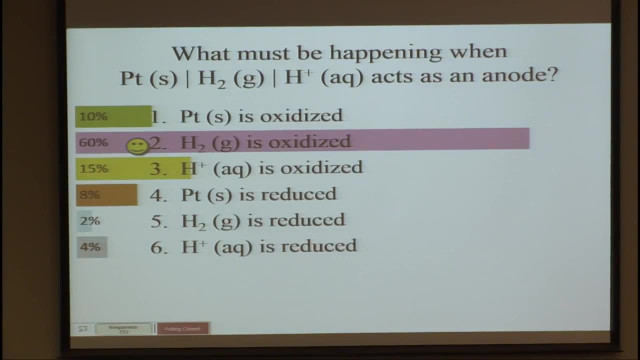 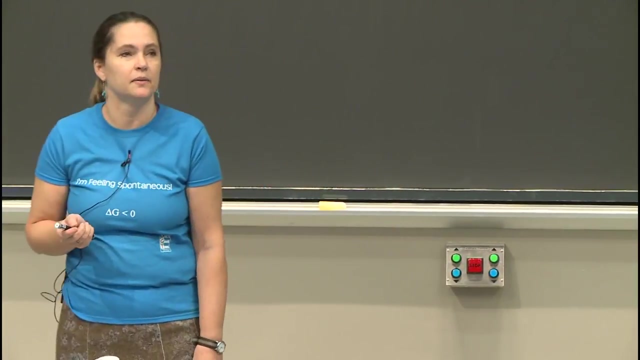 You ever heard of H2 plus? No, So we don't want that. We know at the anode it should be oxidized so we can eliminate all the ones that are reduced. OK, So we have really kind of one good option if you say that the platinum is inert. 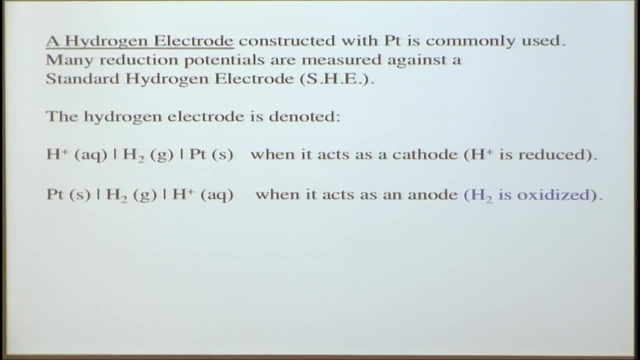 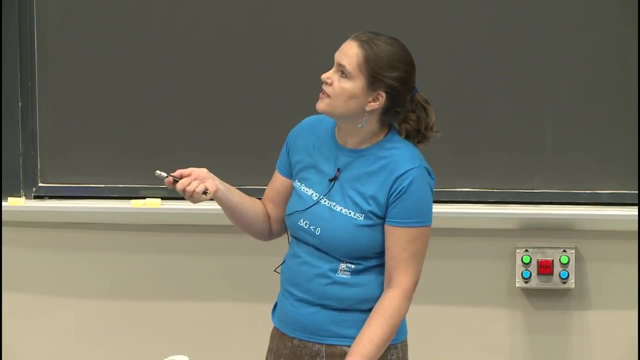 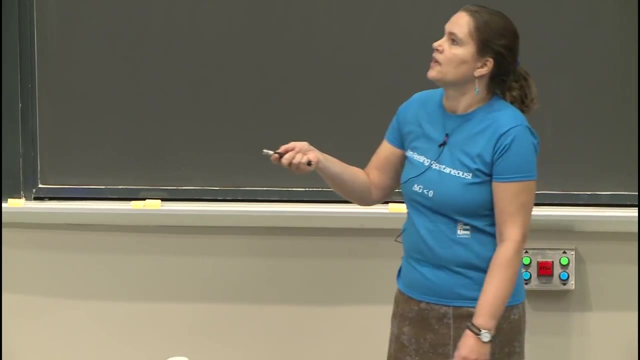 So H2 then gets oxidized, in this case forming H plus. All right, So let's look at a cell like this that uses the hydrogen electrode. So here's an example. Now on this side we have our regular zinc system. 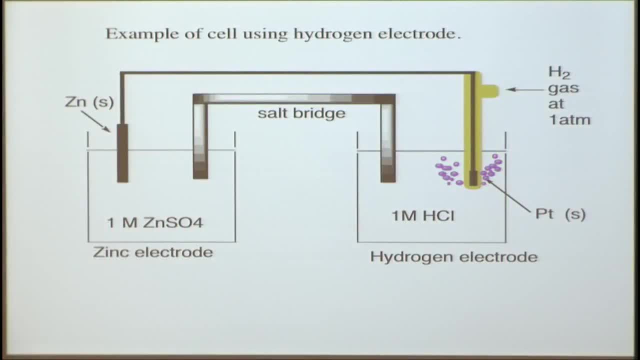 for our anode, And so over here we're using as the cathode the hydrogen electrode. And so here, in this beautiful drawing that I made, we have a glass tube here where you're pumping H2 gas in at one atmosphere. In the middle of the tube we have our inert platinum. 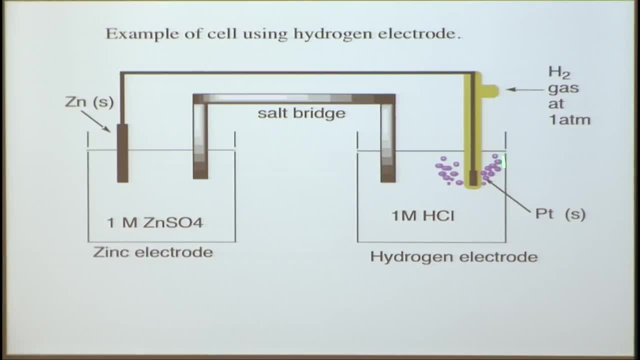 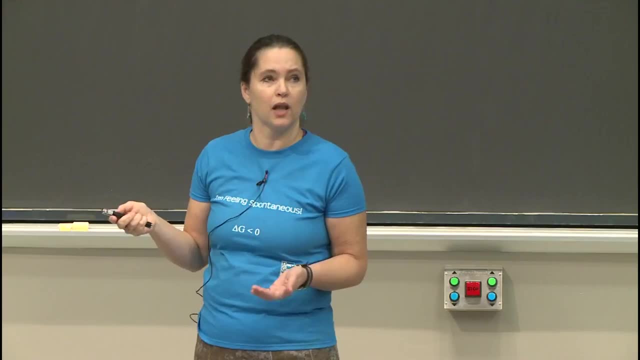 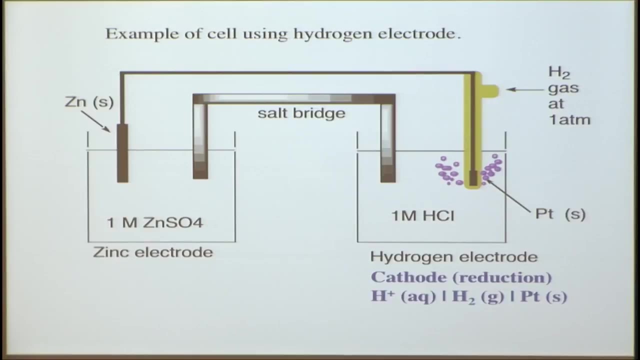 electrode And then these are H2 gas bubbles down here And we have strong acid, HCl, which is our source of H plus in solution. So over here again, this is our cathode, So we have a reduction at the cathode. 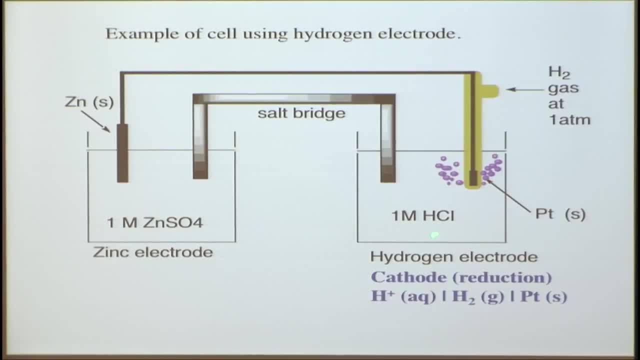 And we have H plus aqueous phase transition, H2 and gas, and then another phase transition to our solid platinum electrode, And over here is our standard anode, our oxidation that involves zinc and zinc plus 2. So we could also have had the hydrogen electrode.